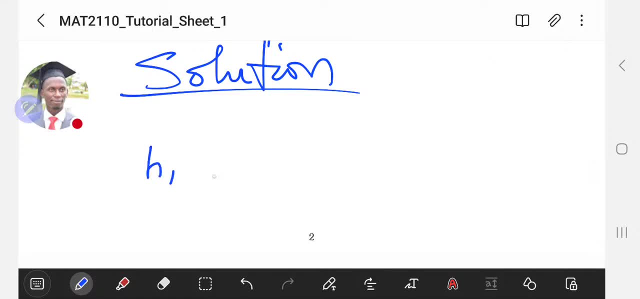 what you need for the, for the most part, is if the center is always given at h comma k. if this is where the center is, then you know to say: the standard formula of a circle is going to be for the x, you're going to have x. 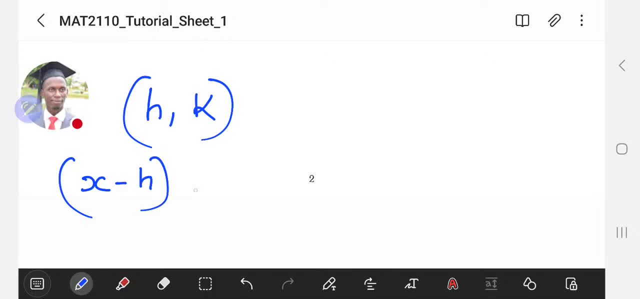 minus where the center is. so the x coordinate, that is, of the center squared plus. then you have y minus the value of k. then this squared equals to one, uh equals, not not one, the radius squared. so this is an expression that gives you the standard formula of a. 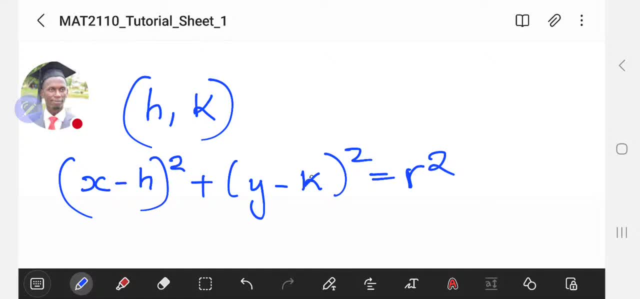 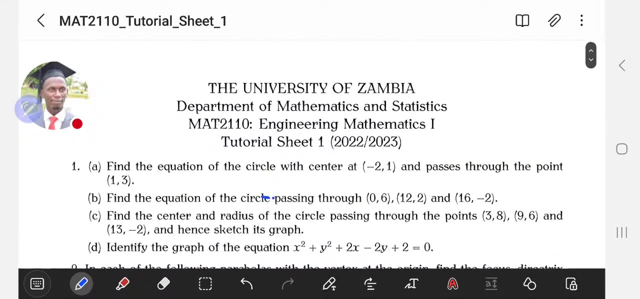 circle, but in this case we're being told where the where the center is. now, how do we actually get the equation given? uh, where the center is, and and where the. uh, yeah, and the point where this, this circle actually passes, if you get the coordinates that have been given. we have two coordinates for the center. 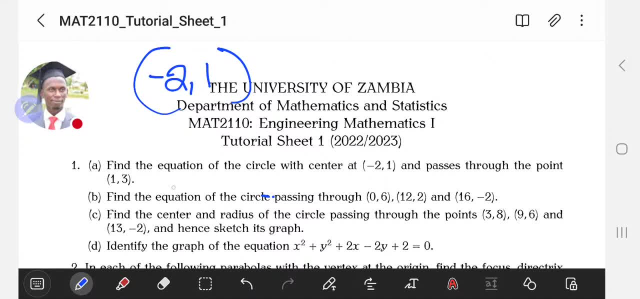 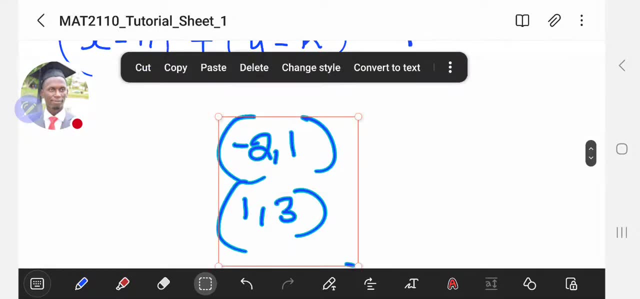 we have negative two comma one. this is our center, and then it passes through a point one comma three. so if you have these two points, let's get them. let's see, um, let's take them down. okay, so we know, our center is at negative two comma three. what does that imply? it now means that. 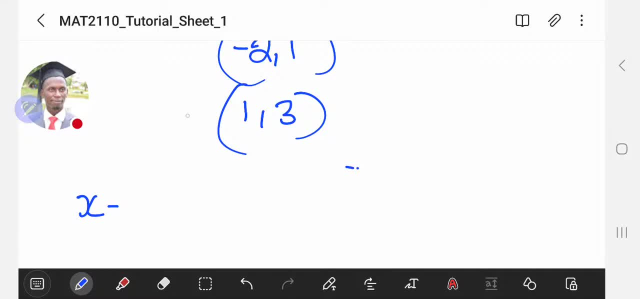 we can have our equation as x minus negative two. so you have negative two here and then this is squared. then you have plus the y value, so you have y minus the y value from the center, which is just a one squared equals to the radius squared, so this of course becomes x plus two. 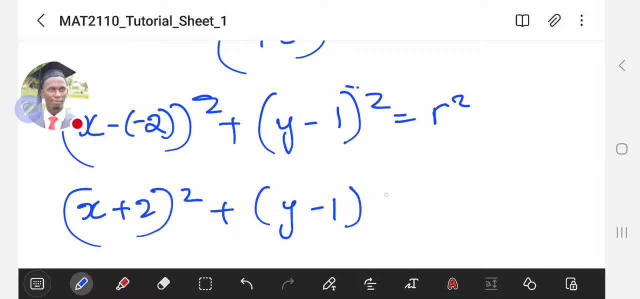 squared plus y, minus one squared, equals to r. for this to be complete, we see that we need to know what the radius is. but how do we get what the radius is? to understand what the radius is, we have to go back and see how the radius relates. 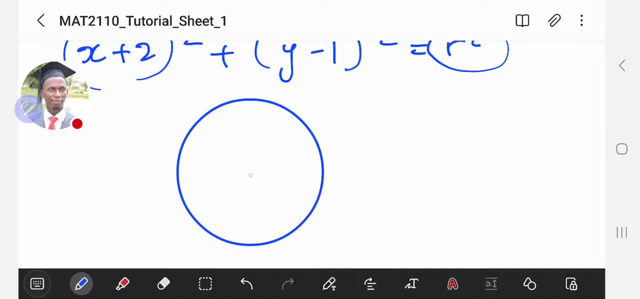 to um, to the circle itself altogether. if the center is here, then what you have to understand is that the distance from the center to any point on the circumference, that distance is actually what the radius is going to be. so if the center is at h comma k and this point is at x comma y, 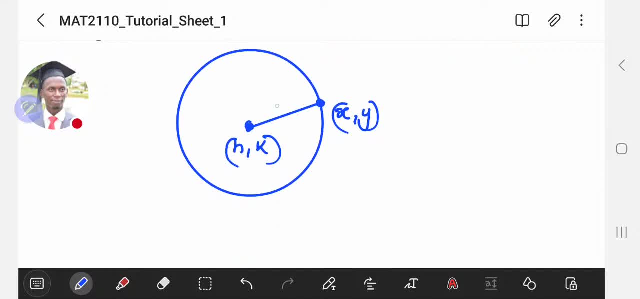 notice that it then implies that to get the distance here, which is of course the radius, the distance squared will be equal to you know how to get the distance between two points. it's going to be: you're going to have the first part, so you can say um. 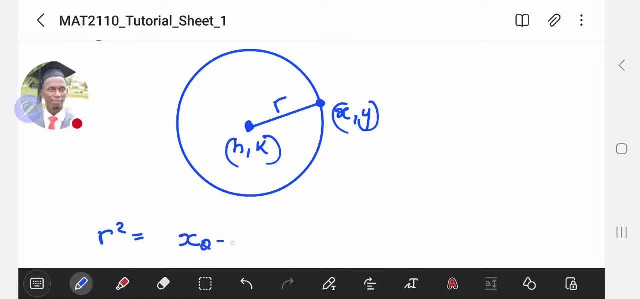 x. let's even say x2 minus x1 squared, plus y2 minus y 1 squared. this is how we get the distance between two points. so in other words, the radius will now be equal to the square root of x2. we can use x2 as the value this side. this is where x2 will be. 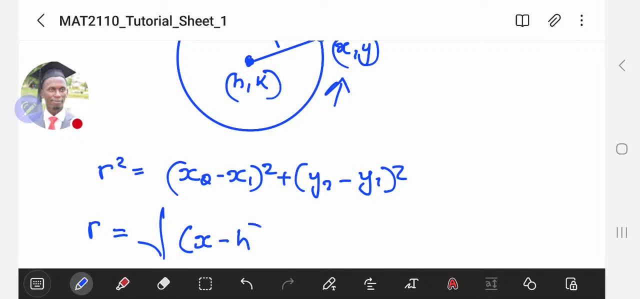 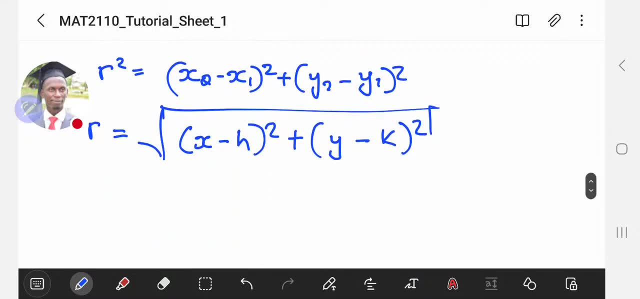 so we're going to have x minus the value of h squared plus. then this is going to be y minus the value of k squared. so this is a technique that we're going to use here, so we substitute this, the point we're using in this case for our question, this circle. 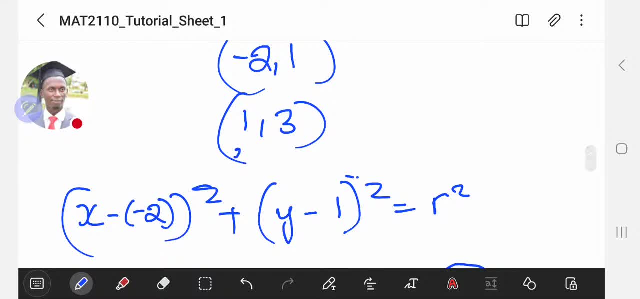 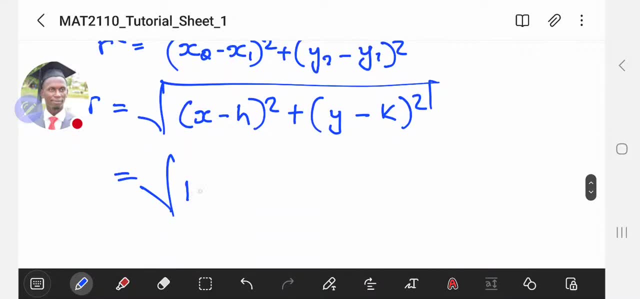 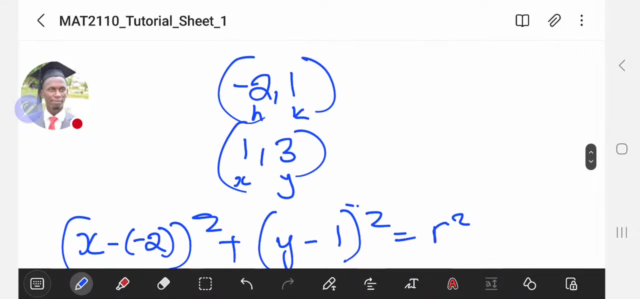 passes through a point one, comma three. so this will be our x, this is our y, and this is to our h, this is to our k. so we have that's one minus minus, uh minus two, so it becomes one plus two. uh, squared then, what else plus the y value? the y value from our point, that's. 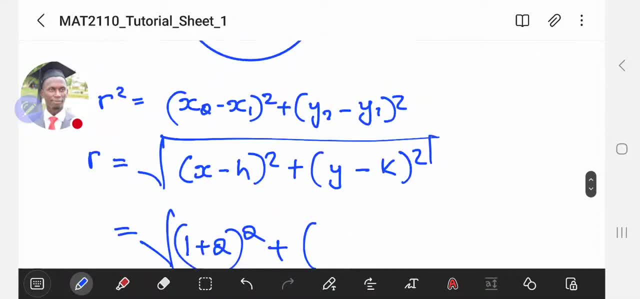 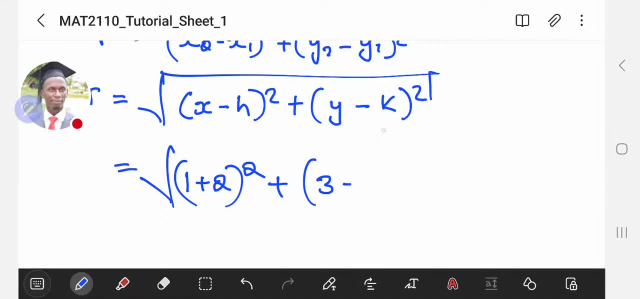 one, that's a one. um, the y value- sorry, that's a three. the y value, that's a three. so i'm going to have three here, minus, uh, the value of k. the value of k is coming from the center and the center was at negative two. 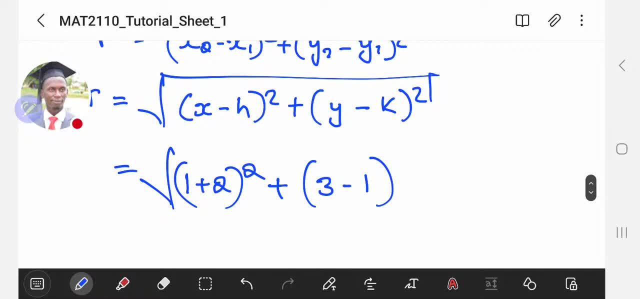 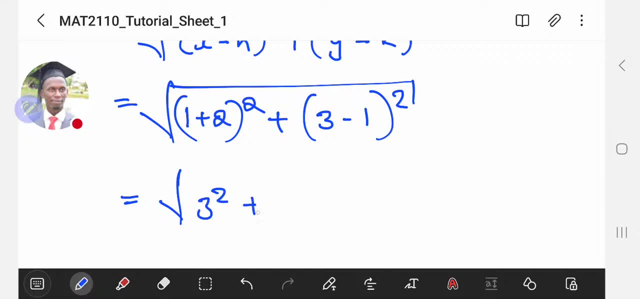 comma one. so that's a one, so i'm going to have a one here. then this has to be squared, so we simplify this. this becomes three squared, this becomes plus two squared, and then this is going to be nine plus four, then this is going to be root 13.. so r becomes 13, of course. 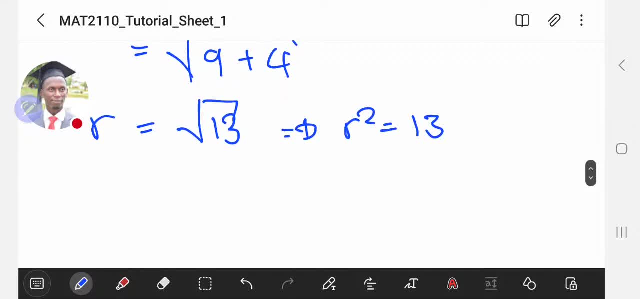 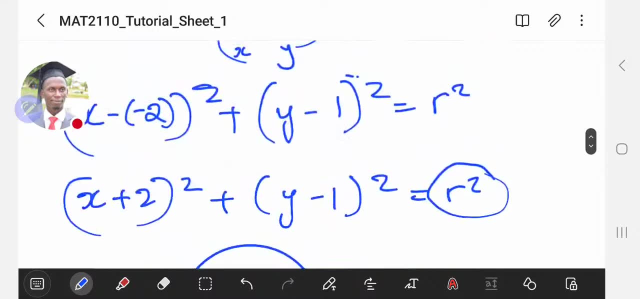 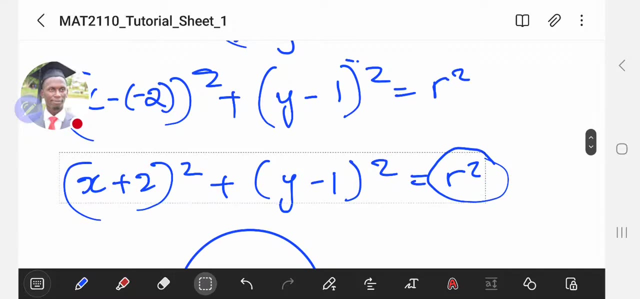 here, r squared is equals to 13.. so, uh, yeah, r squared will be 13.. so if we go back to the standard formula- we already wrote it earlier on the standard formula, when we substituted the values for the center, we had this expression: let's not get this. let's get this one here. 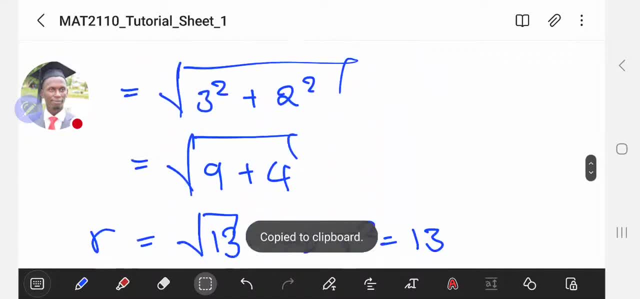 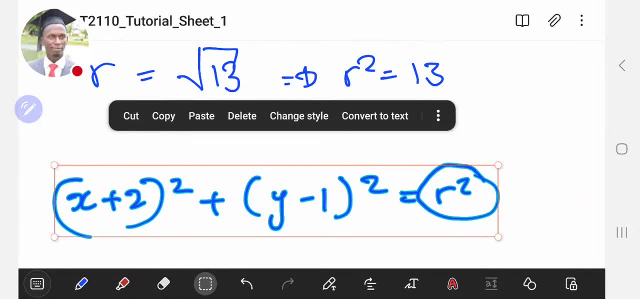 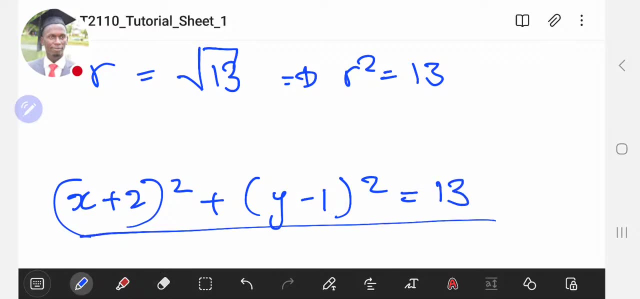 so we had this expression, so let's bring it down. so if we bring this expression down, now we know what the radius is. so where there's r squared here, we'll just put that 13, so this becomes the standard formula of standard equation for this circle that passes. 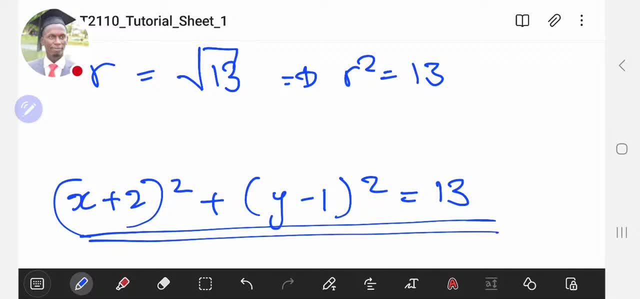 through negative 2 comma 1, that has a center negative 2 comma 1 and whose center is at, uh, whose center is at negative 2 comma 1 and passes through that point which was given us. um, what point was that? again, that was 1.3. 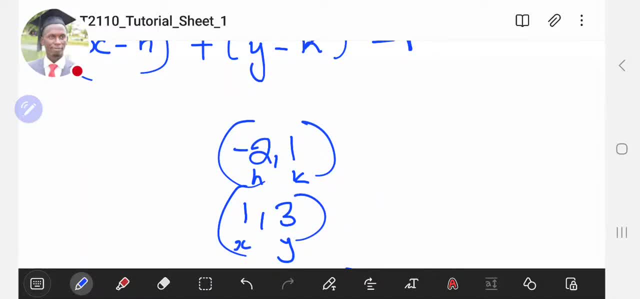 okay, so now we're going to have this equation, so this is how we're supposed to work out this question. yeah, so i'll be checking out in the charts, in case you are with us and then you have a question there, ask to be able to to check there. so that, um, yeah, see, 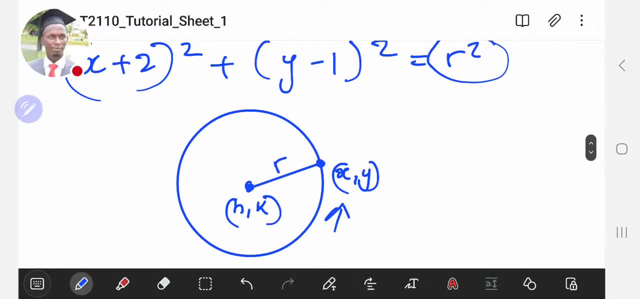 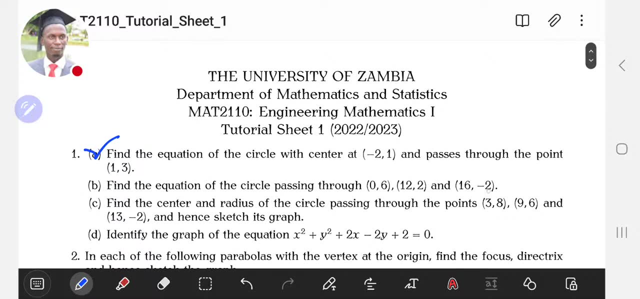 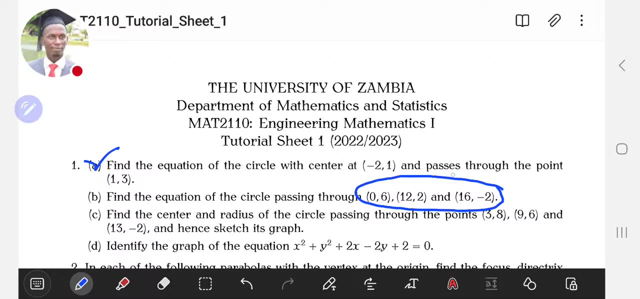 the questions that you guys are having here. okay, so this is how you handle the first question, so that deals. that sorts out this one. uh, the second question here now notice that we're given three points, but instead of um, we're not given what the center is. we're given three points, so we've seen that. if 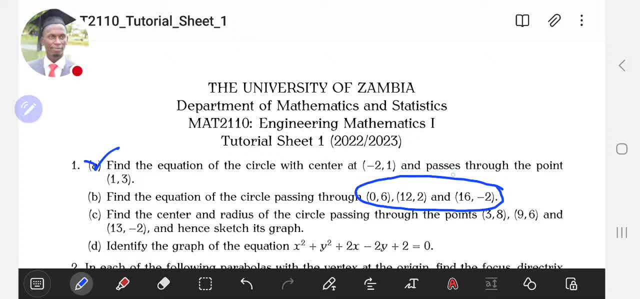 we know what the center is, we're given three points. so we've seen that if we know one point on the circumference of this circle and we know the center, it's easy for us to get the equation. but what if you're given three points instead? well, there are a number of methods that 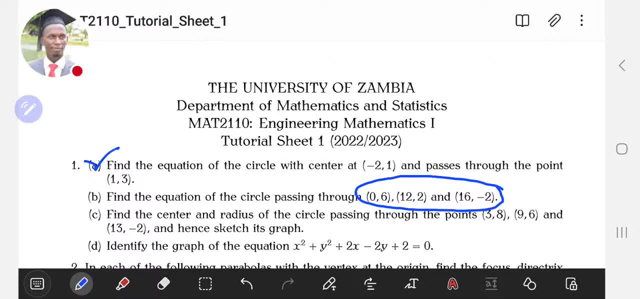 you can use here the method that i'm going to show you here. i feel it's a little bit easier. in the other method you will have to solve a simultaneous equation in three unknowns, but in the method i'm going to share, you just have to take advantage of one simple trick. 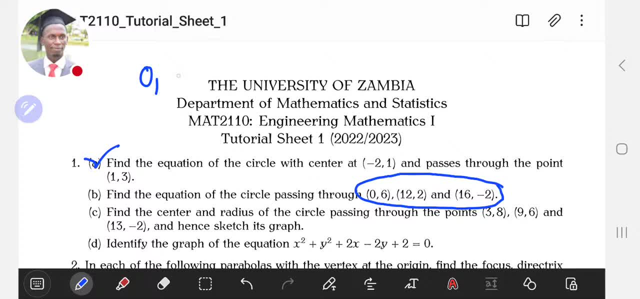 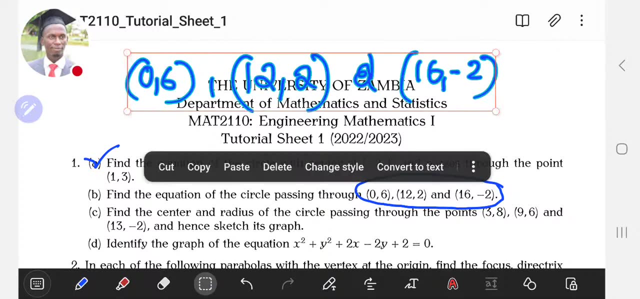 so let's just take the points down. so the points here are 0.6 as a first point, then you have 12.2, then you have 16 comma negative 2.. so these are the points that, uh, that you have here. now, how do we take advantage of, or how does the, the method i want to show you, work well for this? 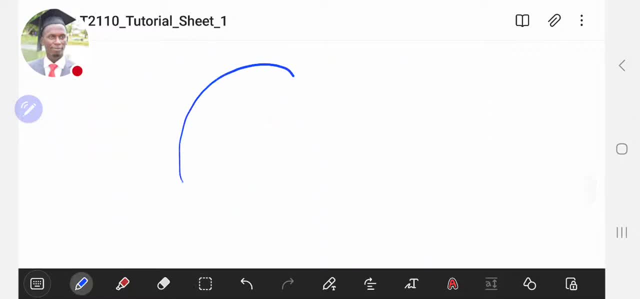 method. here is how it goes. you want to take advantage of one thing: if you have three points on this circle, let me start with two. so if you picked two points on the circumference- this point and this point- and then you connected them, so if you connected these two points here, 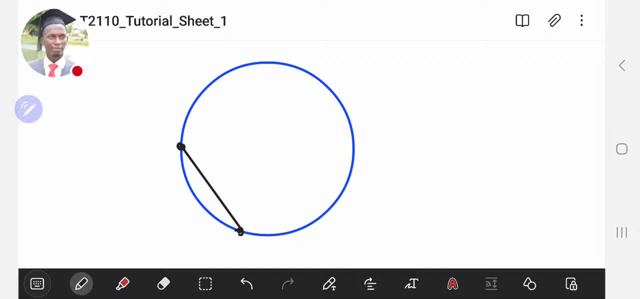 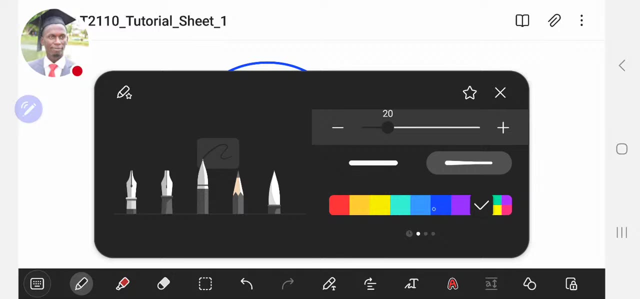 and then you, you find the center of these two points. let's say, the center happens to be somewhere here, and then you draw a perpendicular at this exact point. so if you draw a perpendicular line at that exact point and then you have its equation, then you get your third point, remember? 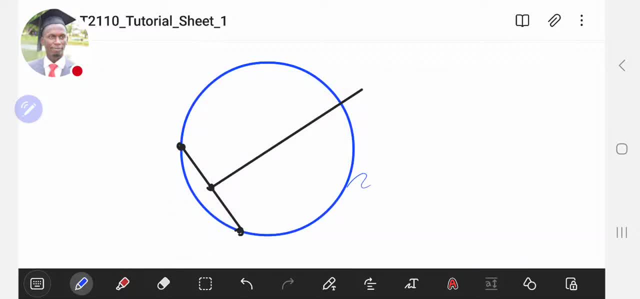 in the question you're given three points. so if you get a third point, let's say, the third point is somewhere here. so now, if you connected this point, n of these points, really even if even the other point could have worked, if you connected these two points, then find the center, the midpoint of this new line and then also draw a perpendicular. 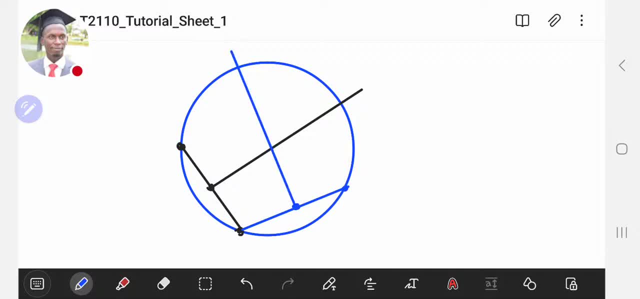 from this line. what you have to understand is that at the point where these two lines meet, where this is the first line and this is the second line, perhaps let me have them in red- at the point where these two lines meet, that is exactly where the center is. 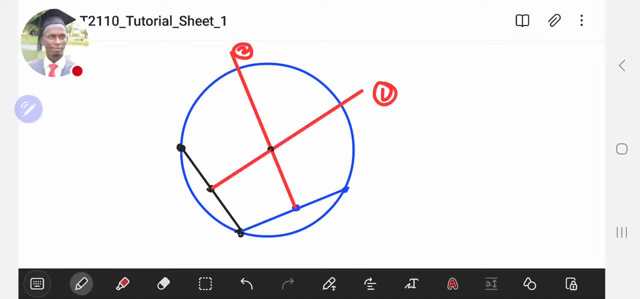 so we see that our center in this case is going to lie right here. so in this method, all we have to do is come up with the equation for this red line, then come up with the equation for this red line number two. once you have the two equations, equate them where they are equal. 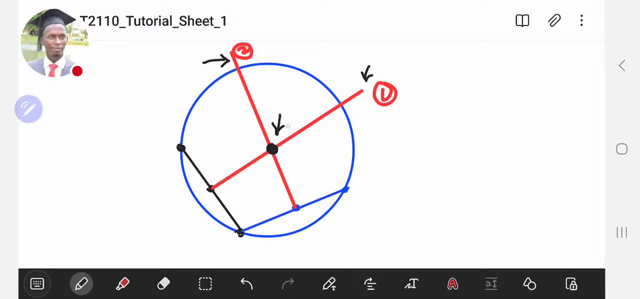 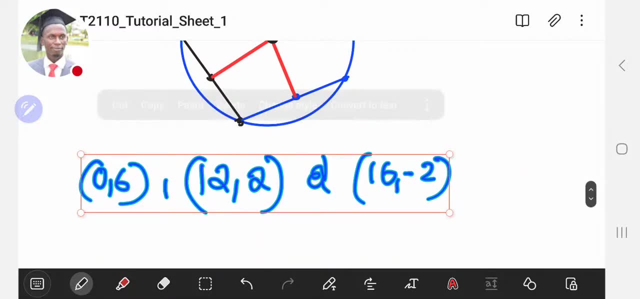 that is going to be where the center is. now. what do i mean? let's get three points that we had. so our three points in this case were these points. so i'm going to start with the first two points, these points, and i'm going to say: 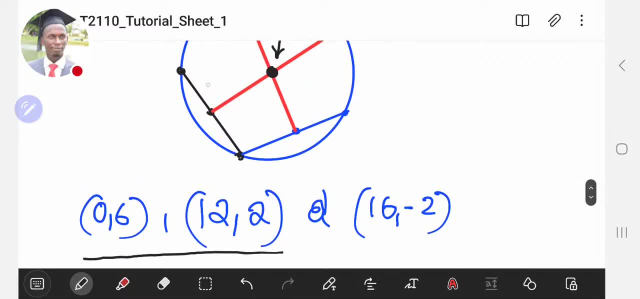 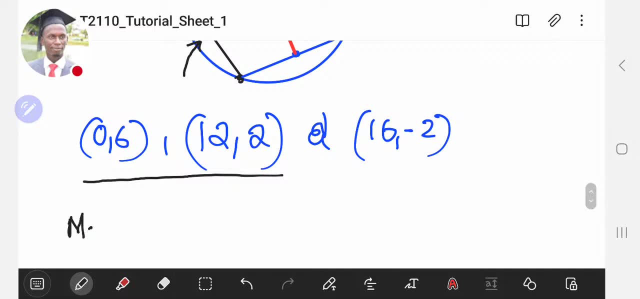 these are the first two, two coordinates that i want to deal with. so what i'll do is: first i want to find their midpoint, so i'll find the midpoint of those two points. so to find the midpoint of any two points, you know how it goes. you get the x coordinates, add them, then half them, so this is. 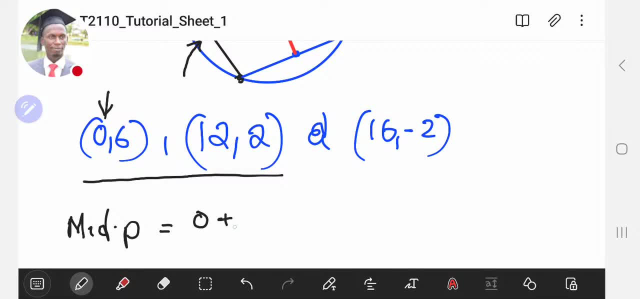 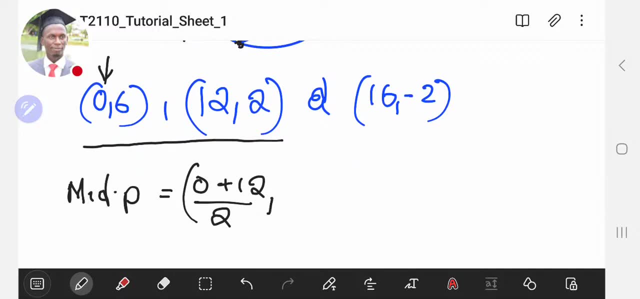 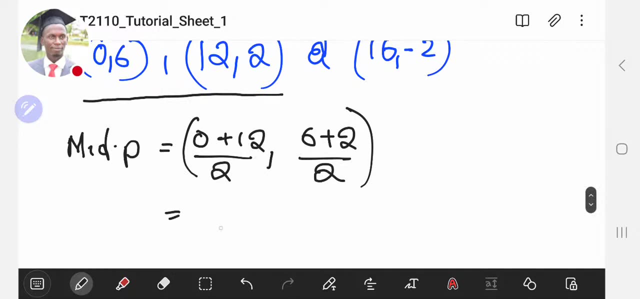 going to be 0 from the first point plus 12 from the second point. then divided by 2, this will give me the first coordinate, the x coordinate comma, now the y values. so that is going to be 6 plus 2, then divided by 2 as well. so this now gives me from the first part i have 12 over 2 comma. this. 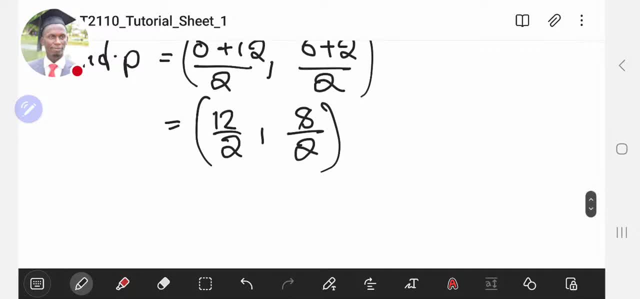 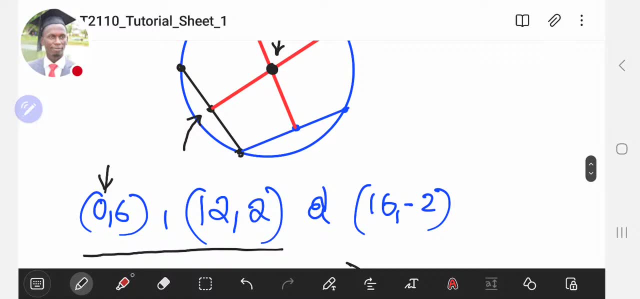 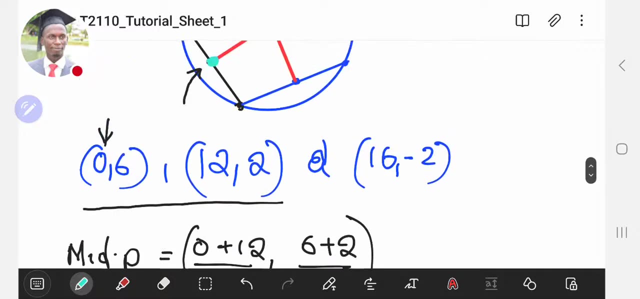 is going to be 8 over 2, so that this now becomes 6 comma 4. so this becomes the midpoint. now i know that this point is actually according to what we've done, this is 6 comma, that's 6 comma. what? 6 comma 4. now we know the midpoint to get this equation, to get the equation of this red line. 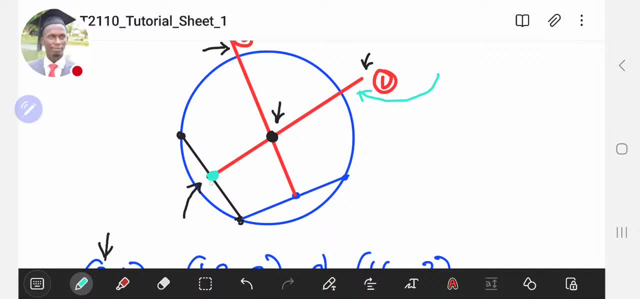 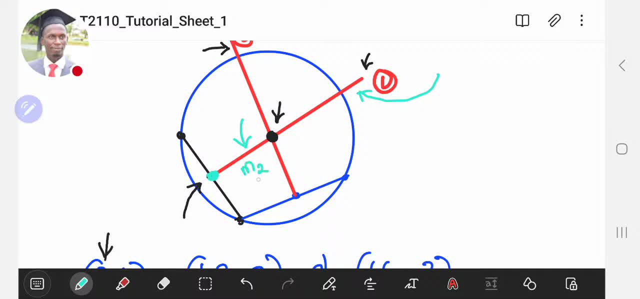 red line to get the gradient of this red line. but to find the red line. to get the gradient of this red line. but to find the gradient if i labeled its gradient here gradient. if i labeled its gradient here gradient. if i labeled its gradient here as m2, to find the gradient of m2 here. as m2 to find the gradient of m2. here as m2 to find the gradient of m2. here we first are going to find the gradient of. we first are going to find the gradient of. we first are going to find the gradient of the first line. 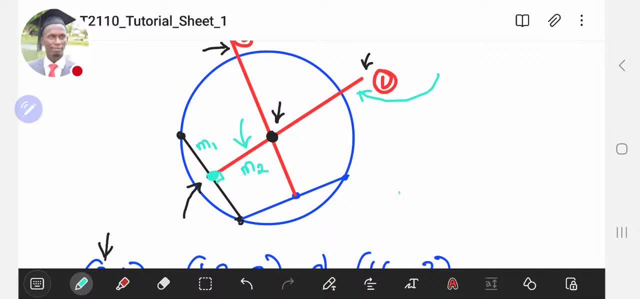 the first line, the first line: m1 here. since the two lines are m1 here, since the two lines are m1 here, since the two lines are perpendicular, you know to say the perpendicular, you know to say the perpendicular, you know to say the gradient of m1. 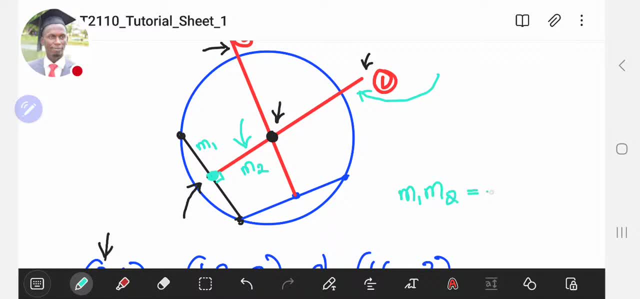 gradient of m1. gradient of m1 multiplied. the gradient of m2 is just multiplied. the gradient of m2 is just multiplied. the gradient of m2 is just going to be equal to going to be equal to going to be equal to negative one. so this is how the two 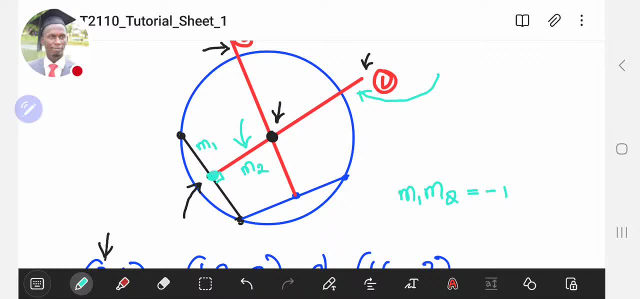 negative one. so this is how the two negative one. so this is how the two gradients will relate. gradients will relate. gradients will relate when the two lines are perpendicular, when the two lines are perpendicular. when the two lines are perpendicular, which is going to be the case here, 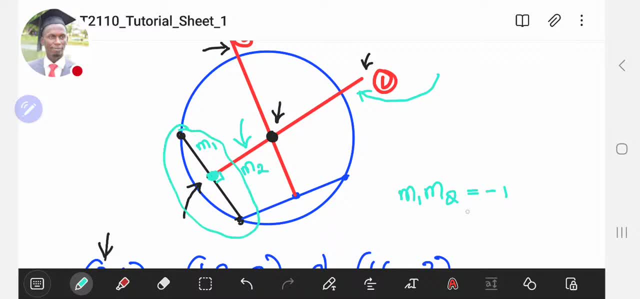 which is going to be the case here, which is going to be the case here. so let's find the gradient of this line. so let's find the gradient of this line. so let's find the gradient of this line first, so that we use this expression to. 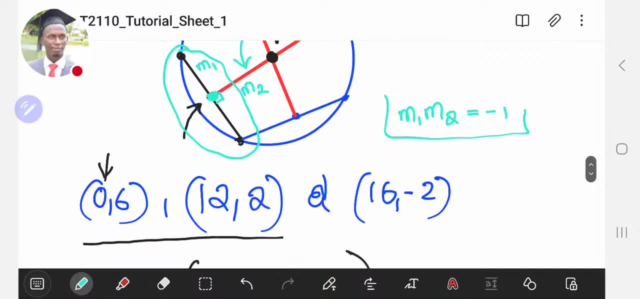 first, so that we use this expression to first, so that we use this expression to determine what the gradient m2 is going, determine what the gradient m2 is going, determine what the gradient m2 is going to be, to be to be. so how do we do that? 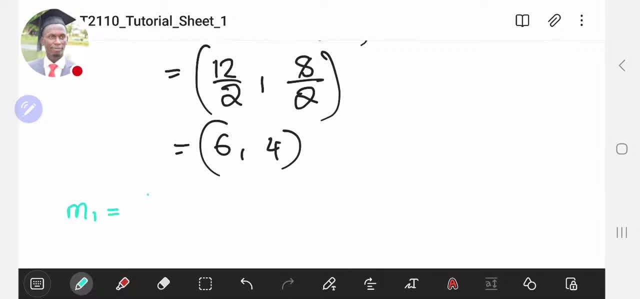 so how do we do that? so how do we do that? to find the gradient m1. we're going to, to find the gradient m1. we're going to, to find the gradient m1. we're going to say m1 will be equal to y2. 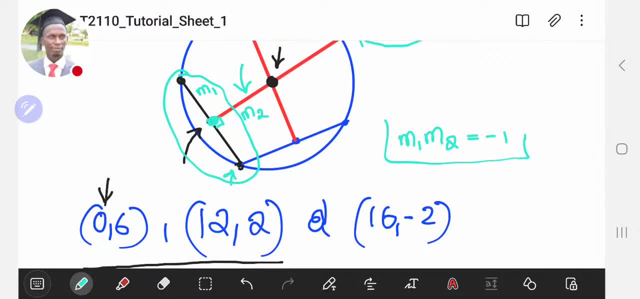 say m1 will be equal to y2. say m1 will be equal to y2, y2. in this case, y2 is going to be at y2. in this case, y2 is going to be at y2. in this case, y2 is going to be at this point. doesn't really matter where it. 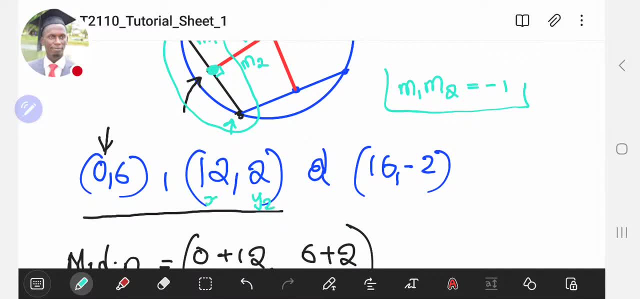 this point doesn't really matter where it. this point doesn't really matter where it is, so i'm going to take this as my y2 is. so i'm going to take this as my y2 is, so i'm going to take this as my y2 for this part. this is my x as my x2. for this part. this is my x as my x2 for this part. this is my x as my x2. then this is my y1 and this is going to then. this is my y1 and this is going to then. this is my y1 and this is going to be my. 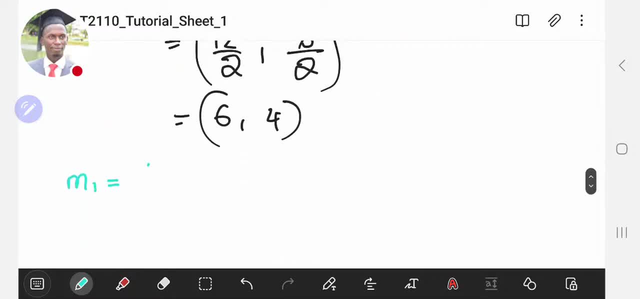 be my, be my x1. so i'm going to have 2 minus 6 x1. so i'm going to have 2 minus 6 x1. so i'm going to have 2 minus 6. so it's going to be 2 minus 6 divided by. so it's going to be 2 minus 6 divided by: so it's going to be 2 minus 6 divided by: x2 minus x1, that's 12 minus 0. so here: x2 minus x1, that's 12 minus 0. so here: 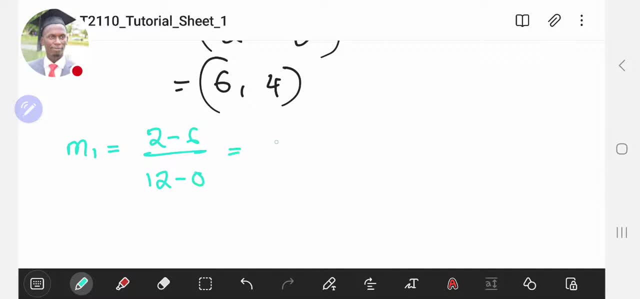 x2 minus x1, that's 12 minus 0. so here i'm going to have 12, i'm going to have 12, i'm going to have 12 minus 0, and this is going to be minus 4 in minus 0, and this is going to be minus 4 in. 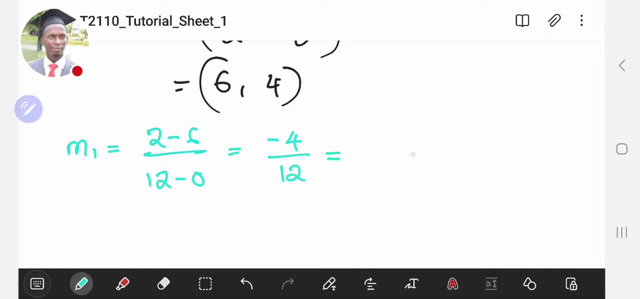 minus 0 and this is going to be minus 4 in the numerator, the numerator. the numerator divided by 12 here. so this is just minus divided by 12 here. so this is just minus divided by 12 here, so this is just minus 1. 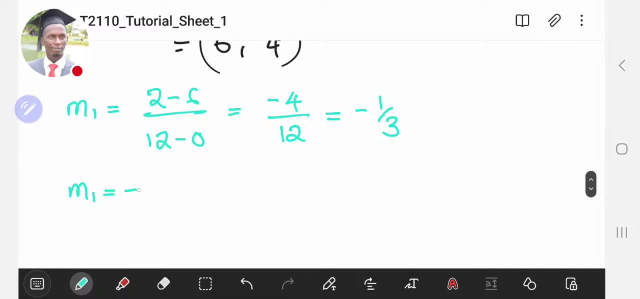 1, 1 over 3. so my gradient m1 is now just over 3. so my gradient m1 is now just over 3. so my gradient m1 is now just going to be minus 1, going to be minus 1, going to be minus 1 over 3, since you have your gradient now. 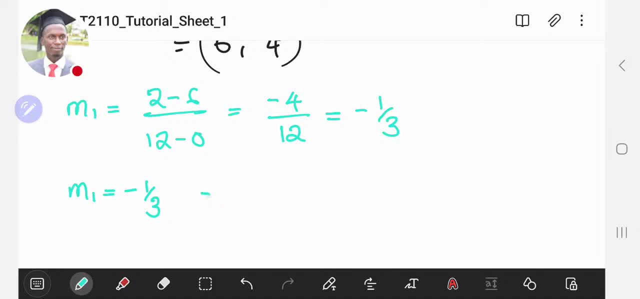 over 3, since you have your gradient now over 3, since you have your gradient now as minus 1 over 3, as minus 1 over 3, as minus 1 over 3, the next thing that we can do is to find. the next thing that we can do is to find. 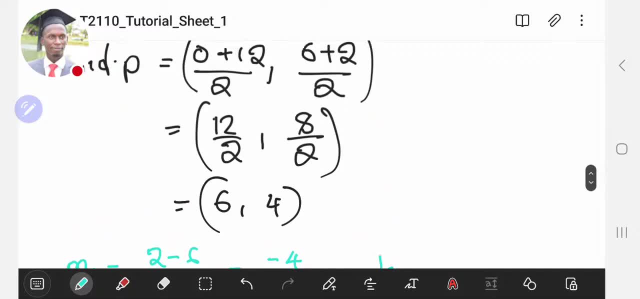 the next thing that we can do is to find the gradient of m, the gradient m2. so the gradient of m, the gradient m2. so the gradient of m, the gradient m2. so again, remember the relationship that we again remember the relationship that we again remember the relationship that we wrote earlier on. 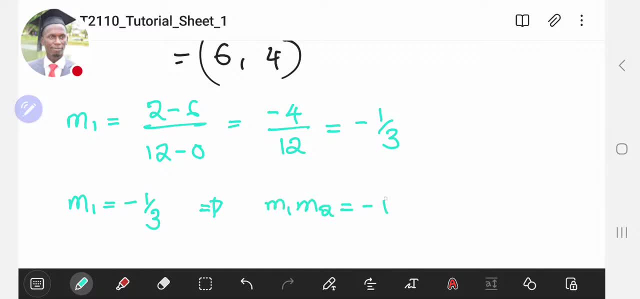 wrote earlier on. wrote earlier on. m1 multiplied with m2 will be equal to m1. multiplied with m2 will be equal to m1. multiplied with m2 will be equal to minus 1. since we know what m1 is, that's minus 1. since we know what m1 is, that's. 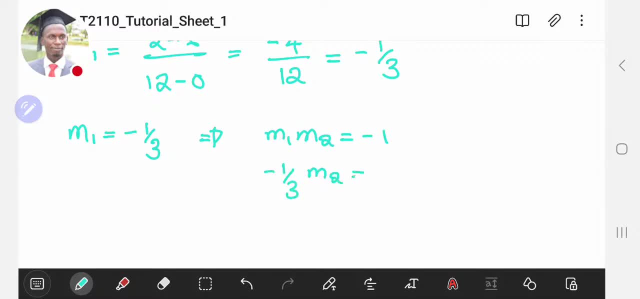 minus 1, since we know what m1 is. that's minus 1 over 3, we can easily get what m2. minus 1 over 3, we can easily get what m2 minus 1 over 3, we can easily get what m2 is going to be. 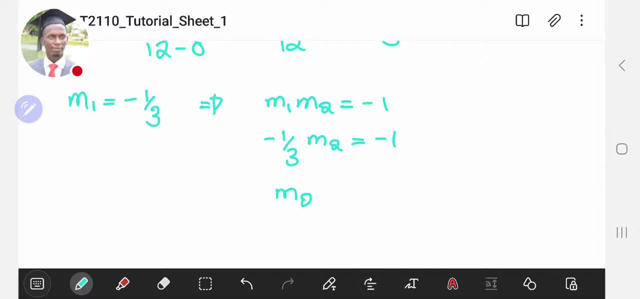 is going to be, is going to be, and from here you should see that m2, and from here you should see that m2, and from here you should see that m2 will just come out to be, will just come out to be, will just come out to be positive 3.. so what does this tell us? 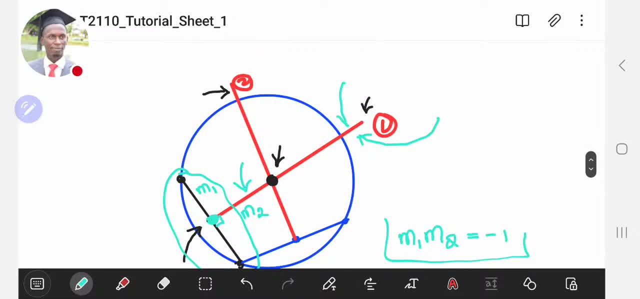 positive 3.. so what does this tell us? positive 3.. so what does this tell us? it tells us that the gradient of this. it tells us that the gradient of this. it tells us that the gradient of this line, line, line, the red line, labeled one, its gradient. 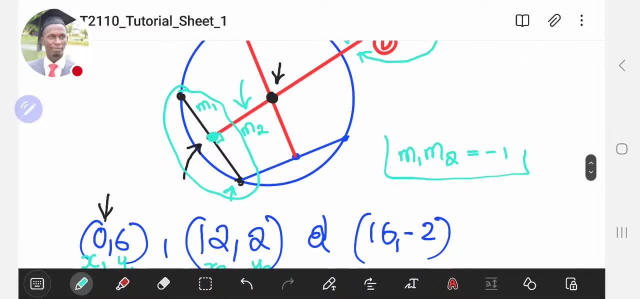 the red line labeled one its gradient. the red line labeled one its gradient. m2 is actually just three now. look at m2 is actually just three now. look at m2 is actually just three now. look at what this implies. what this implies, what this implies if i was to remove this black line, not 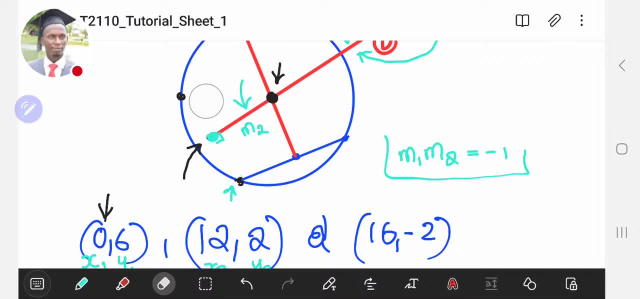 if i was to remove this black line- not if i was to remove this black line, not, not there, not everything. if i was to not there, not everything. if i was to not there, not everything. if i was to remove this part here, remove this part here. remove this part here. notice that now we know. 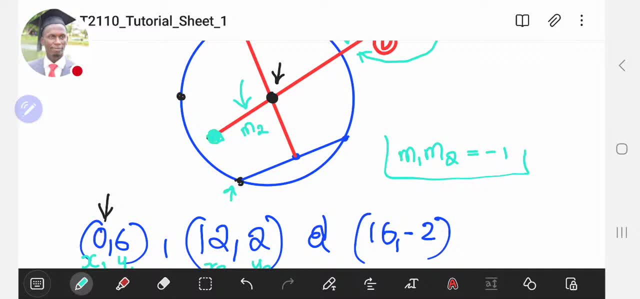 notice that now we know. notice that now we know we know one point on this line. we know we know one point on this line. we know we know one point on this line. we know this point. this is the midpoint of the. this point, this is the midpoint of the. 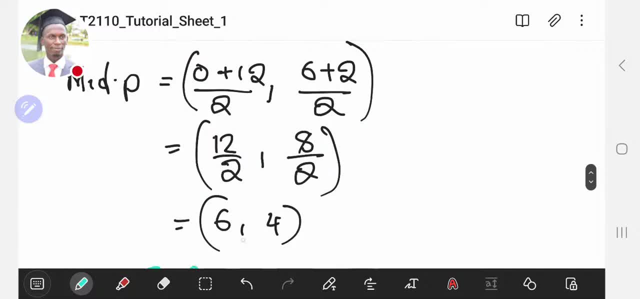 this point. this is the midpoint of the line which i've just erased and remember, line which i've just erased and remember, line which i've just erased and remember. we found the midpoint in the first step, we found the midpoint in the first step, we found the midpoint in the first step. six comma four. so this point is six. 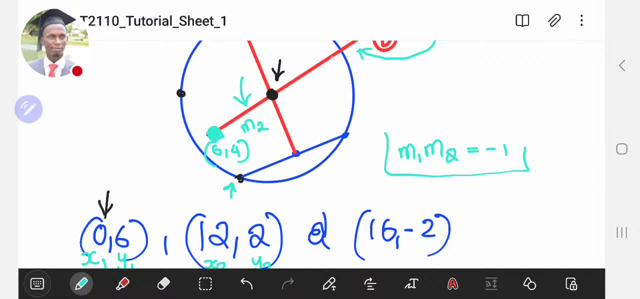 six comma four. so this point is six, six comma four. so this point is six comma four. so we know one point and we comma four. so we know one point and we comma four. so we know one point and we even know the gradient of this line. so 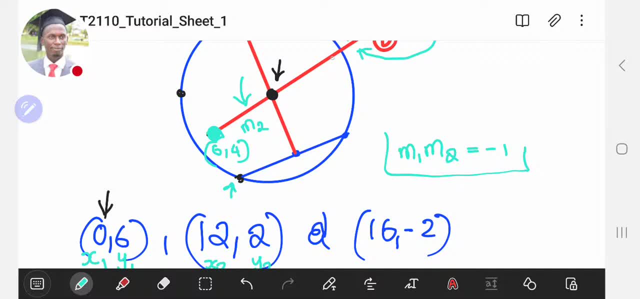 even know the gradient of this line. so even know the gradient of this line. so remember, if you know the midpoint in, remember if you know the midpoint in, remember if you know the midpoint in the gradient, the gradient, the gradient, uh, you can easily get. uh, you can easily get. 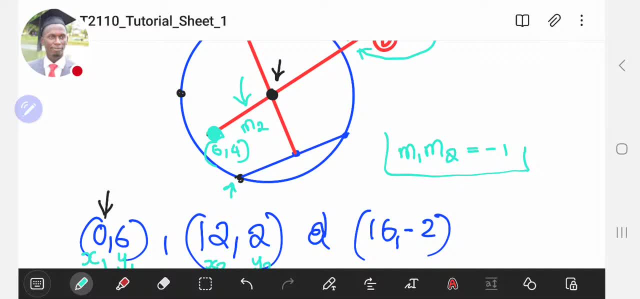 uh, you can easily get. you can easily get um. you can easily get um. you can easily get um. get the equation, so get the equation, so get the equation. so how is the product of the gradients equal? how is the product of the gradients equal? how is the product of the gradients equal to the negative one? it's something that 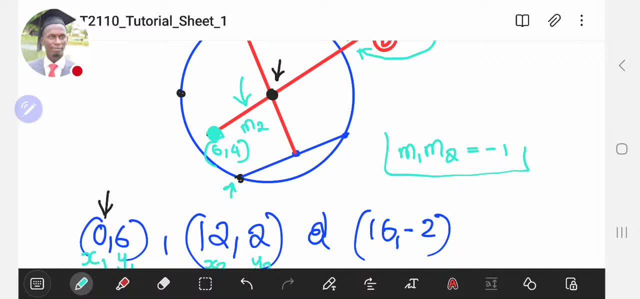 to the negative one. it's something that to the negative one. it's something that you can easily show. you can easily show. you can easily show, but it has been proven. i think a number, but it has been proven. i think a number, but it has been proven, i think, a number of times before. 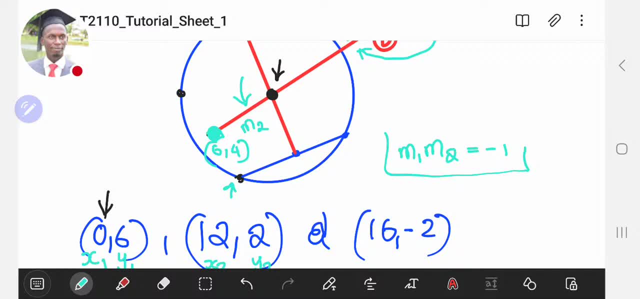 of times before, of times before i i won't prove it here, but some that i i won't prove it here, but some that i i won't prove it here, but some that you can just take advantage of. you can just take advantage of, you can just take advantage of the gradient of two lines which are 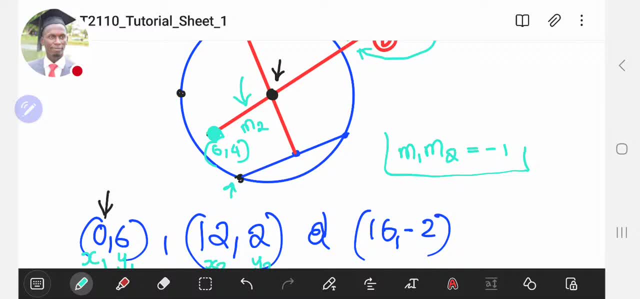 the gradient of two lines which are the gradient of two lines which are perpendicular, perpendicular, perpendicular. when you multiply them, let's say you have. when you multiply them, let's say you have. when you multiply them, let's say you have two, two lines which are perpendicular to. 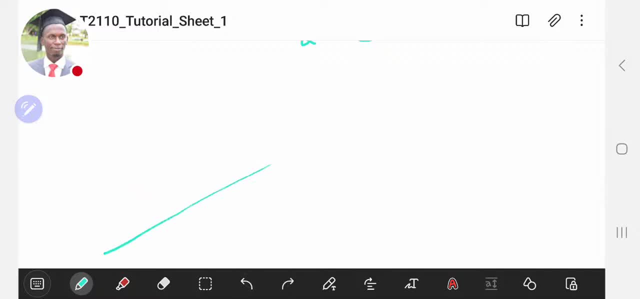 two, two lines which are perpendicular to two, two lines which are perpendicular to each other, each other, each other. so you have one, let me not draw them. so so you have one, let me not draw them. so so you have one, let me not draw them. so obviously, you have one line like this: 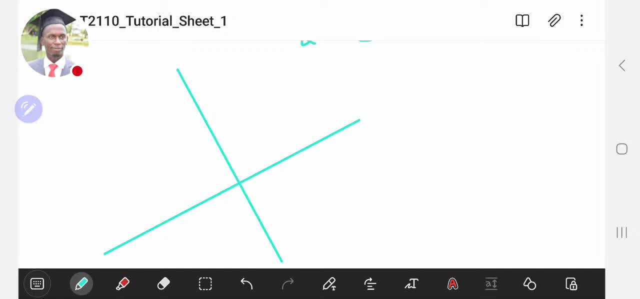 obviously you have one line like this. obviously you have one line like this, and then you have another line that is, and then you have another line that is, and then you have another line that is like this, like this, like this, if these two lines are perpendicular to: 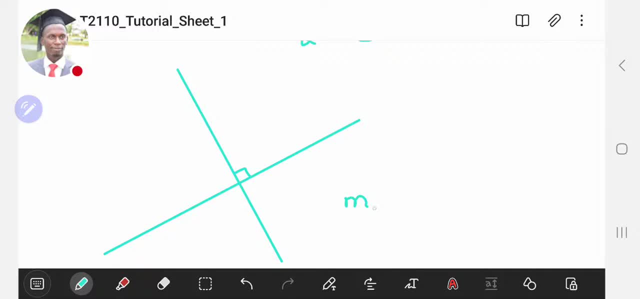 if these two lines are perpendicular to, if these two lines are perpendicular to each other, each other, each other, they need to imply that, if you multiply, they need to imply that, if you multiply, they need to imply that, if you multiply the gradient of the first line, the gradient of the first line. 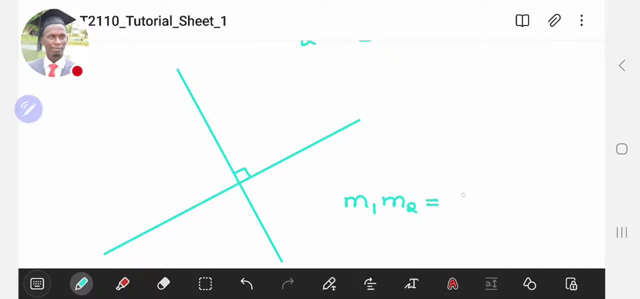 the gradient of the first line times the gradient of the second line, times the gradient of the second line, times the gradient of the second line. this product will actually give you a. this product will actually give you a. this product will actually give you a negative one, negative one. 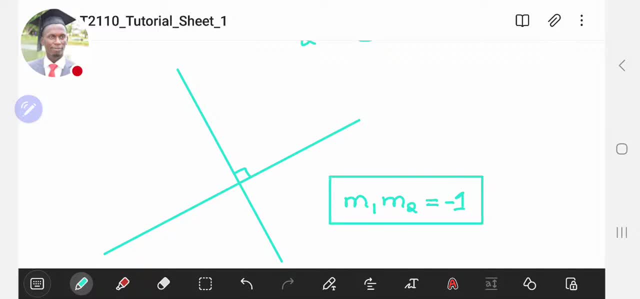 negative one. you can try to find two lines which are: you can try to find two lines which are: you can try to find two lines which are directly perpendicular and try to see if directly perpendicular. and try to see if directly perpendicular and try to see if this holds. 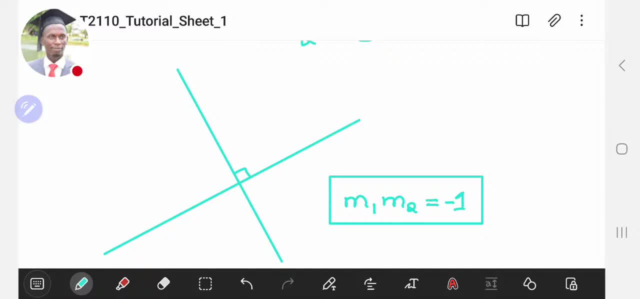 this holds, this holds, but it's something that can be proven. but it's something that can be proven, but it's something that can be proven, but in this case we're not trying to. but in this case we're not trying to. but in this case we're not trying to prove it, just trying to take advantage. 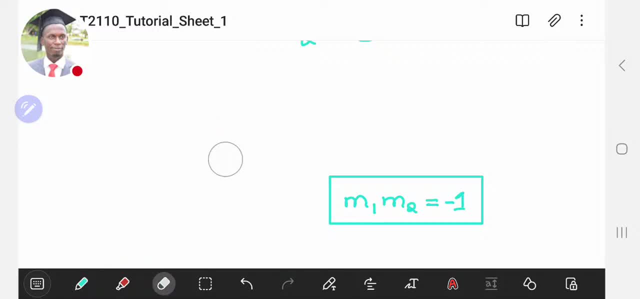 prove it, just trying to take advantage, prove it, just trying to take advantage of it, of it, of it okay. so, having found it okay, so, having found it okay, so having found it, um the gradient of m, the gradient m2, um the gradient m2, um the gradient m2 to be to be positive three, we can easily 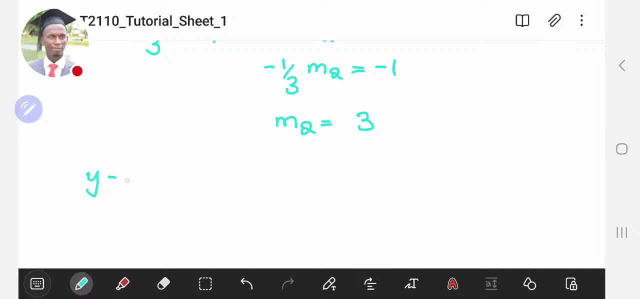 to be to be positive three. we can easily to be to be positive three. we can easily get the equation for that line we know. get the equation for that line. we know. get the equation for that line. we know the equation of a line is given by y. 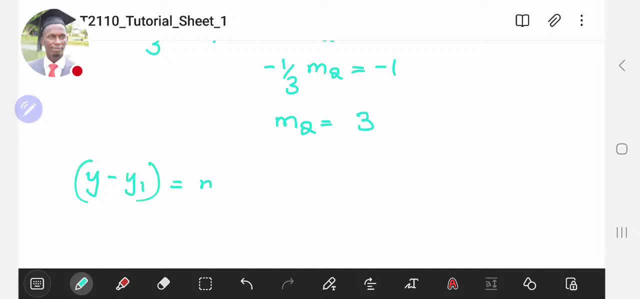 the equation of a line is given by y. the equation of a line is given by y minus y1, minus y1 minus y1, equal to the gradient, and then you have x equal to the gradient, and then you have x equal to the gradient, and then you have x minus x1. 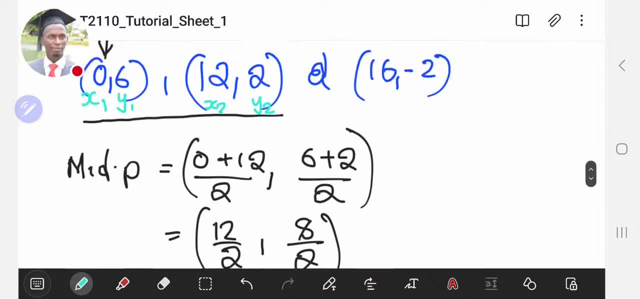 minus x1. minus x1, then here you're going to have y minus y1. then here you're going to have y minus y1, then here you're going to have y minus y1. so in this case, y1- y1 has to just be. 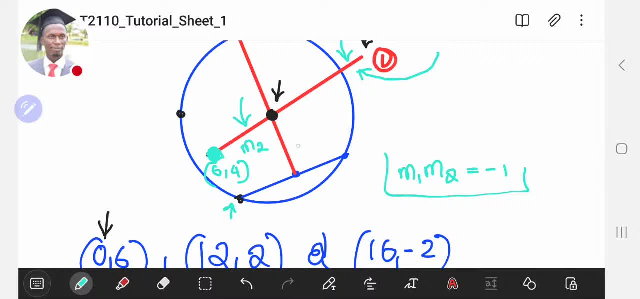 so, in this case, y1, y1 has to just be so. in this case, y1- y1 has to just be any point along this line, which you've, any point along this line, which you've, any point along this line which you've labeled one in red. 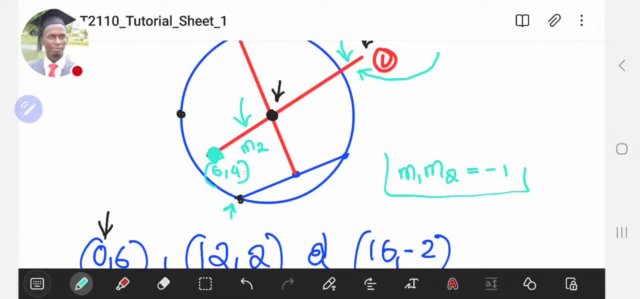 labeled one in red. labeled one in red. so in this case we're going to take the. so in this case we're going to take the. so in this case we're going to take the midpoint one we got earlier this side, midpoint one we got earlier this side. 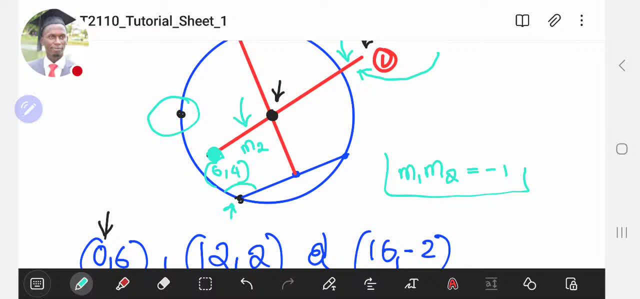 midpoint, one we got earlier this side. the midpoint don't be tempted to use any. the midpoint don't be tempted to use any. the midpoint don't be tempted to use any of the three points which are given for of the three points which are given for of the three points which are given for this part. 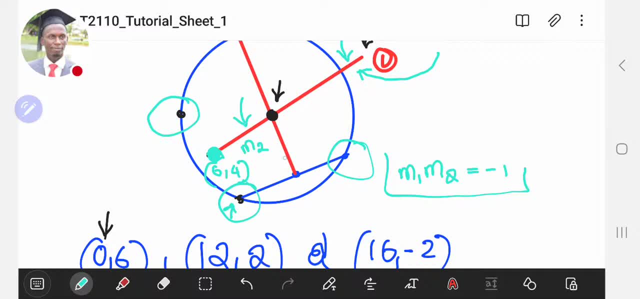 this part, this part, these points do not lie on this line. these points do not lie on this line. these points do not lie on this line that is passing to the center, so that that is passing to the center, so that that is passing to the center, so that this is why we found the midpoint here. 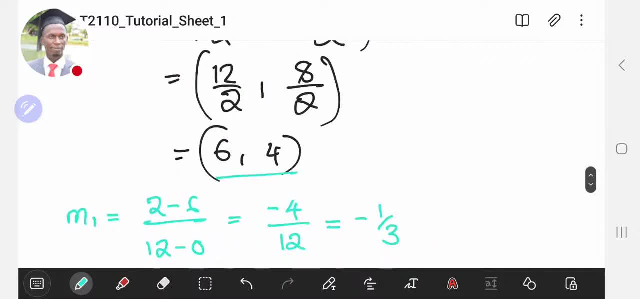 this is why we found the midpoint here. this is why we found the midpoint here, so i'm going to use the midpoint, the. so i'm going to use the midpoint, the. so i'm going to use the midpoint. the midpoint was 6.4. midpoint was 6.4. 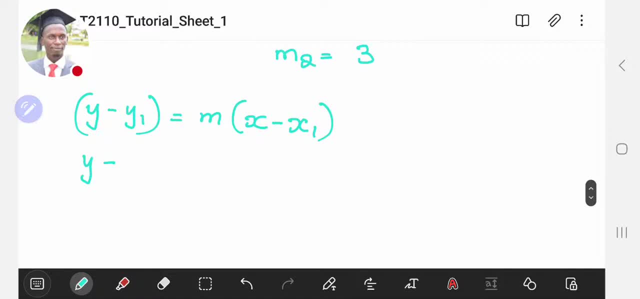 midpoint was 6.4, so we're going to have. its x value is 6, so we're going to have. its x value is 6, so we're going to have. its x value is 6. its y value is 4, so we're going to have. 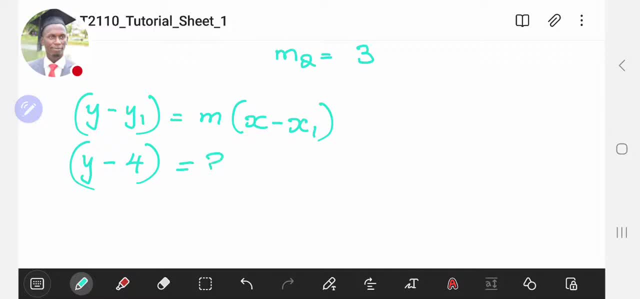 its y value is 4, so we're going to have. its y value is 4, so we're going to have minus 4 here, minus 4 here, minus 4 here, equal to the gradient we've just found, equal to the gradient we've just found. 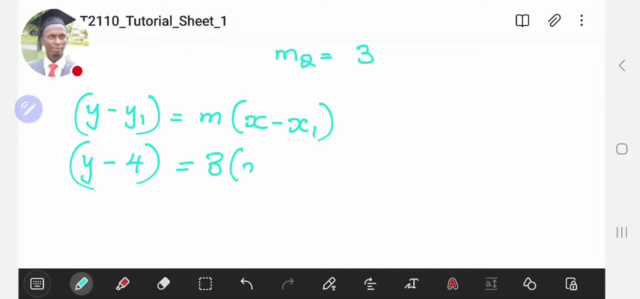 equal to the gradient. we've just found 3 for the gradient, 3 for the gradient, 3 for the gradient, and then x again, so we have x and then x again, so we have x and then x again. so we have x minus minus, minus the y value, the x value, i mean which? 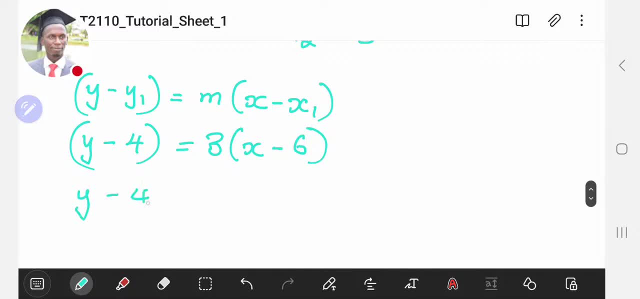 the y value, the x value, i mean which? the y value, the x value, i mean which was six, was six, was six. so from here this equation becomes y, so from here this equation becomes y, so from here this equation becomes y minus 4 is equals to 3x. 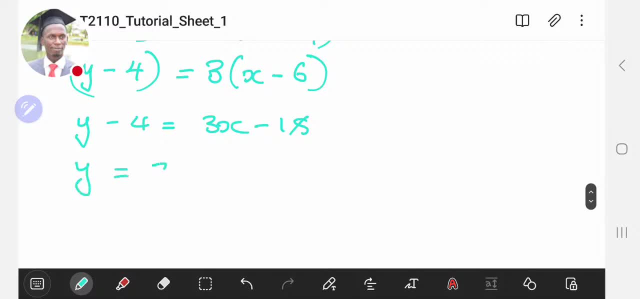 minus 4 is equals to 3x minus 4 is equals to 3x minus 18, so that you have y is equals minus 18, so that you have y is equals minus 18, so that you have y is equals to 3x. 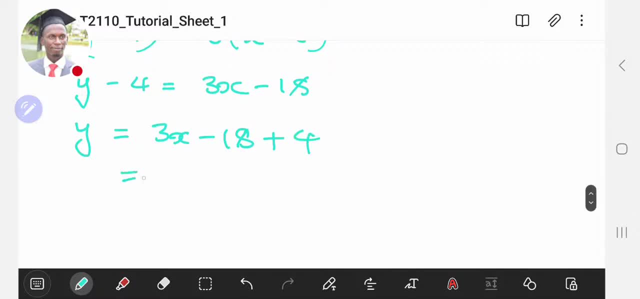 to 3x to 3x minus 18 plus 4. so this is now just 3x minus 18 plus 4. so this is now just 3x minus 18 plus 4. so this is now just 3x minus 14. this becomes the equation. 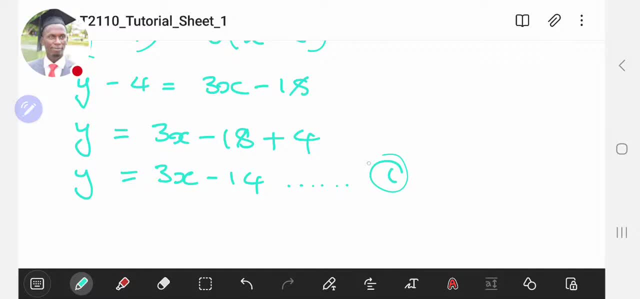 minus 14. this becomes the equation minus 14. this becomes the equation that passes through the center, the first that passes through the center, the first that passes through the center, the first equation passing through the center. equation passing through the center. equation passing through the center. now, i hope you get the trick here. 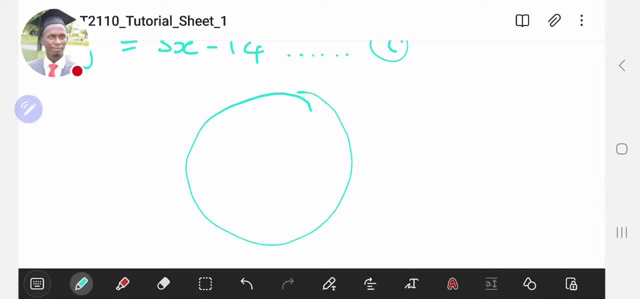 now. i hope you get the trick here now. i hope you get the trick here again, again, again. the method that we are using here works. the method that we are using here works. the method that we are using here works on this concept, on this concept, on this concept. find one line. 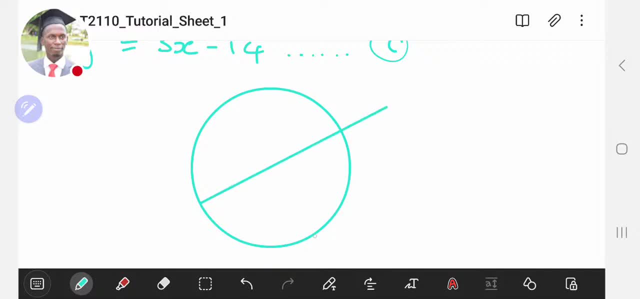 find one line, find one line that passes through the center, that passes through the center, that passes through the center. then find the second line that passes, then find the second line that passes, then find the second line that passes through the center, through the center, through the center. then equate these two points, since they 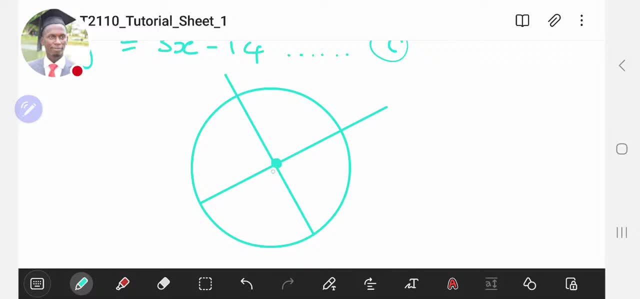 then equate these two points, since they then equate these two points, since they meet at the center, meet at the center, meet at the center. once you equate, get the value for of x. once you equate, get the value for of x. once you equate, get the value for of x where they meet and they get the x value. 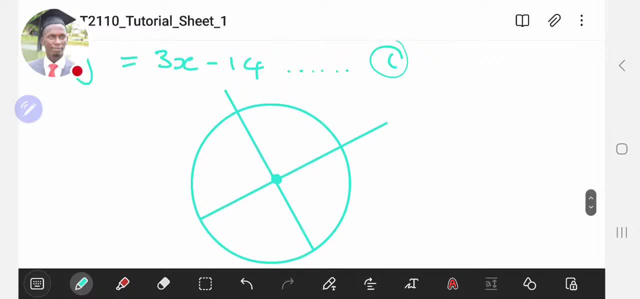 where they meet and they get the x value where they meet and they get the x value for where they meet. those will be the for where they meet. those will be the for where they meet. those will be the coordinates of the center. coordinates of the center. coordinates of the center. we have found one equation passing. 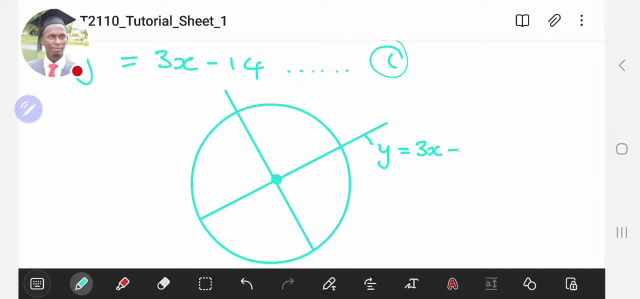 we have found one equation passing. we have found one equation passing: through the center which is y is equals through the center which is y is equals through the center which is y is equals to 3x to 3x to 3x minus 14.. now we want to find: 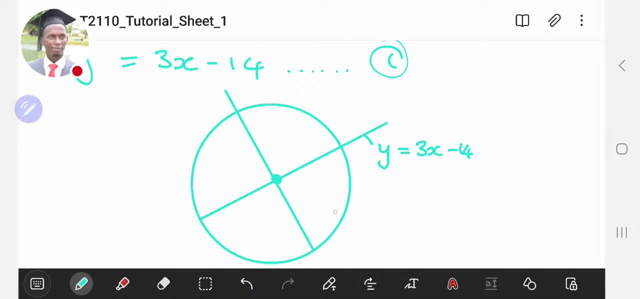 minus 14.. now we want to find minus 14.. now we want to find the second equation, the second line, the second equation, the second line, the second equation, the second line, passing through the center, to find this, passing through the center, to find this passing through the center, to find this second equation. 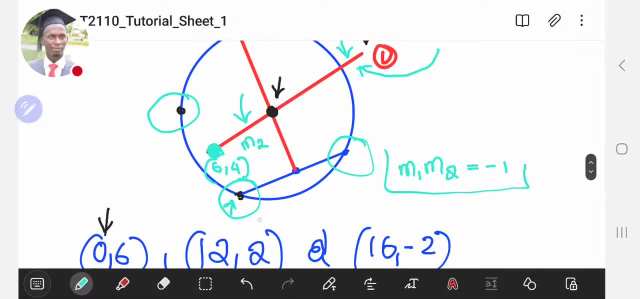 second equation. second equation: we're going to go back to this part. we're going to go back to this part. we're going to go back to this part, but we are done with the first part, we're, but we are done with the first part, we're. 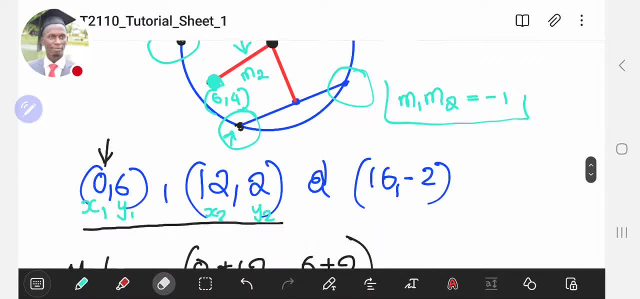 but we are done with the first part. we're just going to use, just going to use, just going to use two coordinates again: if you used, if you used, six comma zero, comma six, and if you used six comma zero, comma six, and if you used six comma zero comma six and twelve comma two. 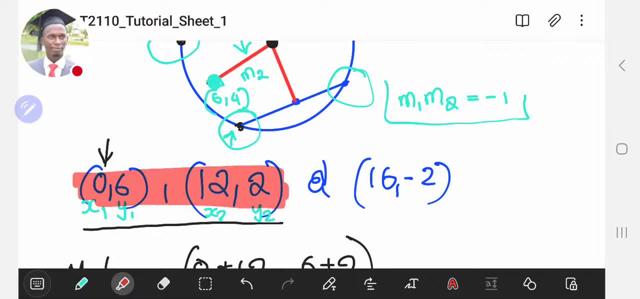 twelve comma two. twelve comma two, to get the first equation now use. you want to get the first equation now use. you want to get the first equation now use. you want another pair, so for the second pair. another pair, so for the second pair. another pair, so for the second pair we're now going to use. 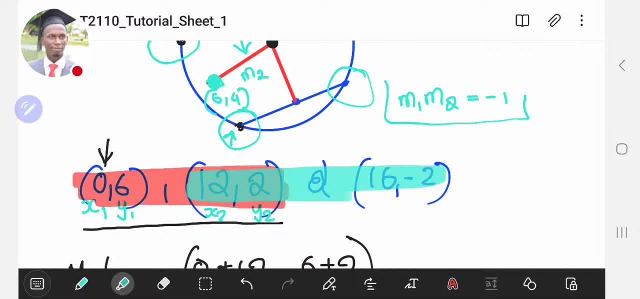 we're now going to use. we're now going to use the 12 comma 2 and the 12 comma 2 and the 12 comma 2 and 16 comma negative 2.. this is the pair: 16 comma negative 2.. this is the pair. 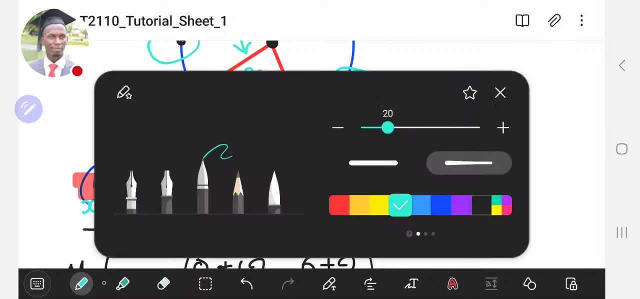 16 comma, negative 2.. this is the pair that we're going to use to come up with, that we're going to use to come up with that we're going to use to come up with the second equation, the second equation, the second equation, because now it's like i'm saying this: because now it's like i'm saying this, because now it's like i'm saying: this is where my 12 comma 2 is, of course, is where my 12 comma 2 is, of course, is where my 12 comma 2 is of course. this is not to stand, i'm just putting. this is not to stand. i'm just putting this is not to stand. i'm just putting the points there, the points there, the points there. this is where my 12 comma 2 is, and this: this is where my 12 comma 2 is, and this. 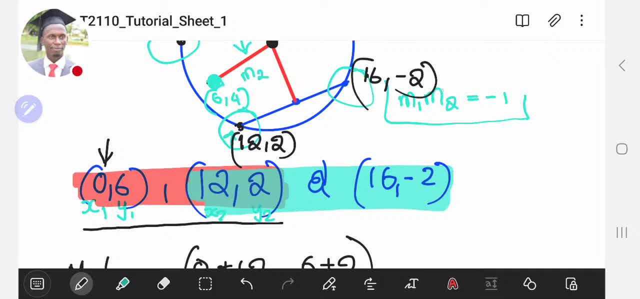 this is where my 12 comma 2 is and this is where my 16 is, where my 16 is, where my 16 comma negative 2 is. so, since i have these comma negative 2 is so, since i have these comma negative 2 is so, since i have these two points, 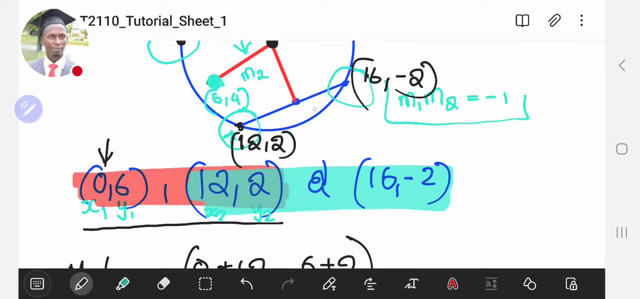 two points, two points. the first step, again just like before. the first step, again just like before the first step, again just like before. get the midpoint. once you have the, get the midpoint. once you have the, get the midpoint. once you have the midpoint, midpoint, midpoint, get the gradient. after the gradient use. 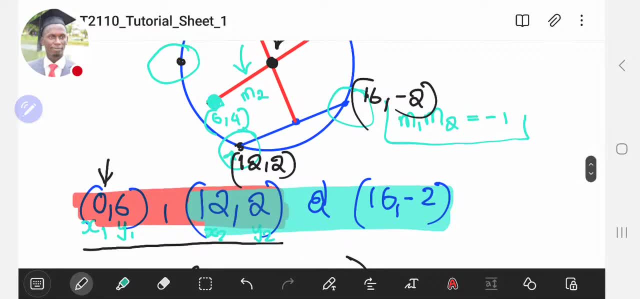 get the gradient after the gradient use. get the gradient after the gradient use that m1 by m2, that m1 by m2, that m1 by m2 being equal to negative one, to find the being equal to negative one. to find the being equal to negative one. to find the gradient of this red line. that's the. 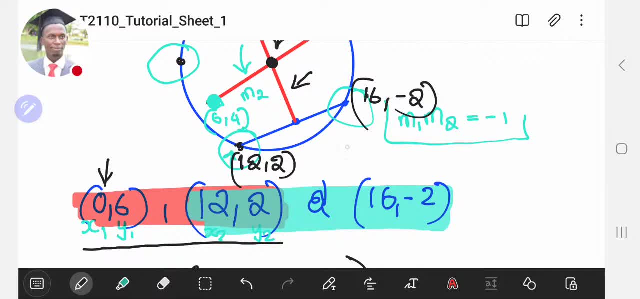 gradient of this red line. that's the gradient of this red line, that's the. that's our target, that's where we're, that's our target, that's where we're, that's our target, that's where we're going, going, going. so let's see, let's get the midpoint of. 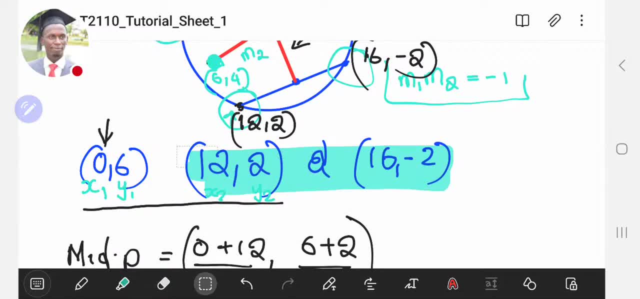 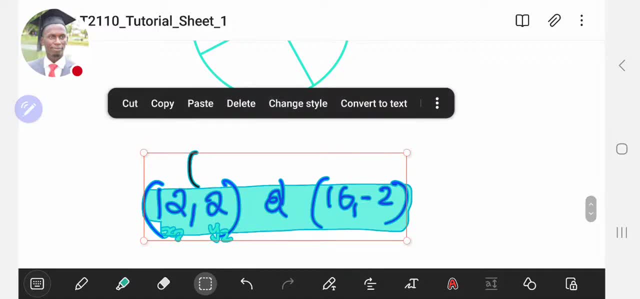 so let's see, let's get the midpoint of. so let's see, let's get the midpoint of these two points, these two points, these two points. so i want just these two, so let me get. so i want just these two, so let me get. so i want just these two, so let me get those. 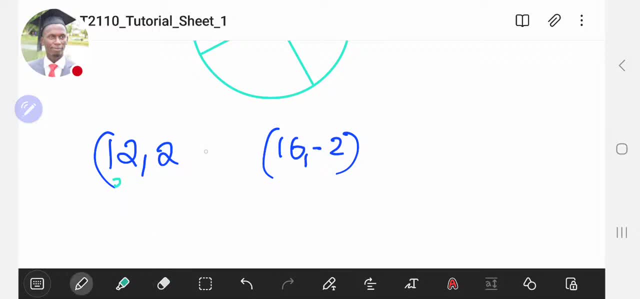 okay, so first thing is their midpoint. okay, so, first thing is their midpoint. okay, so first thing is their midpoint. so the midpoint here, so the midpoint here, so the midpoint here is going to be equal to again, is going to be equal to again, is going to be equal to again. x1 plus x2, so x1 will take 12. 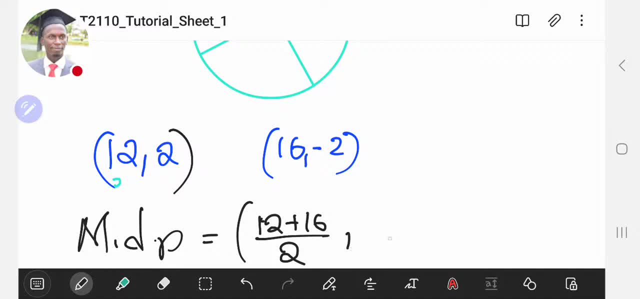 x1 plus x2, so x1 will take 12, x1 plus x2, so x1 will take 12 plus 16, divided by 2 plus 16, divided by 2 plus 16, divided by 2 comma, comma, comma comma y1, y1 will take 2. 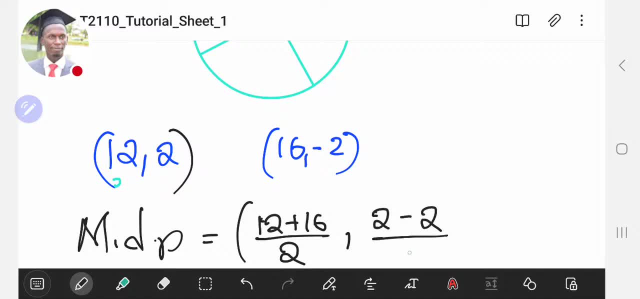 y1- y1 will take 2- y1- y1 will take 2 plus negative. 2- that's just going to be plus negative. 2, that's just going to be plus negative. 2, that's just going to be minus 2, minus 2. 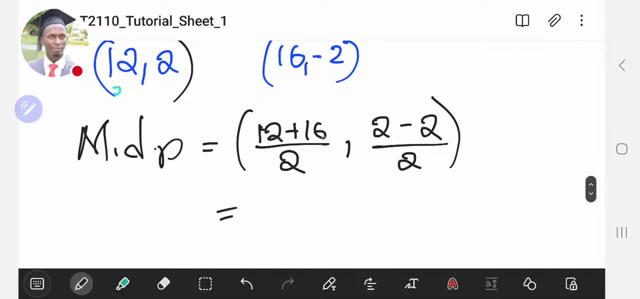 minus 2 over 2. so this becomes over 2. so this becomes over 2. so this becomes, when we add these two. this is going to when we add these two. this is going to: when we add these two. this is going to be 28. 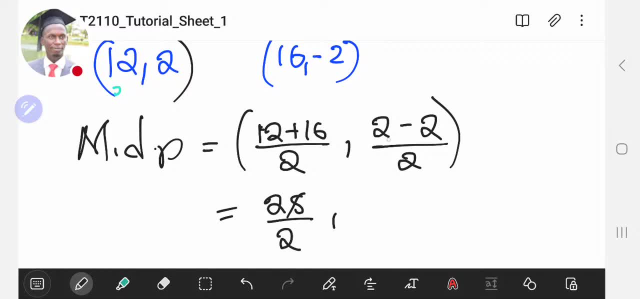 be 28, be 28. we're going to have 28 here divided by 2. we're going to have 28 here divided by 2. we're going to have 28 here divided by 2 comma. this is just going to be zero, this. 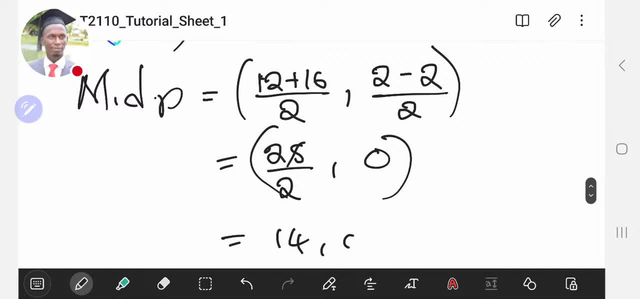 comma, this is just going to be zero. this comma, this is just going to be zero. this side side side. so this becomes 14 comma zero. so this becomes 14 comma zero. so this becomes 14 comma zero. so this becomes the midpoint here. so you, so this becomes the midpoint here, so you. 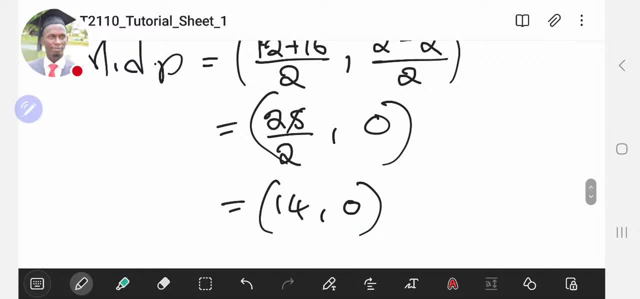 so this becomes the midpoint here. so you guys should be following um. guys should be following um. guys should be following um. yeah, if at all you spot something that. yeah, if at all you spot something that. yeah, if at all you spot something that i've just um. 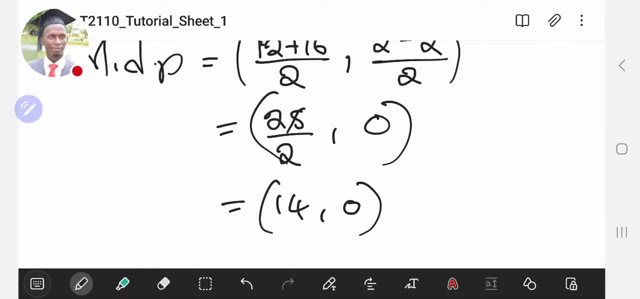 i've just um. i've just um a quick math error, just be able to point a quick math error, just be able to point a quick math error, just be able to point it out. but i'll try by all means to it out, but i'll try by all means to. 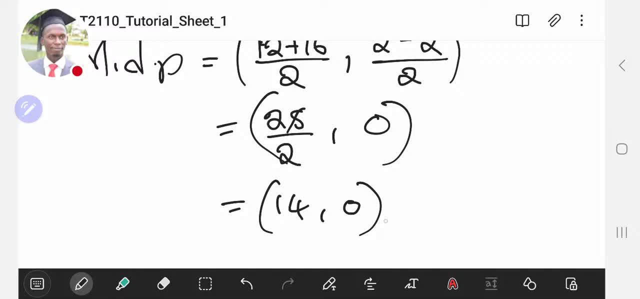 it out, but i'll try by all means to counter check my work. counter check my work. counter check my work. okay, so this becomes 14 comma comma zero. okay, so this becomes 14 comma comma zero. okay, so this becomes 14 comma comma zero as the midpoint. 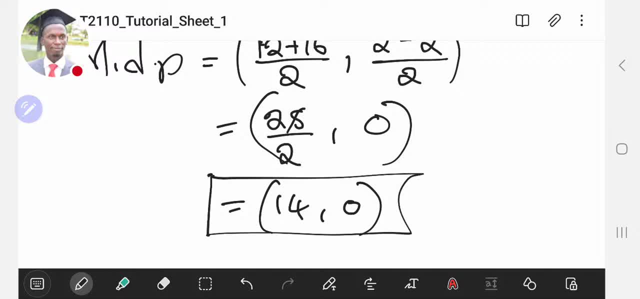 as the midpoint, as the midpoint. now that we know the midpoint, the next, now that we know the midpoint, the next, now that we know the midpoint, the next step is going to get the gradient of step, is going to get the gradient of step, is going to get the gradient of the line at the bottom. so i want to get. 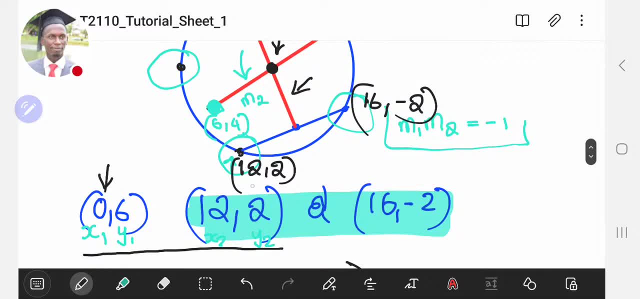 the line at the bottom. so i want to get the line at the bottom, so i want to get the gradient of the gradient of the gradient of this line here, the one running from 12. this line here, the one running from 12. this line here, the one running from 12, comma 2. 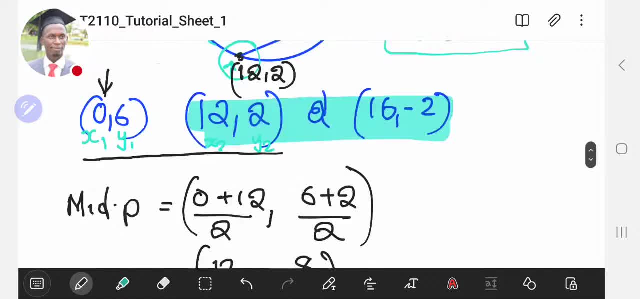 comma 2. comma 2 to 16 comma negative 2 to 16 comma negative 2 to 16 comma negative 2. how do we get the gradient? this is going. how do we get the gradient? this is going. how do we get the gradient? this is going to be our gradient. 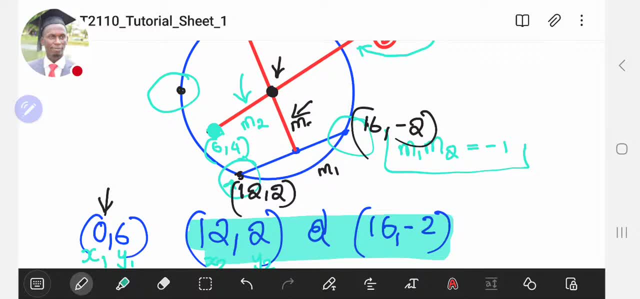 to be our gradient, to be our gradient m1, and then this is going to be the one m1, and then this is going to be the one m1, and then this is going to be the one. here, this is going to have gradient m2. here, this is going to have gradient m2. 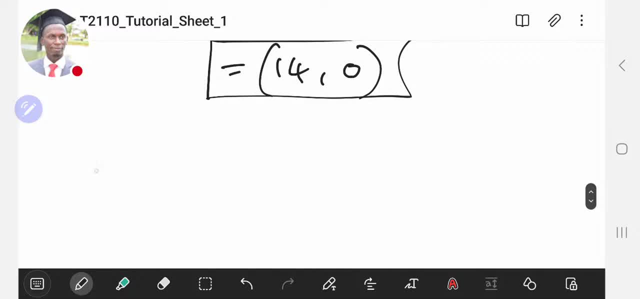 here, this is going to have gradient m2. so how do we proceed with that? so how do we proceed with that? so how do we proceed with that? so we know to say the gradient m1 will. so we know to say the gradient m1 will. so we know to say the gradient m1 will be equal to, again, it's y2 minus y1. 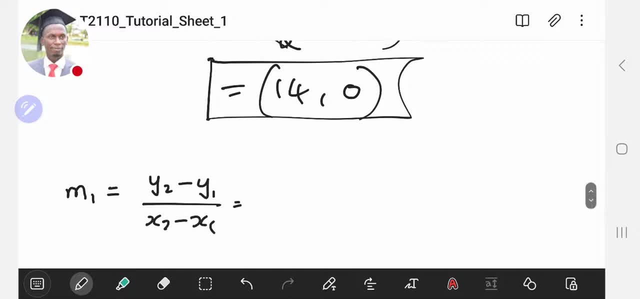 be equal to- again it's y2 minus y1. be equal to- again it's y2 minus y1 over x2 minus x1. so this proceeds over x2 minus x1. so this proceeds over x2 minus x1. so this proceeds, uh, y2. so i, i'm taking, i'll take this. 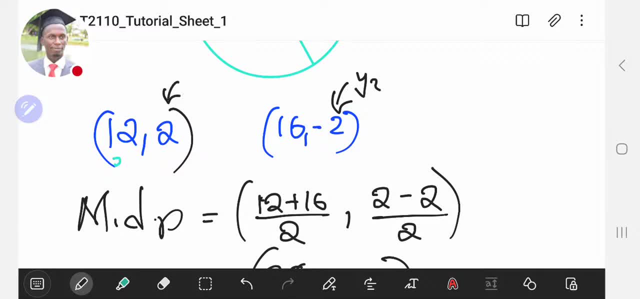 uh, y2. so i i'm taking: i'll take this, uh, y2, so i i'm taking i'll take this to be y2, to be y2 to be y2 and this to be y1, and this to be y1 and this to be y1, so that we have minus 2, minus 2 that. 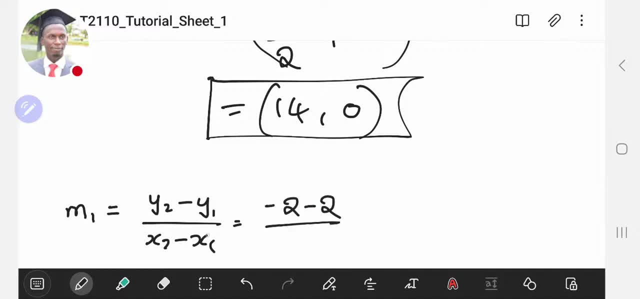 so that we have minus 2 minus 2. that, so that we have minus 2 minus 2, that will be minus 2 will be minus 2 minus 2 will be minus 2 minus 2 will be minus 2 minus 2 divided by x2, so x2 will be 16. 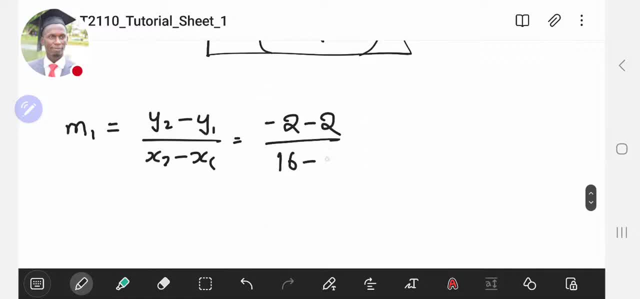 divided by x2, so x2 will be 16. divided by x2, so x2 will be 16, x1 will be 12.. so this is going to be: x1 will be 12.. so this is going to be: x1 will be 12.. so this is going to be 16. 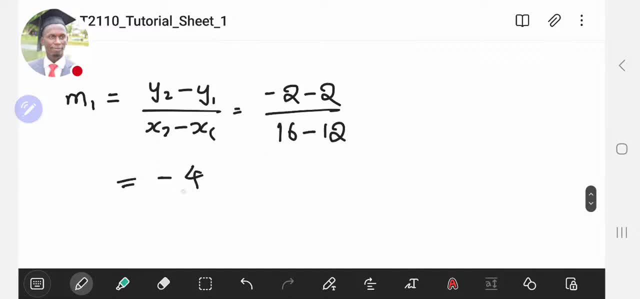 16, 16 minus 12.. so this becomes minus 4 minus 12.. so this becomes minus 4 minus 12.. so this becomes minus 4 over. when i get the difference here, this over, when i get the difference here, this over, when i get the difference here, this is going to be: 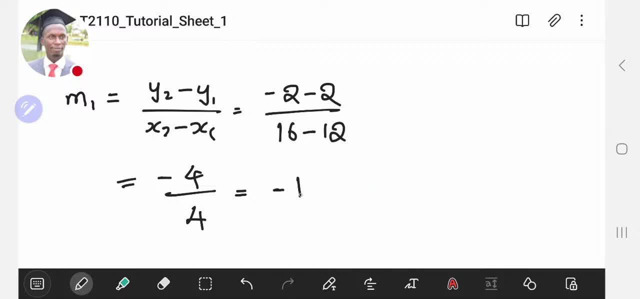 is going to be is going to be to b4, so that in the end this becomes to b4, so that in the end this becomes to b4, so that in the end this becomes minus 1.. minus 1.. minus 1.. so this becomes the gradient m1. m1 is 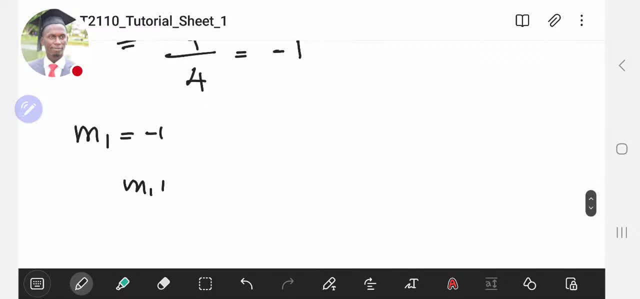 so this becomes the gradient m1. m1 is, so this becomes the gradient m1. m1 is equals to, equals to equals to minus one. so again: m1 times m2 minus one. so again m1 times m2 minus one. so again: m1 times m2 is equal to minus one. so that since m1. 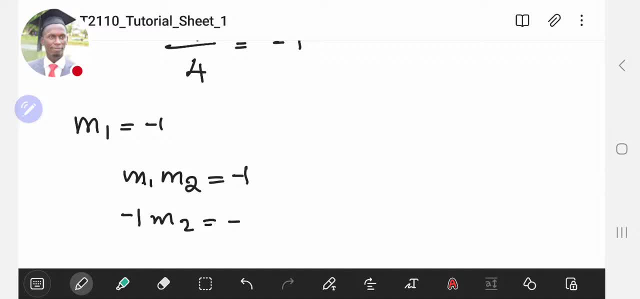 is equal to minus one, so that since m1 is minus one, we're going to have minus one. m2 is equals to minus one, so that m2 is just equal to one. now we know the gradient of the second line, so we can easily get what the second line is going. 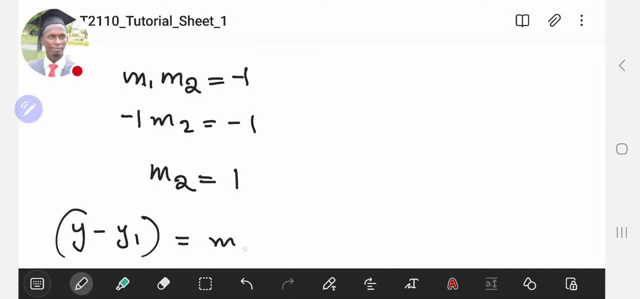 to be y1 equal to its gradient, which is m2, x minus x1. so from here we need a point that where this line passes- and remember this point, we got it earlier on- that's the midpoint we calculated here and remember the midpoint- we had 14 comma 0. so this is going to be y minus y1 is a. 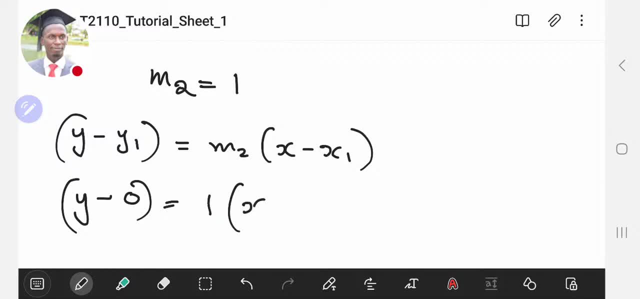 0, equal to the gradient is 1. then you have x minus x1, which is 14. from here we end up with y. this equals to x minus 14. this becomes the second equation. once you have the two equations, to find the center of this. 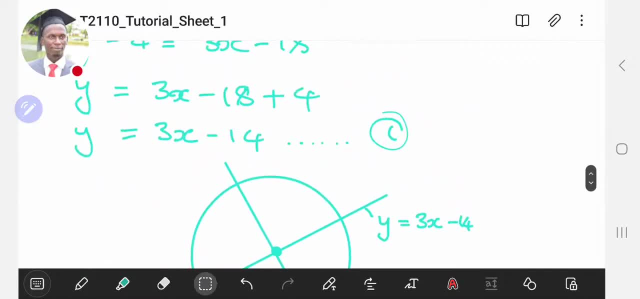 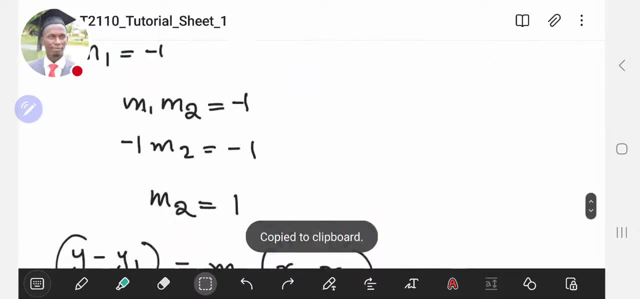 circle, just get where the two equations meet. so this was the first equation we came up with. sorry, i don't want to cut it. so that was the second equation. that was the first. this is the second that we've just written here. so now we can easily equate these two, since at the center that is where they meet. so at the center. 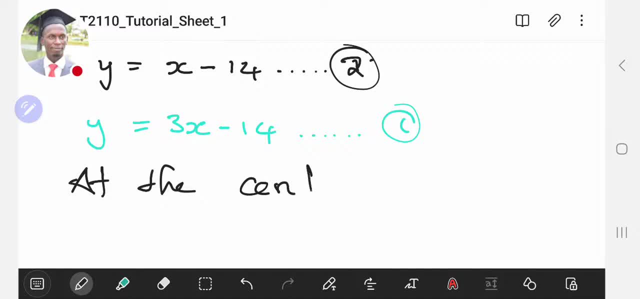 what do we see there? so at the center we have- i'll equate- the right hand side. since the left hand sides are the same, we're going to have x minus 14. we'll have to be equal to 3x minus 14. from here you should see that this becomes minus 14 plus 14 when the 14 crosses, and then the other. 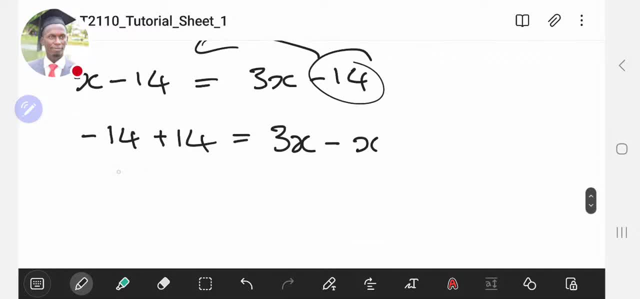 side. we're going to have 3x minus x, so that the left hand side becomes 0, the right hand side becomes 2x. 2 cannot be equal to 0, so it implies that x is equal to 0. so this is telling us that 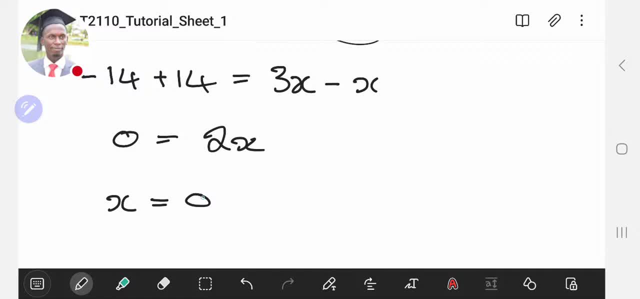 where these two lines are actually meeting, the x and the y are equal to 0. so we're going to have x minus 14 so that we can easily get the y value. we can pick any of these equations. i'll pick equation equation 1. from equation 1 we had, y is equal to. i think i still have it. let's paste it. so this was equation. 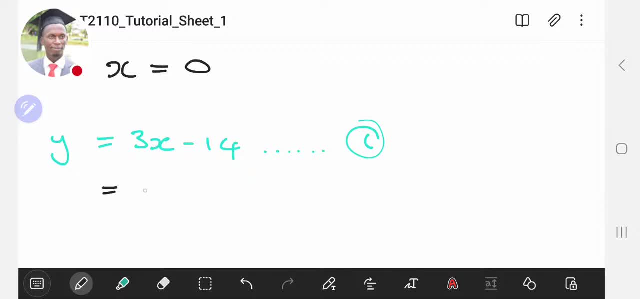 1. so if we put the y, the x value as a 0, this becomes 3 multiplying 0 minus 14, so that we see that the y value becomes minus 14. so what does this tell us? it tells us that our circle, we square it by the y value, so we can easily get the y value. so we can easily get the y value. 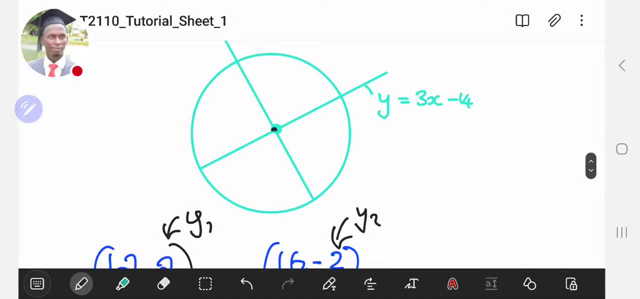 sketched it somewhere here. this circle where the two lines meet where the center is. apparently it's at 0 comma minus 14. this is where the center is. so we now know the coordinates of the center. with the coordinates of the center, now getting the equation of the circle is actually easier. 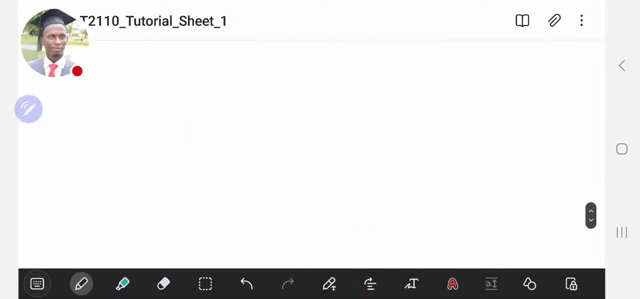 because with the center now, so we have the center of our circle, so the center, we have 0 comma minus 14. so this is going to apply, then: HTML To the center we going to use instead of text we need to do is: we are gifting that center, so we're gifting that center. where's our point? 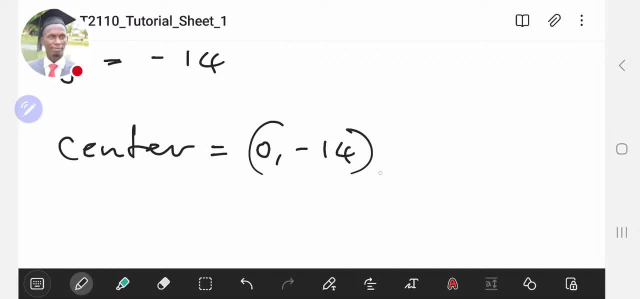 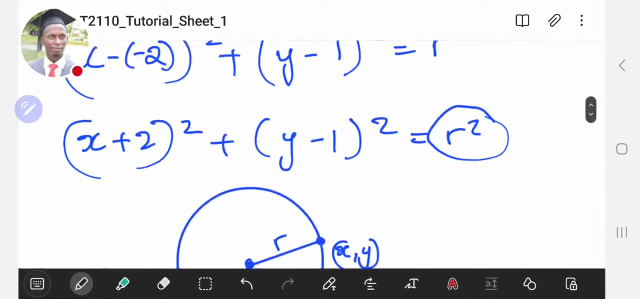 from 0 earlier on. just pick any one of them. in this case i won't work it out, unless if you guys insist. but i'll just pick even the 12 comma two is okay, but let me pick the smaller one. don't want to do with big values, so you can even pick. um which one is that we can pick? 0.6. 0.6 is easier to work. 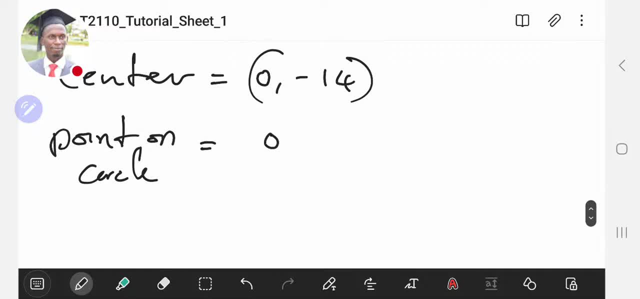 with. so we have 0.6. so this becomes one point on the on the circle. so with this, with these two, we can easily get the equation of of our circle. so we have the center, we have a point on the circle, we can easily work it out to get the equation of the circle. so if you have a question or if you'd 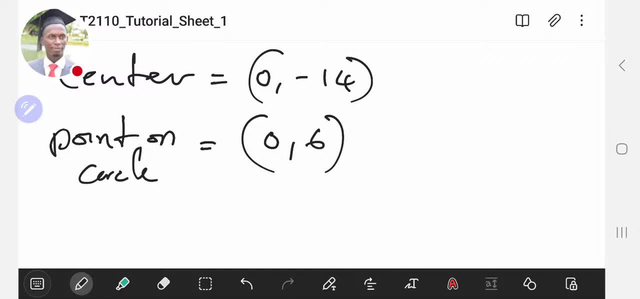 want me to go all the way to find the solution, just comment and i'll be able to do that. if not, you can just try to use the first approach that we did to work out the first question to get the answer for this one. okay, so this uh demonstrates how you answer uh b using this. 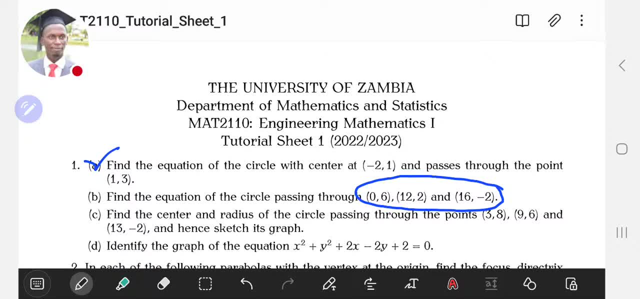 method. the best thing i like about this method is it avoids use, uh, working out a simultaneous equation in three unknowns, which i feel is a little bit. um, it's okay, you can do it, but i always try to avoid simultaneous equations, especially of three unknowns or more. okay, so. 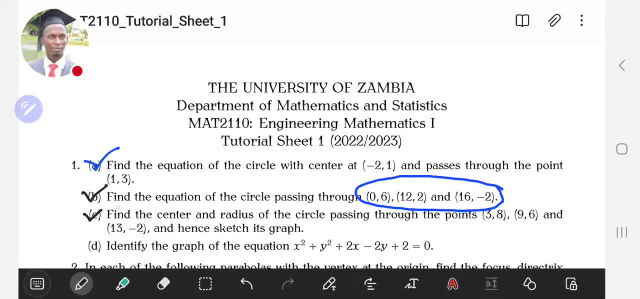 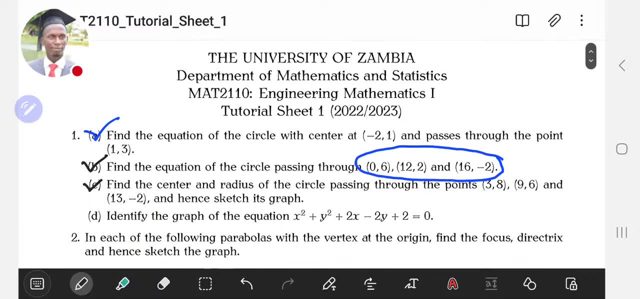 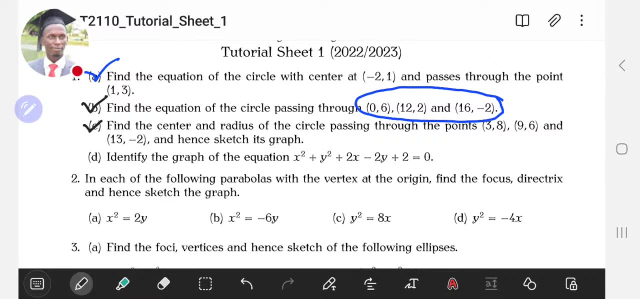 that sorts out this one. we can use the same method to work out c as well, so that gets rid of uh one: a, b, a and c. so if you understand how to do b, you can use the same method to work out c. so we can now move on to look at d. and now the question is: what is happening at with? 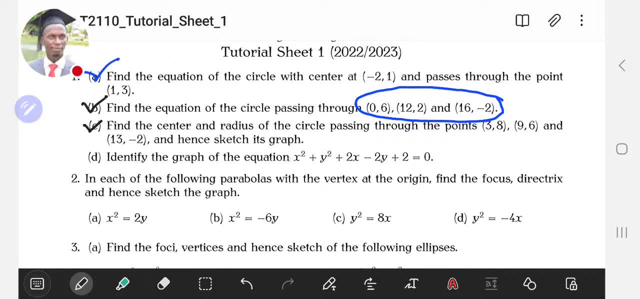 the question d, the saying: identify the graph of the equation. now, to identify um an equation, to identify what you're dealing with, based on just a standard equation, all you have to do is complete the square. so let me get this: x squared plus y squared plus 2x. 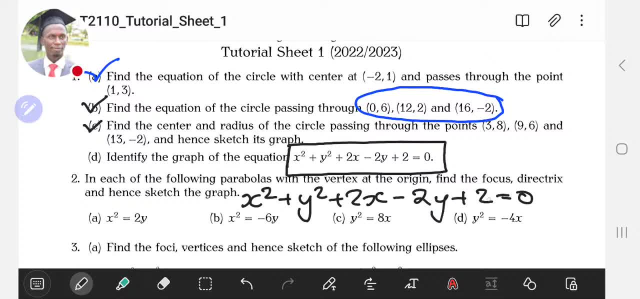 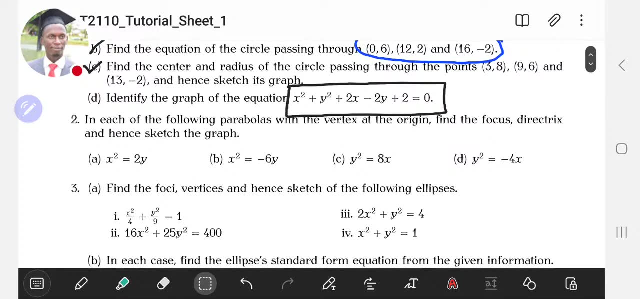 minus 2y plus 2 is equal to 0.. of course, to be able to identify completely, you will have to understand all the different conics that are available. you have to know the ellipse, the parabola, the hyperbola and, um yeah, the circle itself. so you have to know all those if you're 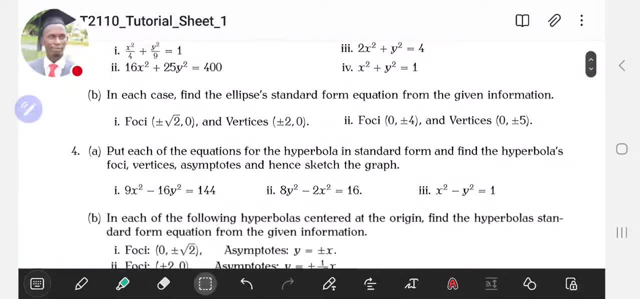 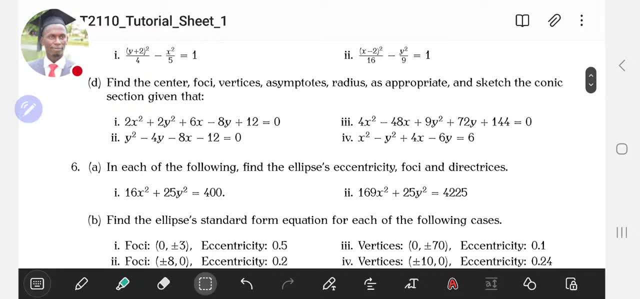 going to make, uh, if you're going to be able to identify a good question that you can use to practice, uh, if you can identify them, is going to be: uh, yeah, some. i think this was what. yeah, they actually said: sketch the conic, so this one here. actually, uh, d here. this is going to. 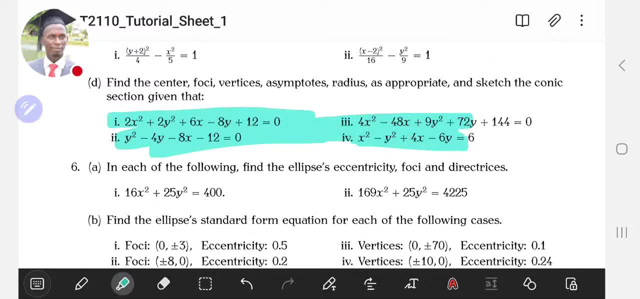 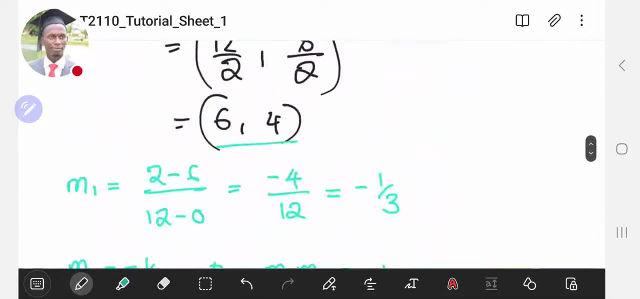 be a good one that you can use if you want to see how to identify them. it's going to be a good one, but of course we'll reach that if we have time to do that one. but let's see how you identify for this one. so the first step, of course, is going to be completing the square. 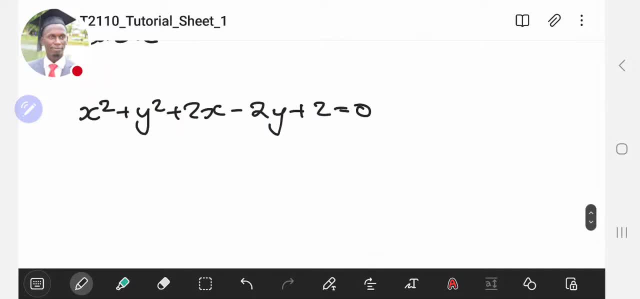 so you have this expression: you want to complete the square group, the terms with x group, the terms with y together. just write them one at a time. so i'm going to have x squared, i'll bring the term with an x here. so plus 2x, then you have plus that the next one is a y squared, y squared, then we're. 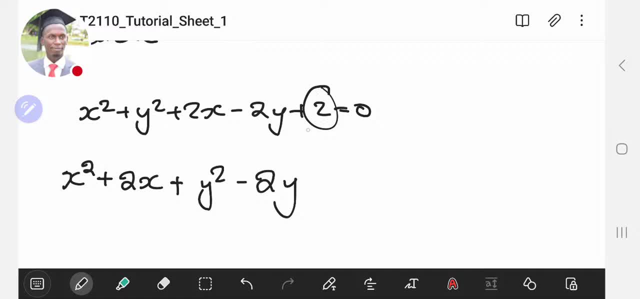 going to have minus 2y. now what you do with this tool, the one that doesn't have an x or a y, it's up to you. you can leave it here or you can already, at this stage, take it to the other side. now, how do you complete the square? first and foremost, you want to ensure that the coefficient 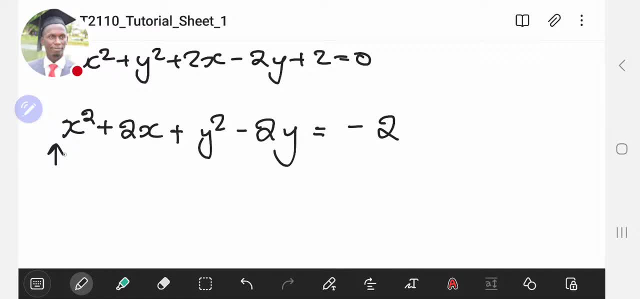 is a one here, not a negative one, a one. if it went a one here, i would factor it out, pull it out and see what remains, but in this case, of course it is. uh, it is a one already. so i think this is, um, this is a little bit straightforward. um, we just go right ahead to start looking at. 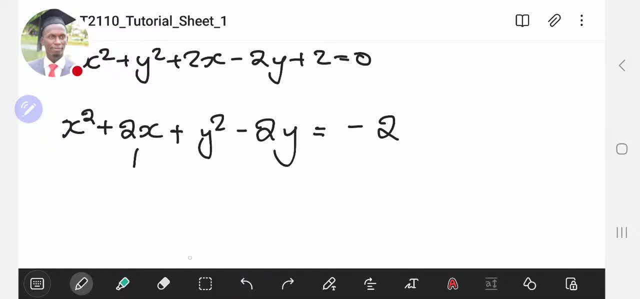 the coefficient of the x, the x term. so the coefficient of the x term here is just a 2. so this is x squared plus 2x. now i'm looking at the coefficient of the x term here. that's a two. so i'll add not just the two, but half of it. i'll divide it by two. after doing that, 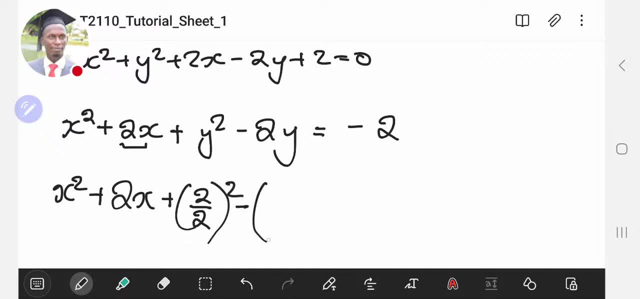 i'll square it, so i'll add it, then i'll subtract it. so again, i'm subtracting this and squared. notice that doing this ensures that what you're doing here is just adding a zero, because this is literally just a zero. we'll do the same thing to y here. 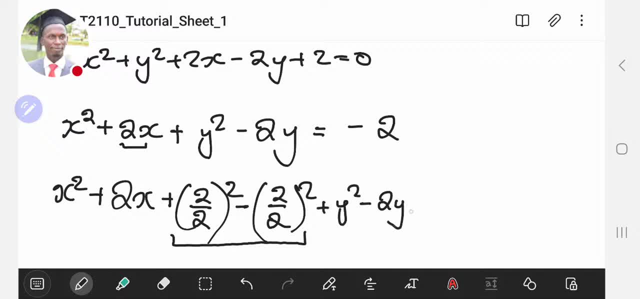 this is y squared minus 2y. so again at this point we'll do the same thing. we'll add half of the coefficient of x of y. this time the coefficient is minus 2.. half of it we divided by 2. so square it, add it, then subtract it. minus 2 over 2 squared is equals to the negative. 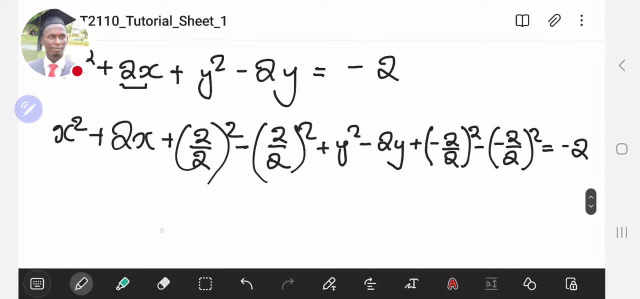 2, which was the other side. now, at this point, you can evaluate the second square. the one you're subtracting can evaluate it, but the one that you are adding don't evaluate this square root. you might lose something important. so, with that in mind, this expression, you have to know to say, this expression can reduce, just get. 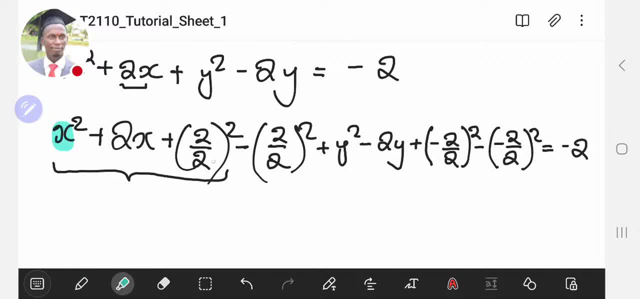 this x stem, the one that is square, just get the x- lose the square for now and then get this stem here in the brackets including its sign. so this stem in the brackets, including the sign, is just going to be positive 1.. so i'm going to end up with x here. i'm leaving the square for now. 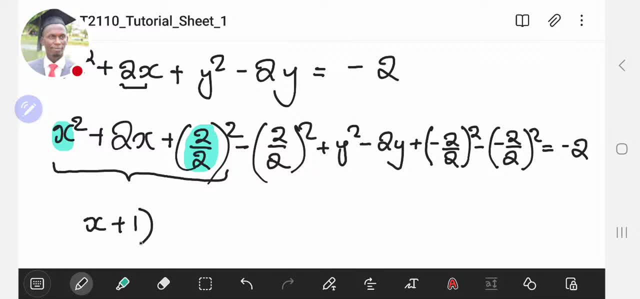 and then this is positive 1, so i'll write plus 1 here, then i'll get both of them and i'll square. what you have to know here is that if you try to expand this, it will actually give you the same answer as this expression here. the whole thing, yes, including the 2x on the middle. so even though 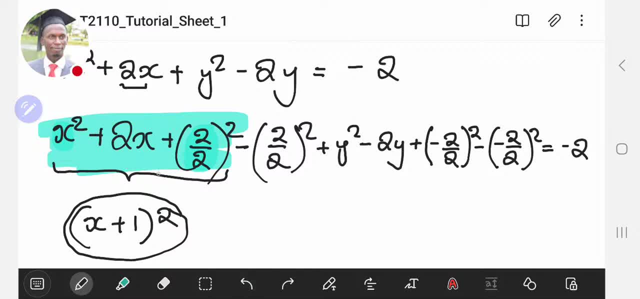 we've just written it shortly, like this: these are actually the same, so this is how it goes. for now i won't show that. we can still show it, but i won't, um, so just move on. so with this, we still have this, it's still there. that's two over two. remember this. i said you can evaluate. 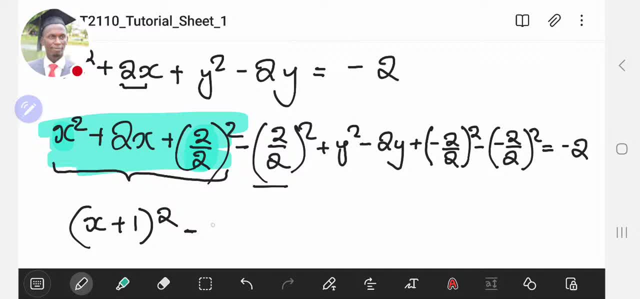 so this becomes minus two over two. that's a one one squared it's two one. so minus one plus. now we reach this part again. this will have a similar behavior. so we'll get the y here. the y is square, so just get the y there. that is going to be y, then we'll. 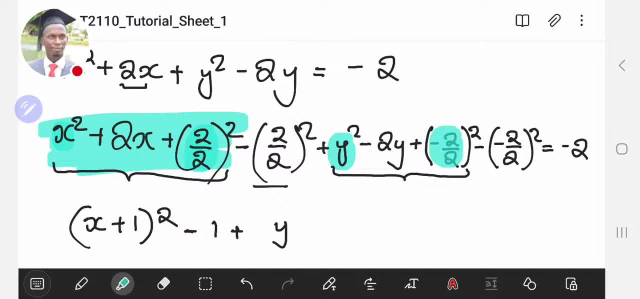 get the thing in the brackets here. this is negative. two over two, that's negative one again. don't evaluate that. uh, that square, that square. so just get minus, including the sign. that's going to be minus 1, then together i'll square them again. the argument is that this thing here 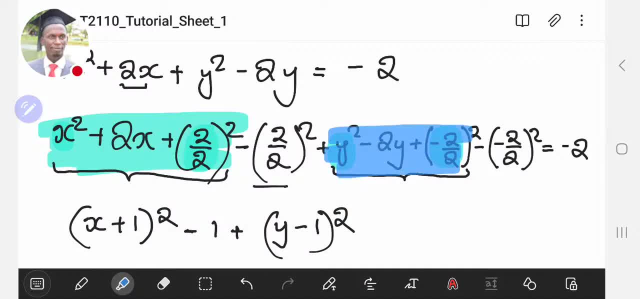 this thing. it will literally be the same as justice. so if you try to expand this, it will give you the same thing in blue there. so everything else there has to still be the same. that's minus negative 2 over 2, that's negative 1.. i can evaluate this. that becomes negative one squared. that's positive one, so this becomes minus one. this is the one squared. that's positive one, so that's 1 square, and so that's the plus k. if you reduce to that, the whole of that is equal to zero, so everything becomes minus one. this is the unsafe thing, which is because the average chance that the index won't be. 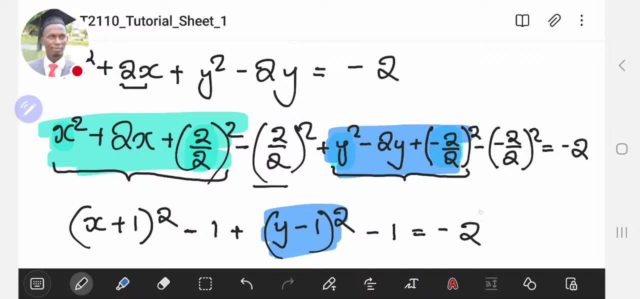 equal. i mean, i'm interests in the equation, so we ended on the time when we have the somehow as this and have the same. i mean, you have enough time. i'm interested in creating theicks which are just to get realized. this is the one that is equal to negative 2 from here. now we are almost done, just simplifying this. 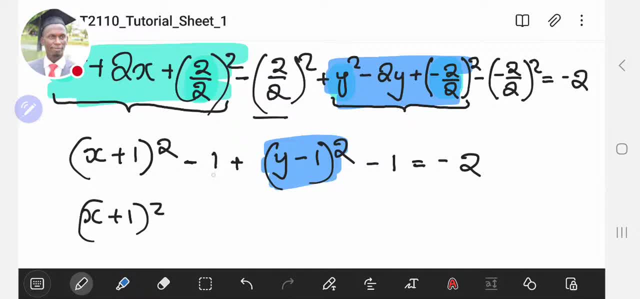 x plus 1 squared, then we have minus 1 and minus 1 that's minus 2. we'll take that to the other side. so this is y minus 1 squared equal to minus 2. then the minus 2 when it crosses, it becomes: 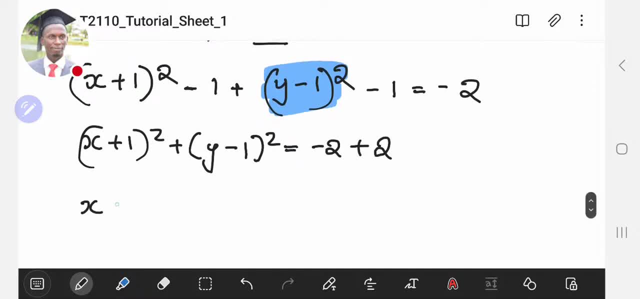 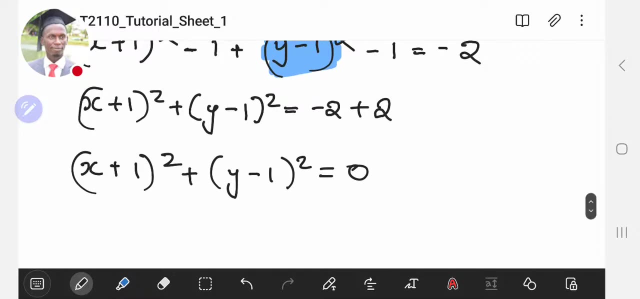 positive 2. so this is just a 0 x plus y plus 1, that is sorry, plus 1 squared. and then we have plus y minus 1 squared is equal to 0. now, when we look at this, this looks like a circle with the center, whose center is, remember the standard, that's x minus h squared plus y minus. 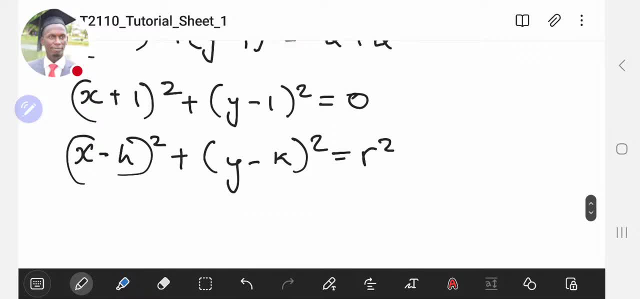 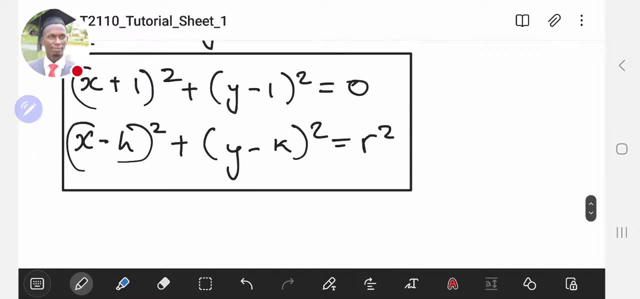 k squared equals to r squared. so if we compare the two expressions, what we have on top looks like a circle, but the only difference is that. well, first let's start with the center. the center of this expression on top it's- uh, it lies at negative 1 comma 1. this is where the, the center lies. so with with that in. 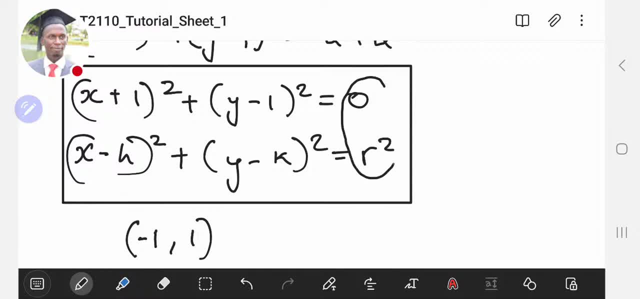 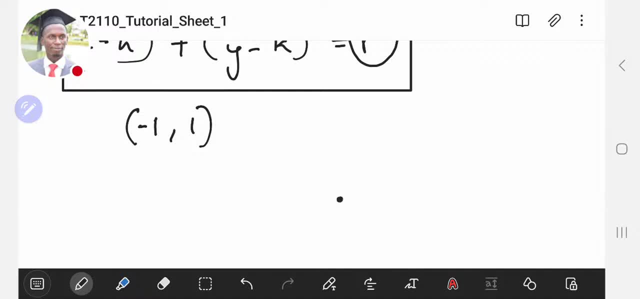 mind. how about this part? when you look at this part, you see it's like the radius is 0. so if you look at this part whose radius is 0, that just reduces to a single point, because the radius is how far the circumference is from the center. this is, uh, where the radius would be. but if the radius 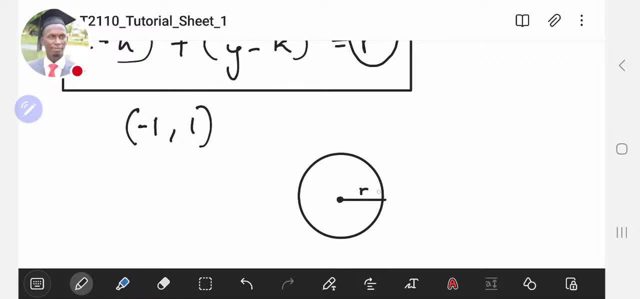 itself is a 0, then that is not necessarily a circle, it's just a point. so that question they were asking us to say identify, uh, what this graph is. well, it's just a point. that equation is an equation of a single point, so that sorts out this question. 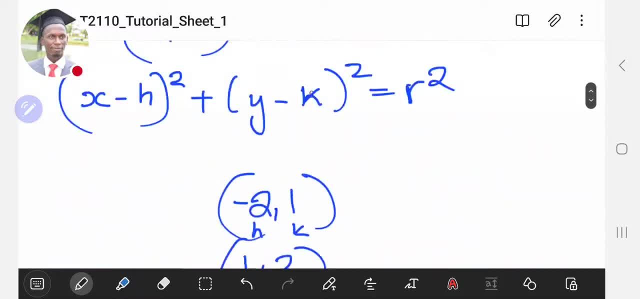 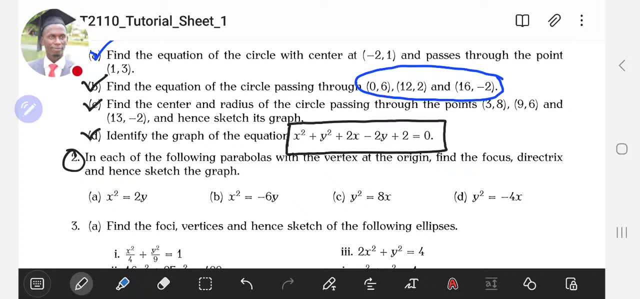 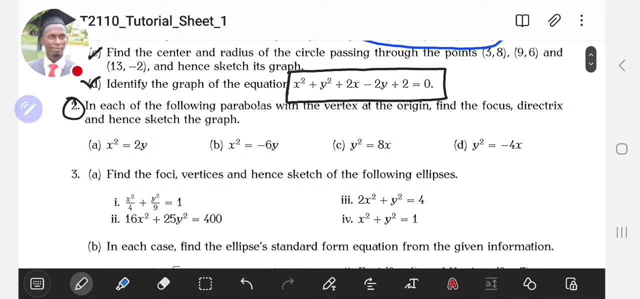 okay, so you can move on to the next part. so that sorts out. uh, this one as well. you can move on to number two. for number two, what is happening? well, now they're saying in each of the following: uh, they're telling us: now we're dealing. 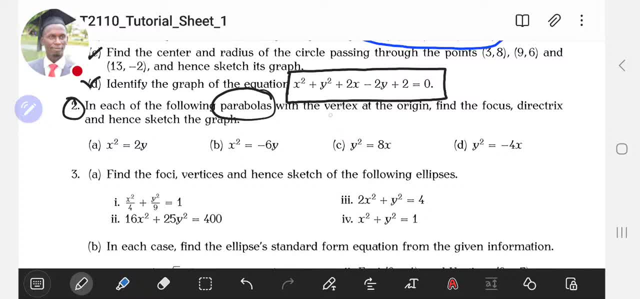 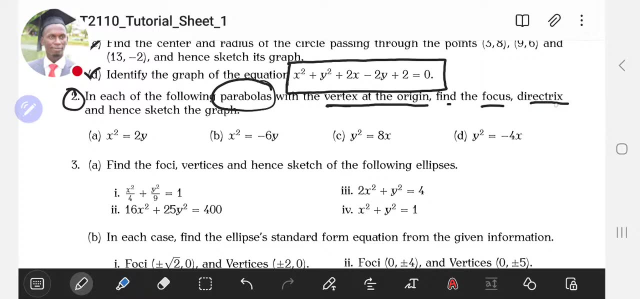 with a parabola, they're saying: they want us to get the vertex and then the origin. uh, this is at the origin, that's where the center is. so i say, with the vertex at the origin, no, okay, so here they're saying that the vertex is at the origin. then they want us to find the focus, the directrix. 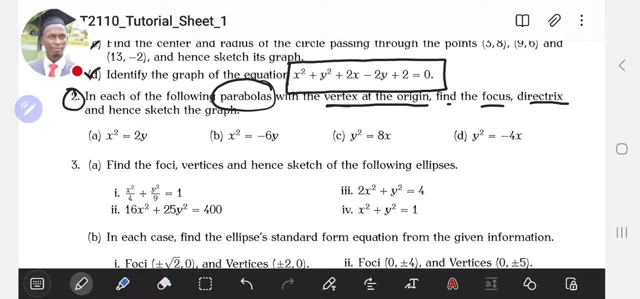 and hence they want us to sketch the graph. so how do we do that? well, it starts with us understanding how a parabola looks like. now a parabola, of course, is going to have an equation which looks a little bit like this: x squared is equals to 4 p, y. so this is how a parabola looks. 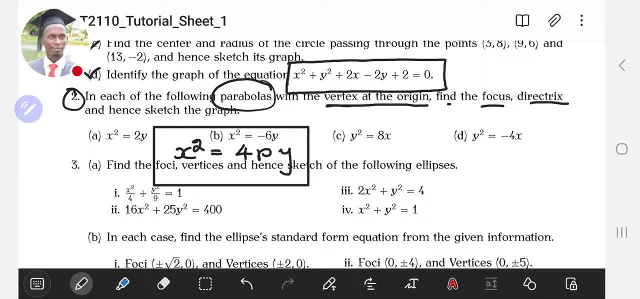 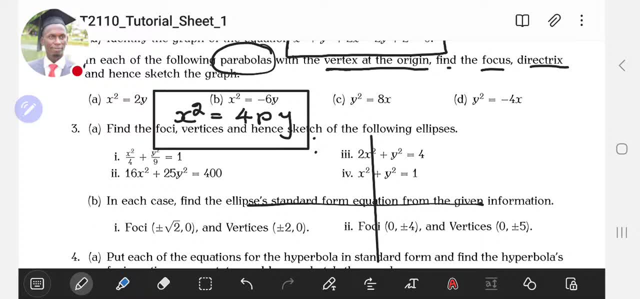 like now. of course, if you have it like this, then you not to say this parabola, it's one that opens upwards. so this parabola opens upwards. its vertex is at at the origin again and it opens upwards. if it were negative here, they know it opens downwards. 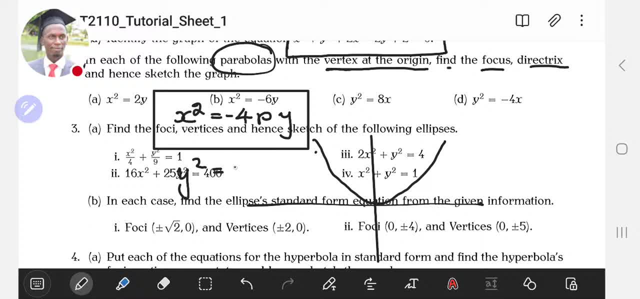 if y is the one that is squared, then now what you're seeing is that if y is the one that is squared, then you're still dealing with a, a parabola, But now it's not opening up or down, It's rather opening to the left or to the right. 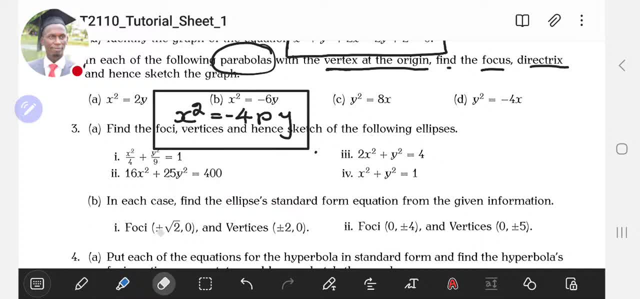 That is, if y is the one that is squared. So if you quickly observe the questions that you're given here, Here x is squared. You know this opens up or down, But because this is positive, you know it opens up. Then next, if you look at this one, this one, here it's x squared again. 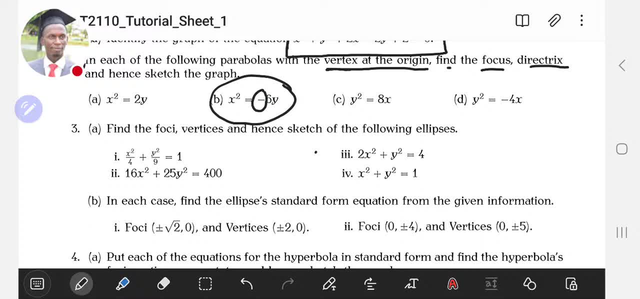 You know it opens up or down, But because you're seeing this negative here, you're sure it opens down. Then you move on to this one. This one y is the one squared. So you know it opens to the right or to the left. 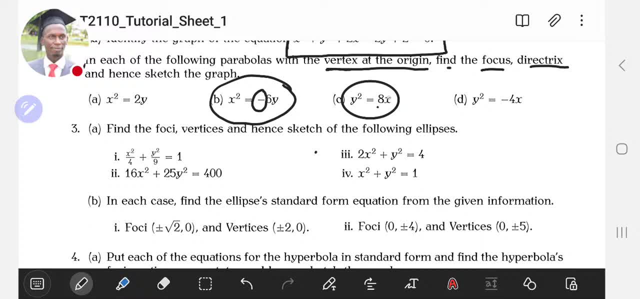 But this is positive, So you're sure it opens to the right. Then next, when you look at this, one y is squared. It's to the right or to the left. Because of this negative, it is to the left. So we've made those conclusions very quickly. 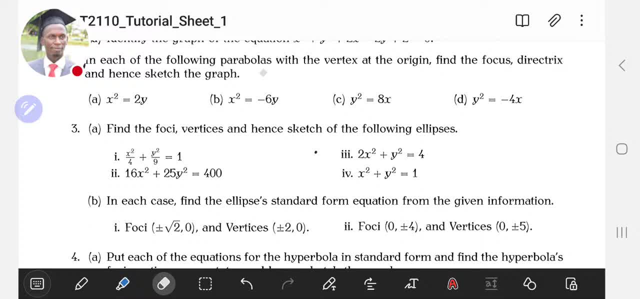 But let's see how do you actually work out this question. If you pick the first one, I'll pick one with an x squared and I'll pick one with a y squared. So if you get the first one here, x squared is equal to 2y. 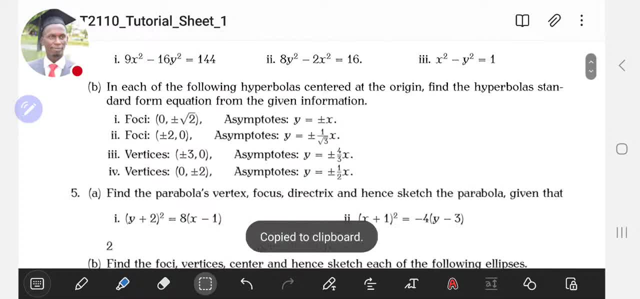 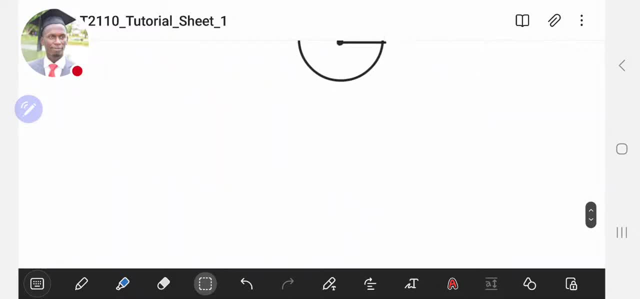 How do you work it out? Well, in this case, the first thing that you do there is: you have- Let's see that. So OK, Yeah, this is our equation. So all you have to do is compare it with what you expect. 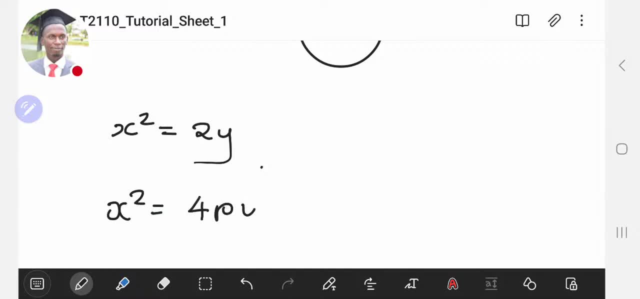 What you expect is x squared is equal to 4. And it is x squared. But what we don't know is you have to do it with the thirdまた by 4p, Right? So Nu4 needs a doubleundermezeh squared over Pi. 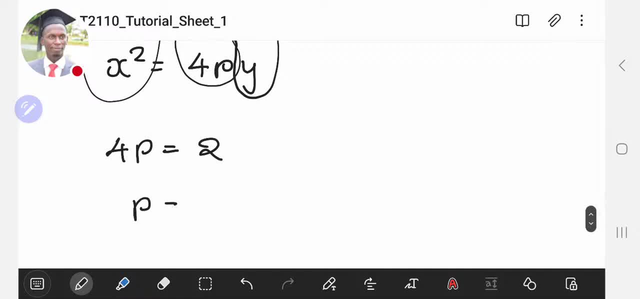 So this is the same. The y here is the same. Then the 2 has to be the same as the 4P, So 4P has to be the same as 2.. From here we end up with: P is equal to 2 over 4.. 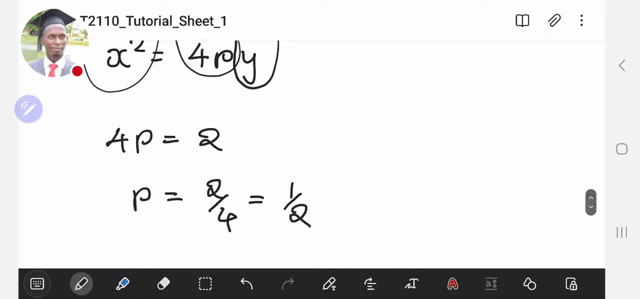 So that P is equal to 1 over 2.. Once we have this figured out, well, there is becomes a little bit straightforward. far, we have to move from the origin to where the focus of this, this parabola, is. so since this, we notice it opens upwards. so I'm going to have our parabola, okay. 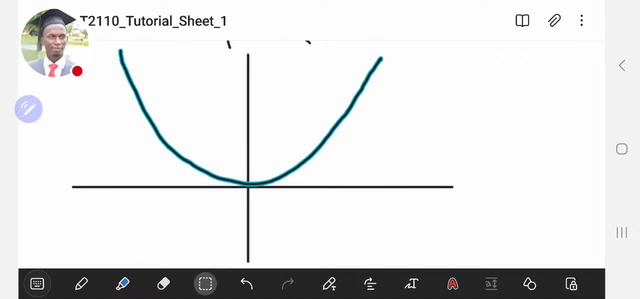 so this, something like this, I just bring it down so that it of it, the origin, the centers at the origin. so this point here, where the focus is going to be this is the distance from where the vertex is to where this is. this is the value of P, so 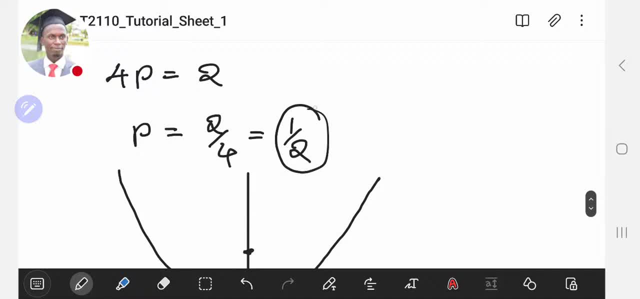 from our calculation here, we've just seen that P is actually 1 over 2. so from here going to where the focus is, this has to be 1 over 2. the question was asking us to get the position, the coordinates of the of the focus for this. 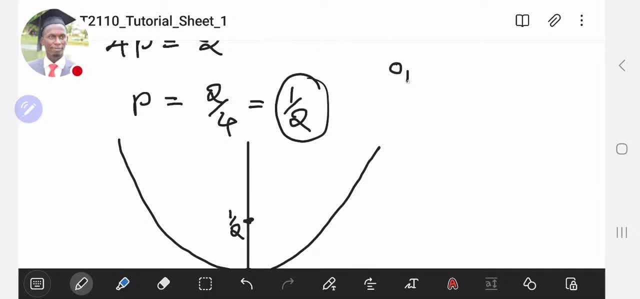 for this parabola. so this is at 0 comma, 1 over 2. this is where the the focus for this, this, this conic, is. but how about the directrix? because we're not to say for a parabola, we have to specify where, if of course it's at the origin, I have to. 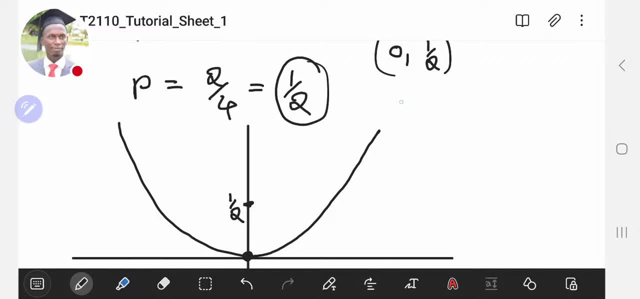 specify where the focus is and also where the directrix is. well, in this case, the distance from- for a parabola, the distance from the vertex to where the focus is is going to be the same as from the same vertex, but going the other direction, to where the directrix is going to be. so if you had to go, 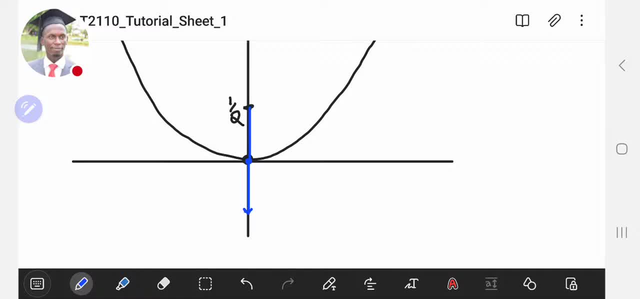 half units up, it will mean that you have to go half units down, so this is going to be at negative 1 over 2. so in other words, if you are to draw the directrix, it will have to be a line that stretches horizontal, passing at negative. 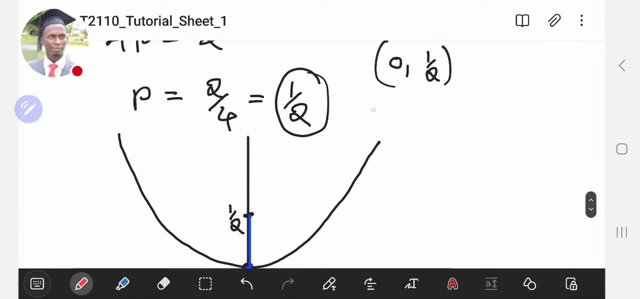 1 over 2. so if wanted to state it, we can say that the directrix is going to be a line which is defined by y is equal to negative 1 over 2. so we have specified a line related to negative 1. we didn't select a line which is upon the 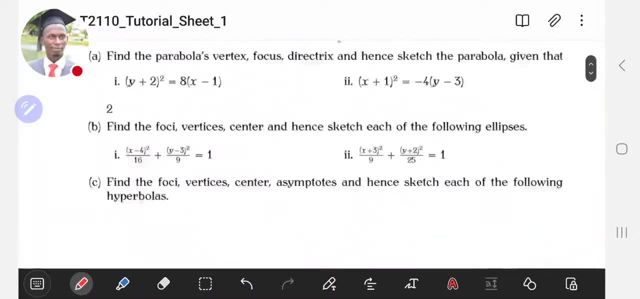 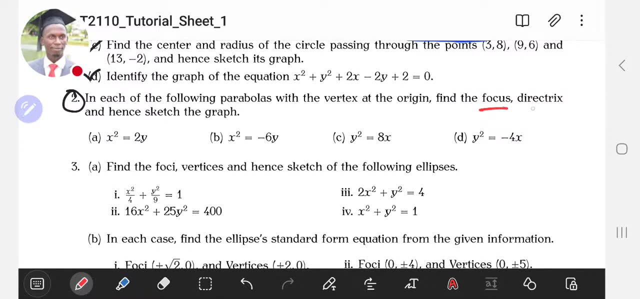 share and we can call this would be negative 1 over 2. so you can between the seemed Ax's and I'm going to choose negative and the finish line is negative, so that you know. so you can simply fill all the find by this shape of the. 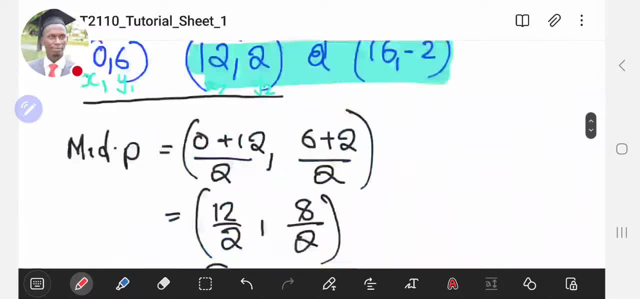 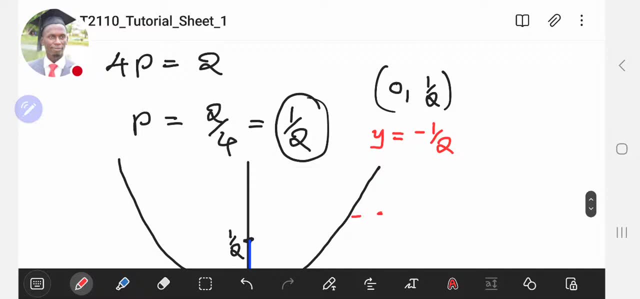 increase. and you can also, instead of as per the distance between the two dominance, you use a derivative source so that you can write it at negative 1 over 2 into negative 2, or you can change it to make y the subject of the formula. it's still okay, so this sorts out. 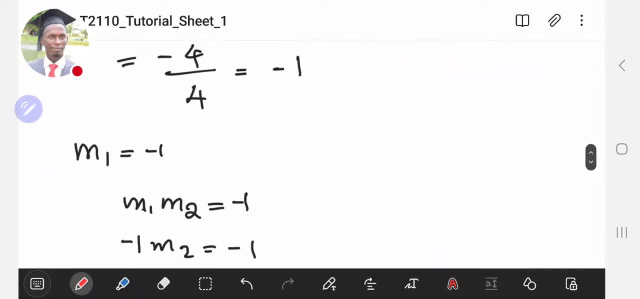 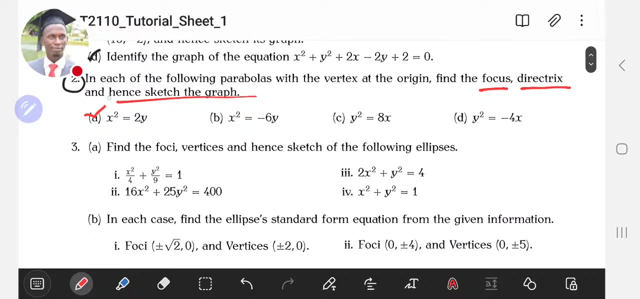 the first one, so i'm going to pick one of them here. we can pick any one, really, okay. so i'm going to pick one equation, one question again, so let's see the one that we can get. so we've just done this one, so we can do one where y is squared. let's do with a negative. 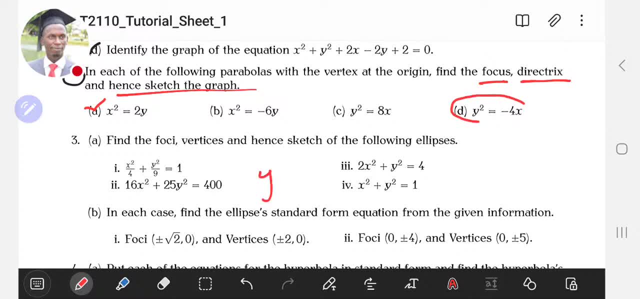 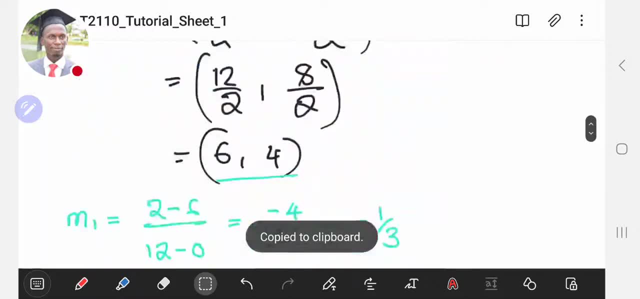 now. so let's do d, so let's do this one. the one is: y squared is equals to minus 4x. so in this case, now let's see how we approach that one. so it's the same thing, but now, because y is the one squared, we know to say things are a little bit different, because now it opens either. 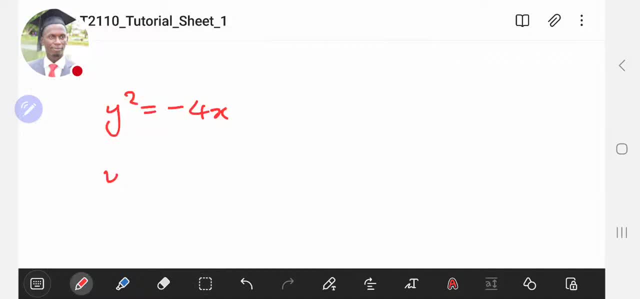 to the right or to the left. so we know to say this: one has to be y. squared is equals to minus 4px, so p is equals to minus 1. you'll get confused by what the minus actually implies here. well, you can just treat it as if it were a positive, so that it just tells you how many. 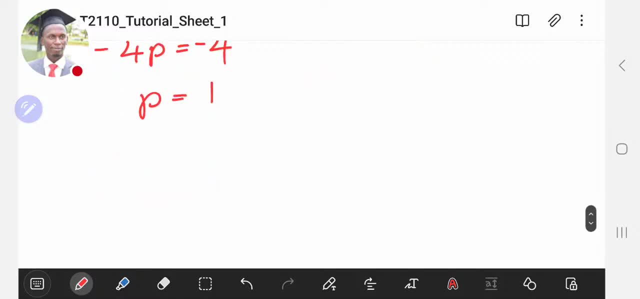 units you have to move. you know to say: being negative, it opens to the left, since this here, y is the one that is squared. so if i was going to sketch this, what we have is this: we know it opens to the left. the vertex is at the origin, so we still have this. 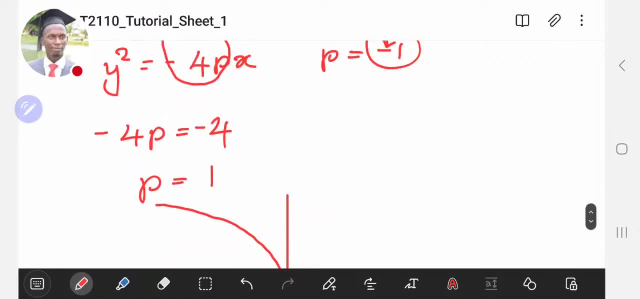 opening to the left, what the p tells us, whether it was negative, or what the value there just tells us to say that we are going to the left. we're going, we have to move one unit, but since it opens to the left, that one unit has to be a step going to the left. so you can even conclude that that negative actually tells you. 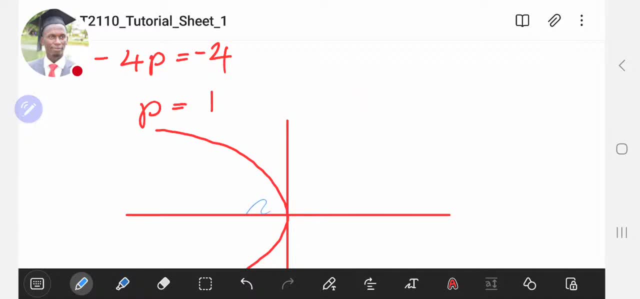 to say that you're going in the negative direction. so here it implies that we have to move one unit. this is going to be at negative one, so if you wanted to get the coordinates of the focus, it's going to be at negative one comma zero. this is where the focus is. then the other thing that we need is the directrix. so where is it you? 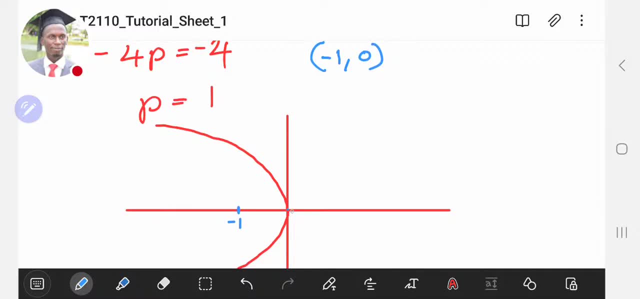 know to say: if you moved one unit to the left, then the directrix is going to be one unit the other direction. so it's going to be one unit, this direction, that is just going to be positive one, so that in the end the directrix is going to be a line that stretches in this manner. 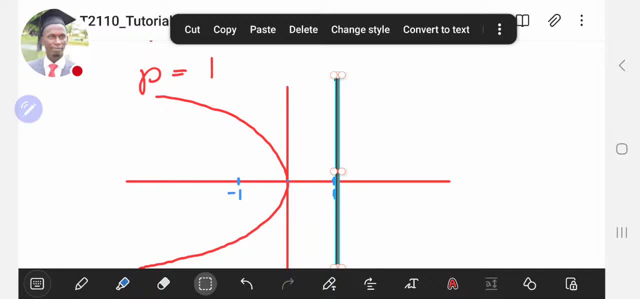 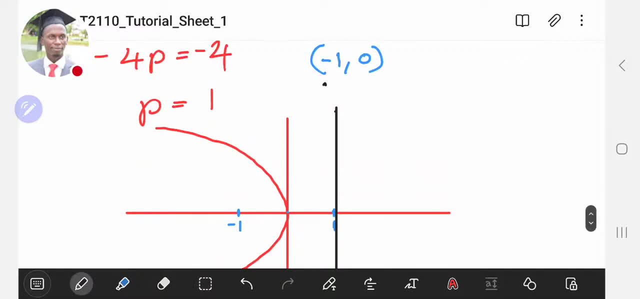 and goes something like that. you can move it around so that it is exactly at at one. so if wanted to state it now as an answer, our directrix is y. a line y is equals to positive one. then we are done with this one as well. okay, with this one done, we can then look at what comes next. 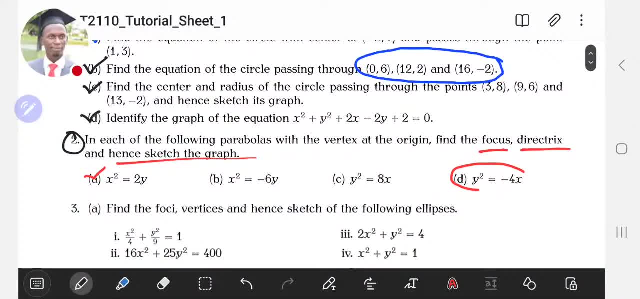 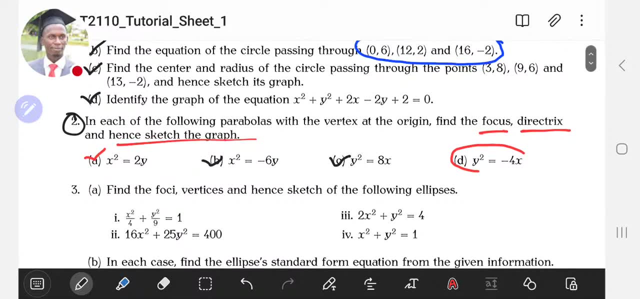 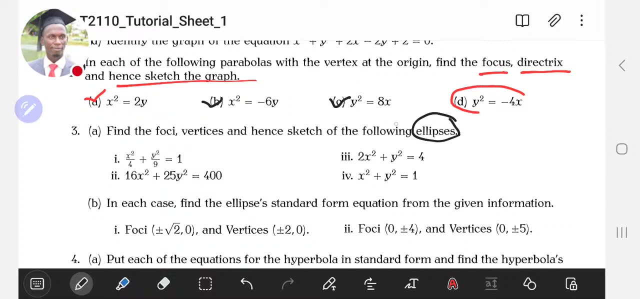 so that sorts out question two as well. the same way we did a and d, you can use that method to work out b and also to work out c. so let's move on to question three. for question three now, this is um. this is an ellipse again. it's all you understanding or knowing how an 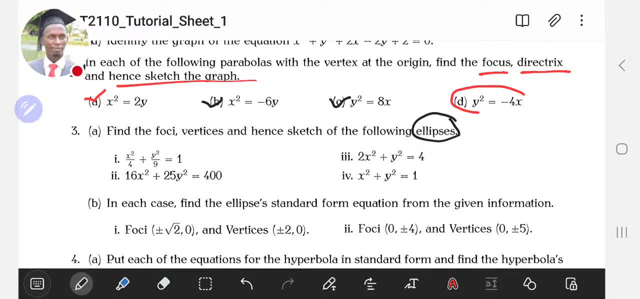 ellipse looks like. so how does an ellipse look? look like. well for an ellipse. what you have is x squared over a squared, plus y squared over b squared is equal to one. now i want to. i want to point out here: the next one that we're going to look at is the directrix. so we're going to look. 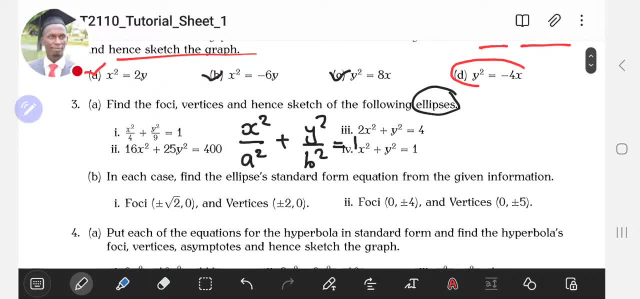 at is going to be the hyperbola. the difference between an ellipse and the hyperbola is a negative one of these terms for a hyperbola is going to be negative, depending on the behavior of the hyperbola it might be. this is the one that is negative or the one that is negative, but for 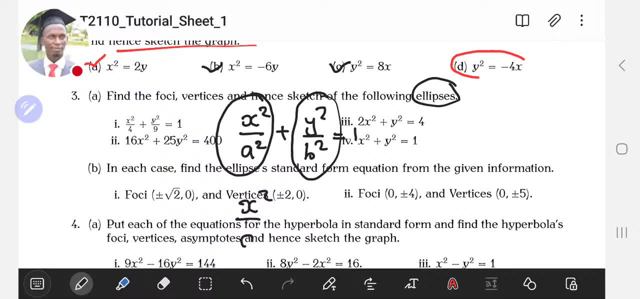 simplicity, you can still go to say: a hyperbola is going to have a negative right on the middle here. so this is the difference between an ellipse and a hyperbola. so i think that is the easiest way to remember them. uh, they're literally the same expression, except the negative which is here. so we'll see. 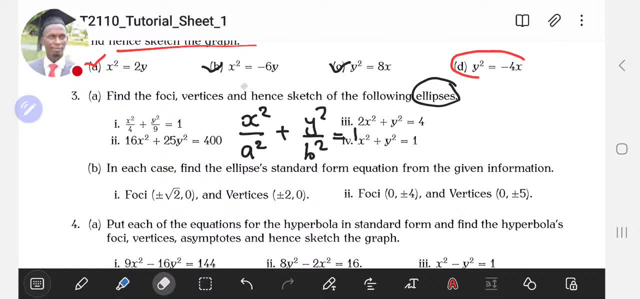 the hyperbola when we reach it, if we will, but for now, let's focus on the ellipse. so this is how an ellipse looks like. of course, we know to say here, a represents, uh, the vertex, and if you want to talk about the vertex, so if you just want to understand it very quickly, the vertex, when you hear the. 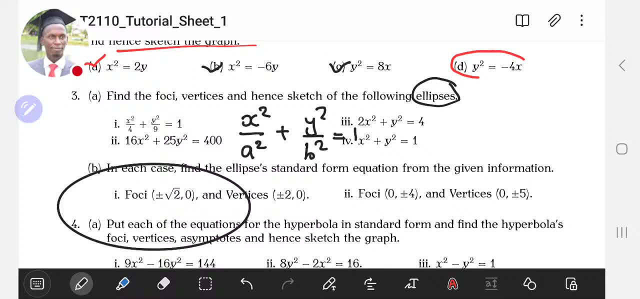 vertex. think about where it is actually curving or where it is actually turning. in this case, the vertex is going to be represented by the vertex and the vertex is going to be represented by the vertex. so that is what is going to be the vertex for the most part, and then the other thing that 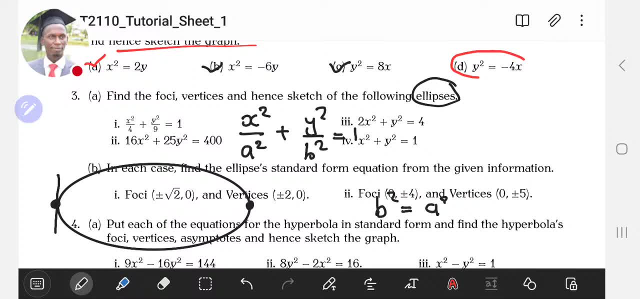 you have to keep in mind is that b squared is going to be equal to a squared minus c squared, where c is the focus. so with that in mind, let's see how we actually have to work out this question for the ellipse. so the first thing that you want to get is: let's just take down. 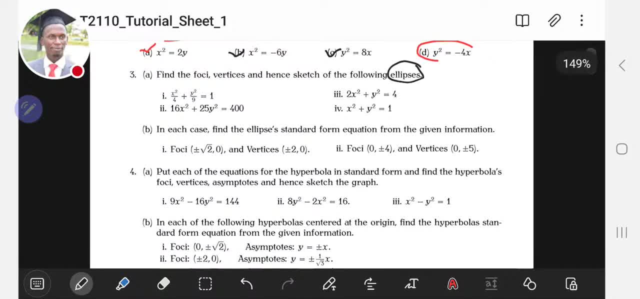 the questions that we have here. so let's start with the question: what is the vertex and what is the vertex here? so the first one, let's see the first one. we're just going to do uh, two here as well, so i can do this one here and i can do this one here. the other ones, um, can be worked out using. 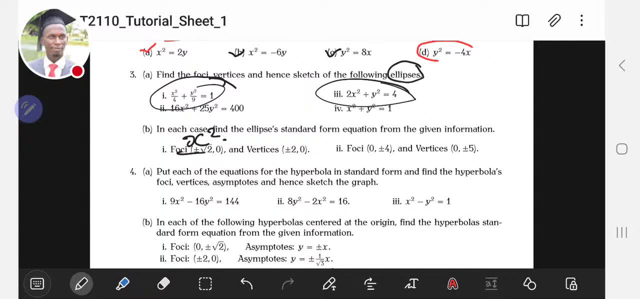 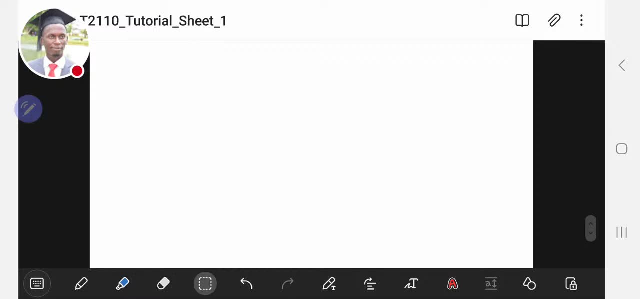 the same approach. so you have x squared um- this is over four, plus y squared over nine, this is equal to one. so how do you actually work out this question? so let's get it here. so well for this one here. what you have to just keep in mind here is that the value of a and the 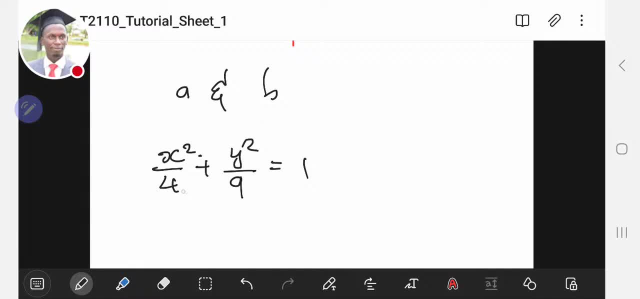 value of b. it actually depends on which one is bigger. if you have an ellipse that behaves something like this, then it implies that your a is actually in the horizontal axis, because your a has to be from here to here. so it only makes sense that a has to be greater than b because b 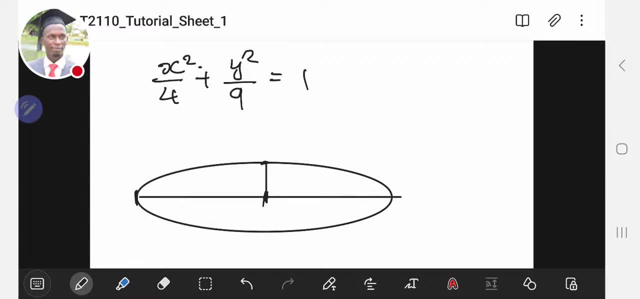 has to be a short distance from the center to just where this part is. so if you have two shapes- one shape like that, one in another shape that looks like this one here, for this one now, notice that your a is now this one, because a is obviously the one that is bigger than b. now, this is going to be. 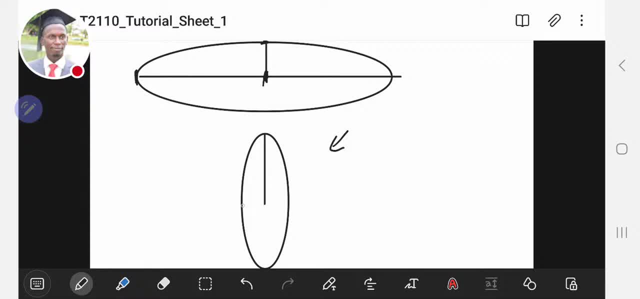 the part that is bigger than b, and your b will have to be in the x-axis now, which is smaller like that. so this is now how it's going to be. this is where your b is going to be. so what you do when you're dealing with this part- one thing i always tell those i teach math: 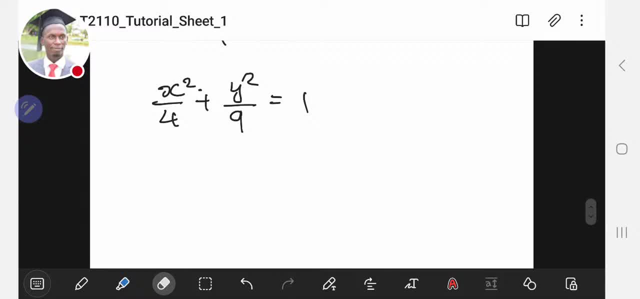 is that when you reach this part, the figure that becomes your a is going to be the big one. so compare these denominators. which one is bigger? of course, the first step is to ensure that this one on the right side, this is a one. once you've ensured that, now look at the two values. what 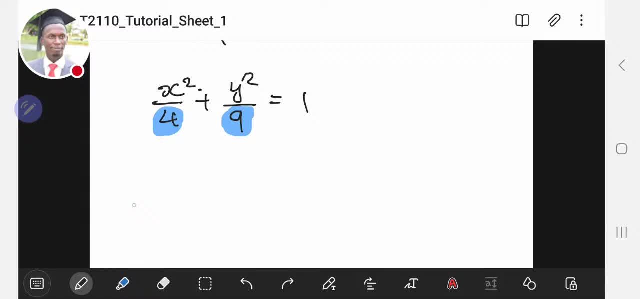 you want is the bigger one of the two. assign it to be your a. in this case, the bigger one is in the y axis. so let a square a squared. a squared is the one that is going to be equal to nine. what this tells you is that a squared, since it is with the y, with the y term, so we can conclude that this is. 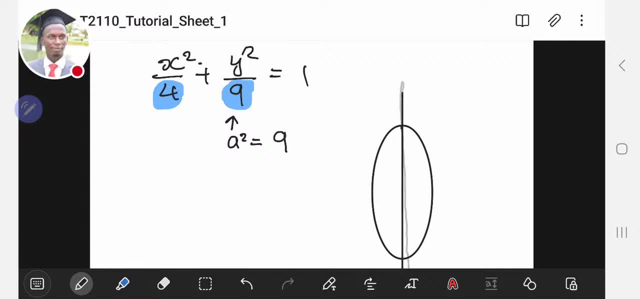 a conic section that is actually whose major is in the y axis. so you can say it's a conic section that looks something like this one, so that the big one, if that is, if the y squared denominator- is actually the one that is bigger than. 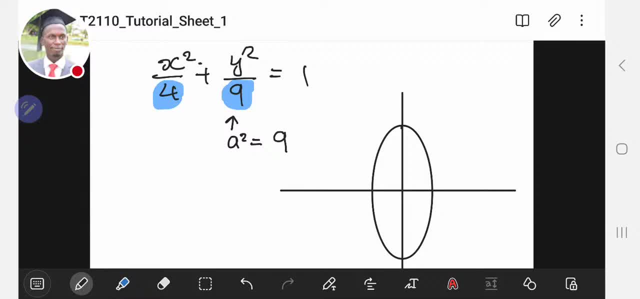 x squared denominator. once you've identified that, it's easy to find your a squared is nine, so that a is actually just plus or minus by square routine: plus or minus three. so this now tells you to say that the top part, the vertex that is actually going to be at three, and the bottom part here, 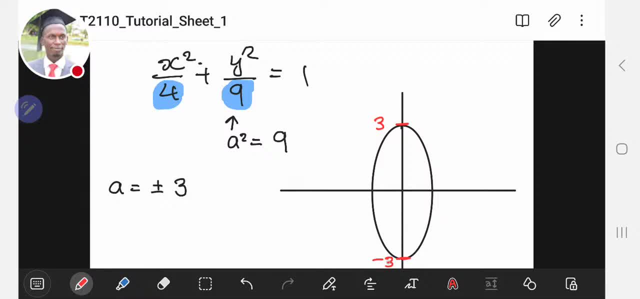 is going to be at minus three. so if they wanted you to state these coordinates so you can say that your vertex is going to be at plus, that's actually zero in the x-axis. this is from the origin. that's zero, comma, plus or minus three. so this is the vertex. 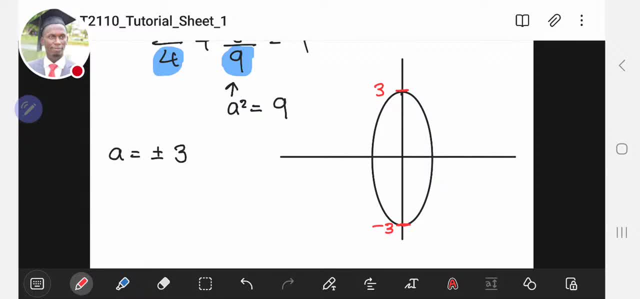 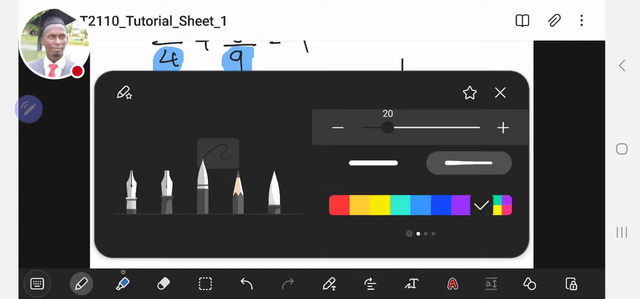 from the value of a. the next thing that we need is from the value of b. we know b squared is equals to four. so we have: b squared is equals to four. so from here we can conclude that b is equals to plus or minus two by square rating again, so that this here, this here, is a two and this one here. 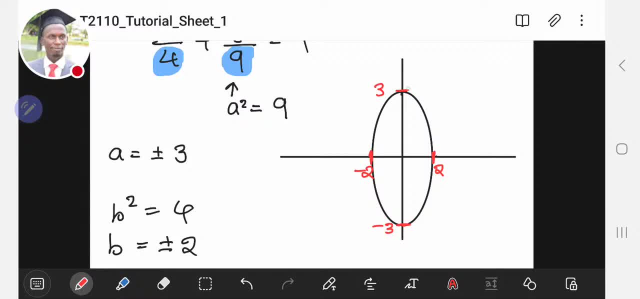 is a minus two, which makes sense. it's longer in the y-axis, so the value here has to be bigger than the value here, so this actually makes sense. so, with that done, the only other thing that we're left with here is the position of the focus. so how do we find that one? well, the relationship. 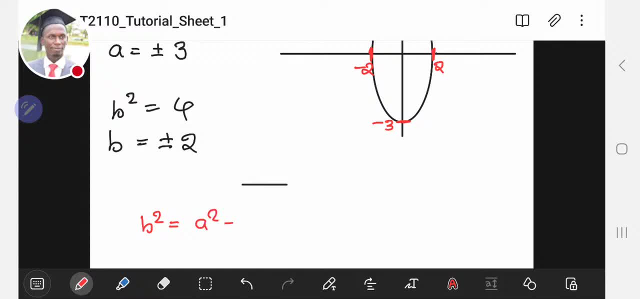 comes in. you know that b squared is equals to a squared minus c squared. the foci is given by the value of c. so how do we find it? so from here we can easily make c the subject or substitute. b squared is four, so you have four. 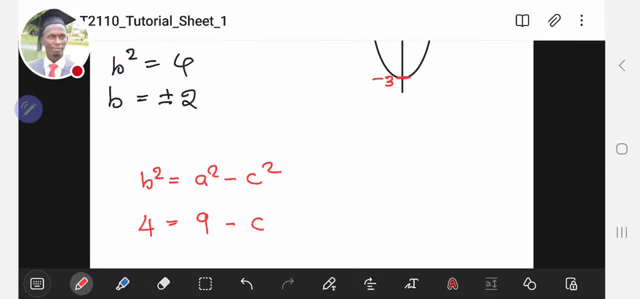 here a squared is nine. so you have nine here minus c squared. from here the c squared can cross, becomes positive. here the four becomes negative. so minus four, so that we end up with c, is equals to the square root of nine minus four, which is just the square root of the square root of five, but of. 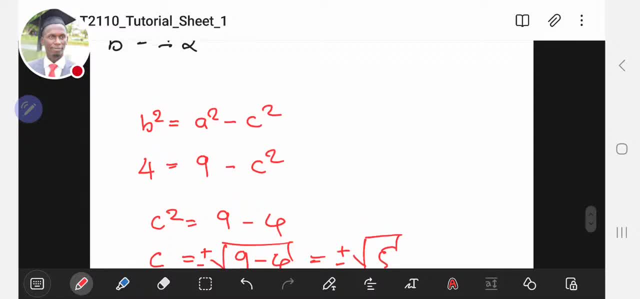 course, this is positive or negative, positive or negative. so we conclude that the focus is going to be somewhere here, the positive one, we can just place it somewhere here, positive root five, and the other one is going to be somewhere here, negative root five. so this is how you deal with this one. 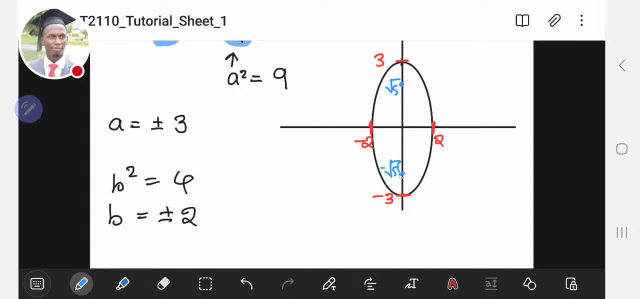 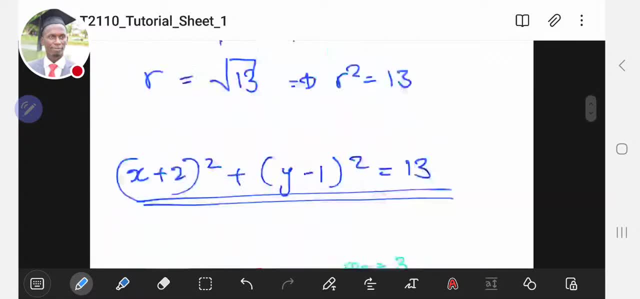 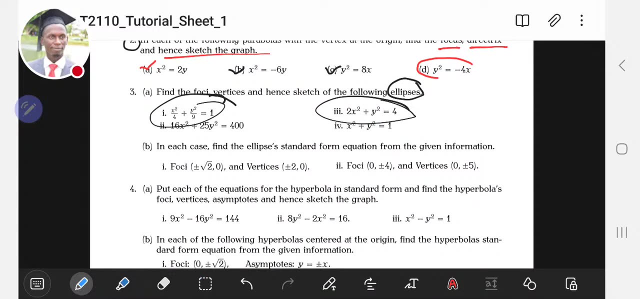 now, this answers this question. we've even sketched it. then you can move on to the next one. okay, so for the next part, for the next question, uh, I said we're going to do, we're going to do this one. I'm thinking we do just part two. but 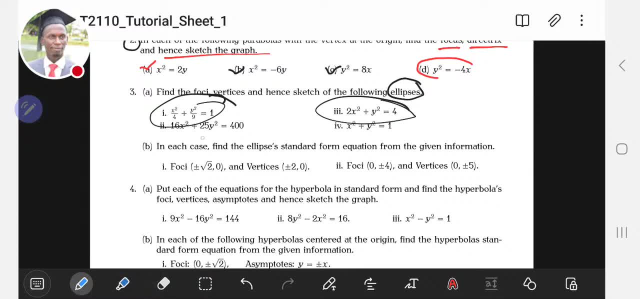 it's okay, that's the same one. I'm thinking it's going to be the same behavior. at least this one is going to behave a little bit differently. let's do this, let's do part two. so part two: this is now 16 x squared plus 25 y squared is equals to 400.. 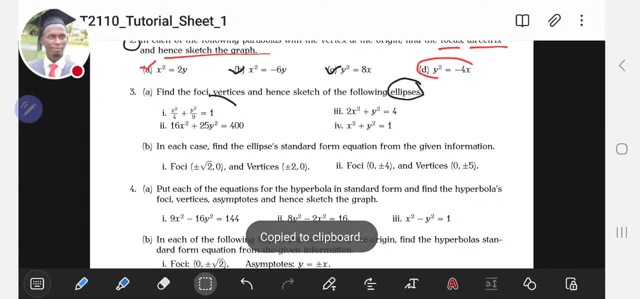 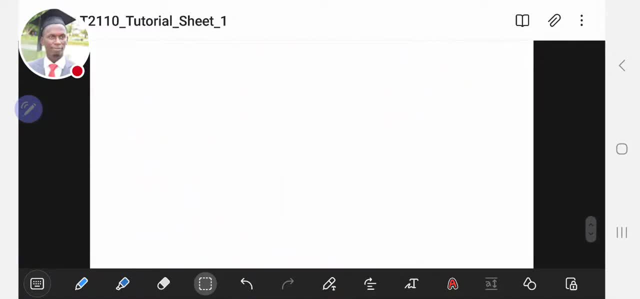 so we're trying to do the same thing: the vertex, the foci, and then you also want to sketch it right. so I'm going to say X square power, sh c, and we're going to stress that, but then I'll just hide the object. so I mean we're gonna do 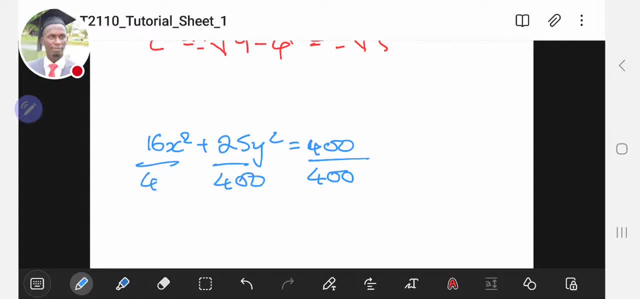 the same. so we're going to dove the output point to where provision center is. really just looking at the denominator and multiplying by, if you will. ch turned into adjoining device, 16 goes once there, but into 416 goes um. is it 25 times? yeah, you can try to do it uh slowly if you. 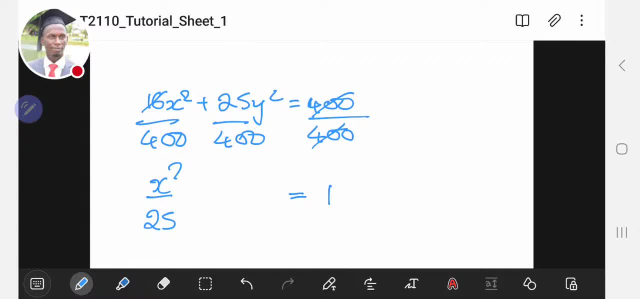 don't know what, what it actually gives you all together, you can still uh do it using using two. let me just do it very quickly here. that's uh 400 divided by of course you don't have a calculator. if you don't have a calculator, you can just do it in stepwise. but trying to save time, let me do it. 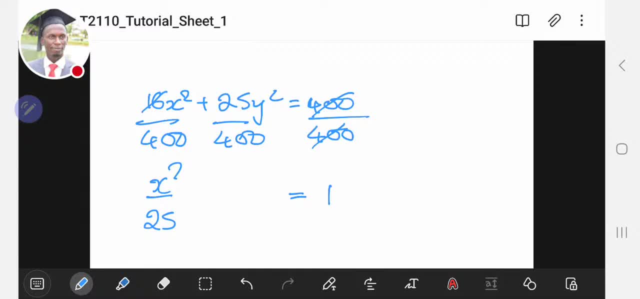 very quickly somewhere else. yeah, that's 25, so this is plus. then you have 25 into 400. so if 16 goes 25 times into 400, it only makes sense that 25 will go 16 times as well. so this has to be 16 here. 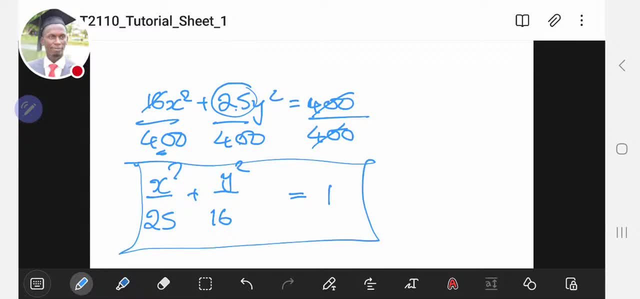 so this is how this simplifies. so we end up with this expression. so this expression- now we have x squared over 25 plus y squared over 16, is equals to 1. again that trick that i told you. you want to know how it behaves? just look at the terms. which term is it the x term or the y term? which term actually has? 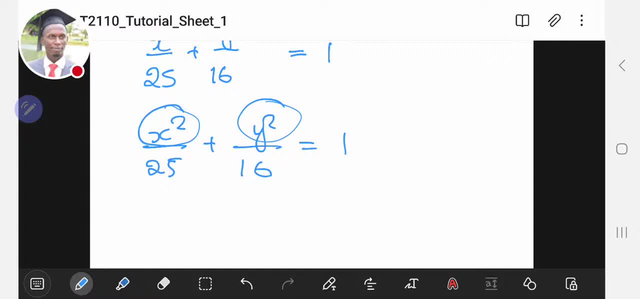 a bigger number in terms of the denominators. you see that x is the one that has a bigger number in the denominator. because of that you know to say your ellipse actually has a major in the x-axis. so you know that your ellipse is going to have a major in the x-axis. 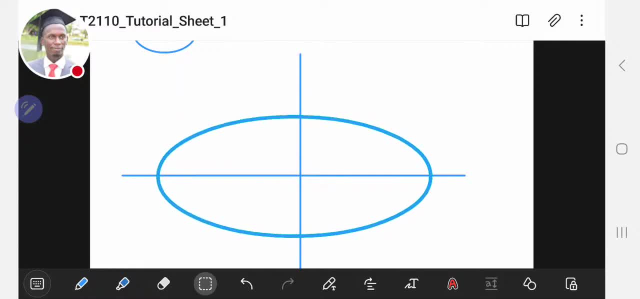 so again, i hope you you got how i deduced that. just look at which one is bigger, which one has a bigger denominator. if x has a bigger value, then the major is in the in the x-axis. if y is the one with a bigger value, then the major is in the y-axis. this only works for the ellipse, don't. 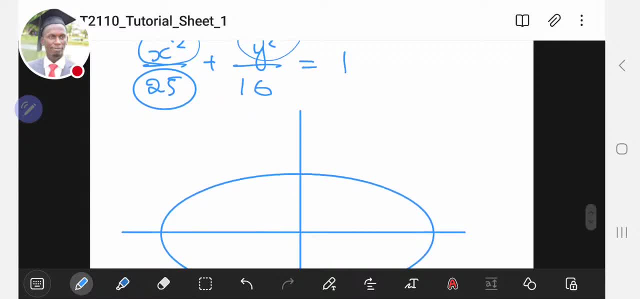 use it in the for the hyperbola, okay. so with that done, we're not going to say the bigger value has to be your, a squared. so a squared is 25, so that a is going to be plus or minus the square root of 25, which is just 5.. so with that done, already we can conclude. 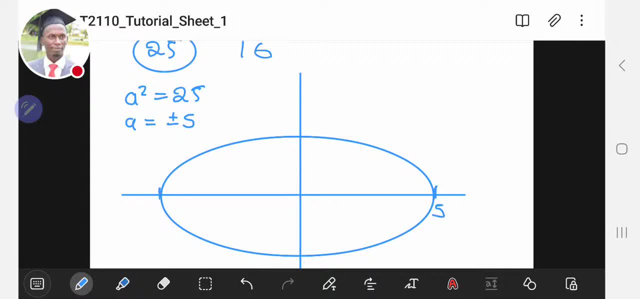 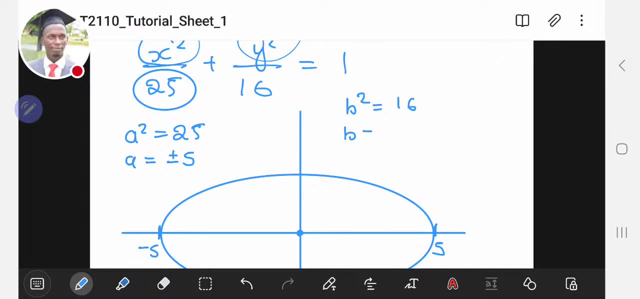 that. this is the positive part, that is going to be the 5. this is the negative part, this is going to be the negative 5.. the center is at the origin. then next, b tells us where the, the y, intercepts, will be in this case. so b squared is equals to 16, so that b 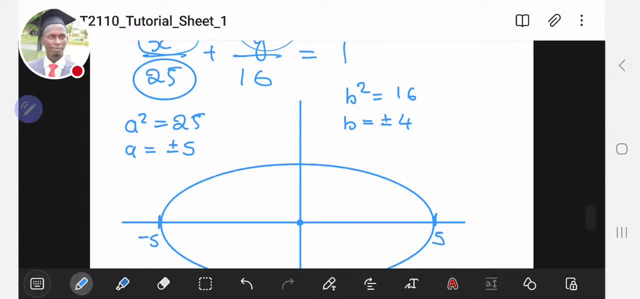 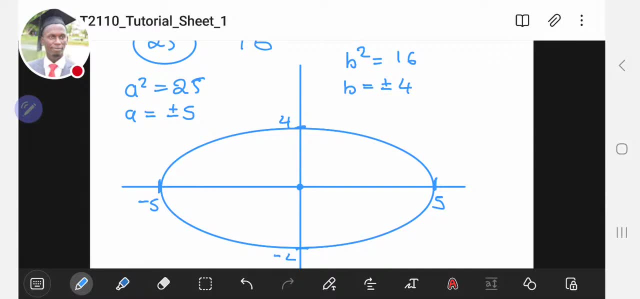 will be equal to plus or minus 4, again by square rooting. so here again we know to say the top part is a 4 and the bottom part is a minus 4.. so this sorts out the um, the vertices. the next thing that is left now is just the foci. how do we get it? well, again, the relationship. it's an ellipse, so b squared. 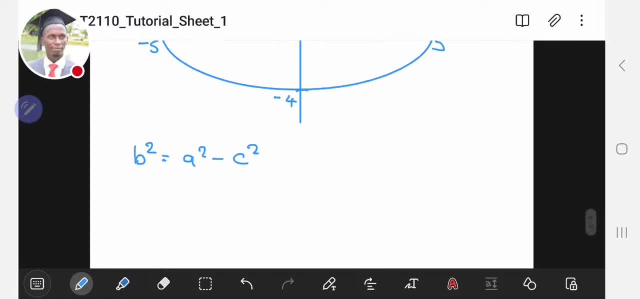 is equals to a squared minus c squared. from here our b squared, we found b squared was 16.. so you have 16.. a squared was 25 minus c. squared again, c squared crosses becomes positive 25 minus 16.. this is going to give us 9 and then we square root 9. this is going to be plus or minus. 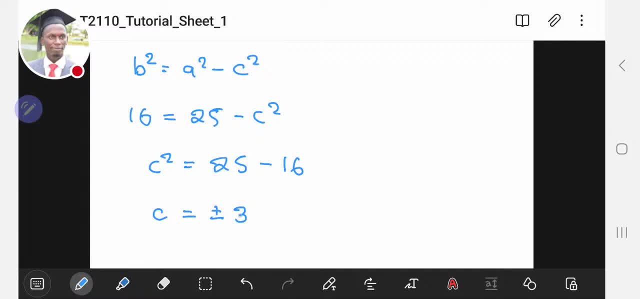 3, square root of 9 is going to give us 3.. so with this found, we now know where the foci is. so this part is going to be the, the negative part minus 3. this part is going to be the positive part, positive 3.. so we can make a conclusion now: the foci is going to be at it's in the x-axis. 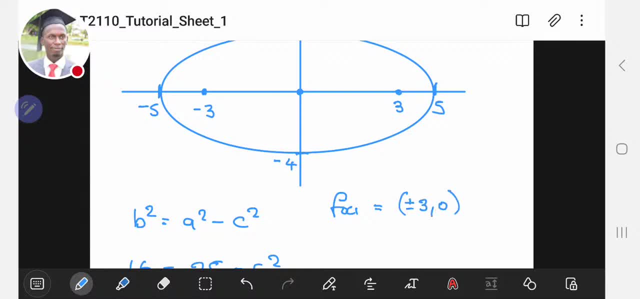 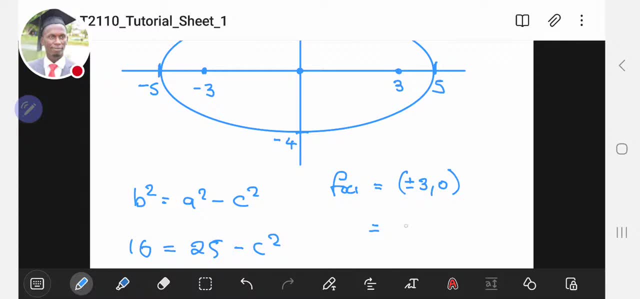 so we're going to say plus or minus 3 comma 0, and then you can even go to the vertex. the vertex is going to be at um. this is again that's in the x-axis. so it's going to be plus or minus 5. 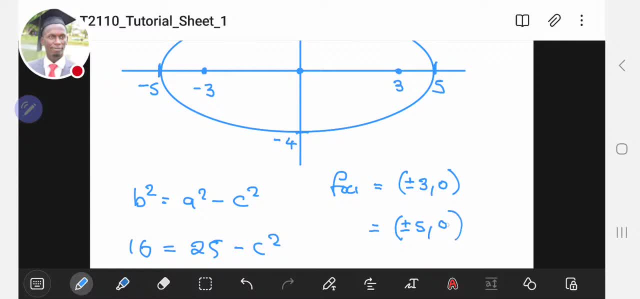 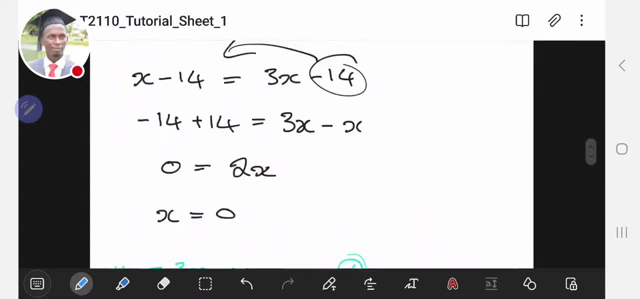 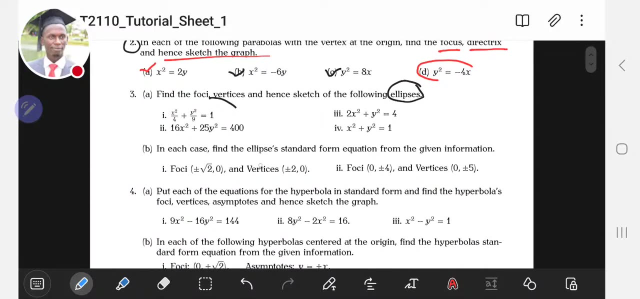 comma 0. so this answers this question and we have also sketched it okay. so this answers question. this was question. what was it? question three? so this answers question three. uh, leaving us only with uh, with part b. so we're done with this part. now we're only moving to b for b, we're just going to do one of these. b is quite straightforward. 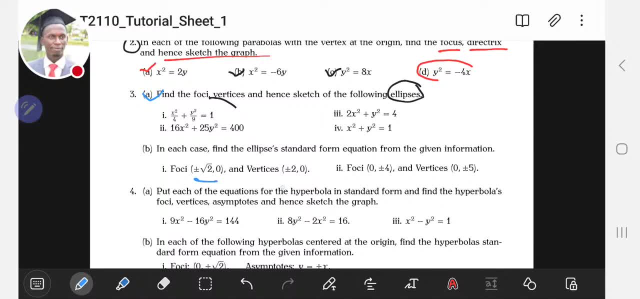 uh, here, of course, they're giving us, uh, what the foci is and also what the the vertices are. just observe where they're giving this foci: the foci is an x-coordinate. even the vertices here, when you look at them, this is an x-coordinate. so you are. 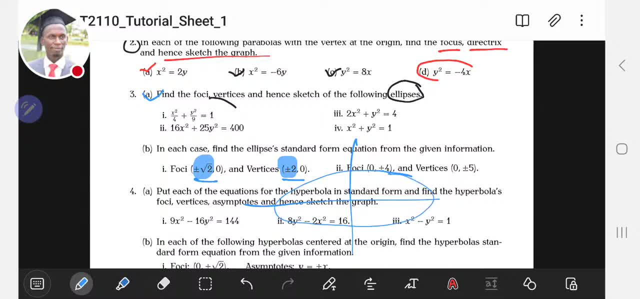 guaranteed that this one it's. it actually has a measure in the x-axis. but on the next one here, part two, when you look at it what you see is that it's a zero in the x and then it only has that value, the plus or minus four for the y value. and then when you look at the next one, here again it's. 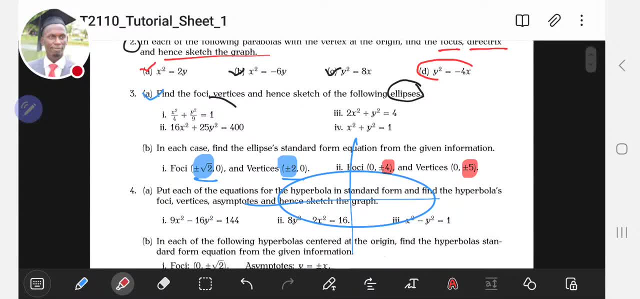 given as a y value here. so what this is going to do is it's going to give us an x-coordinate, and this is telling you is that this ellipse for part two, that ellipse actually has a measure in the y-axis, that this ellipse is going to look like this. so this is how you identify, just by: 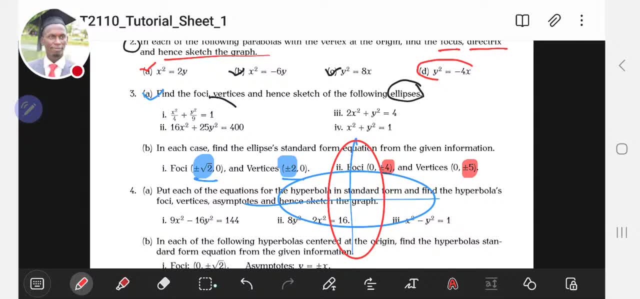 observing, observing those, okay, so you can use that trick, but we're going to just do one of them here. let's do part one. for part one, we have plus or minus root two comma zero, that is going to be, and then the vertices. what we have is plus or minus two comma zero. so how do we take advantage? 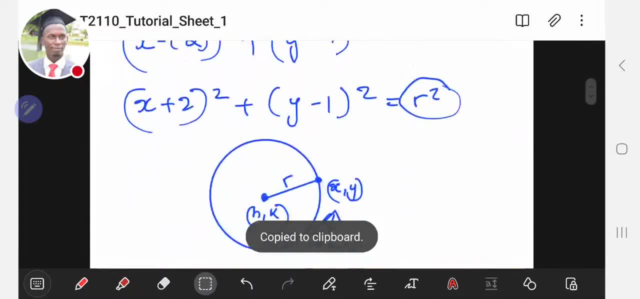 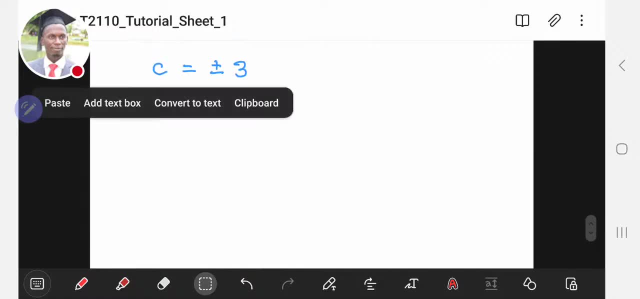 of of these to work out our question. well, let's see how it goes again. well, these are what we have. so we know to say: from the foci we always get the value of the value of c. from the vertices we always get the value of the value of a. so from here we see that. 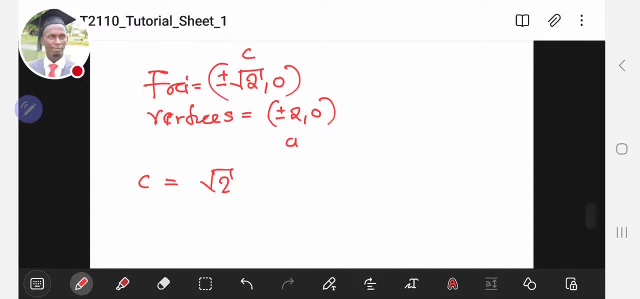 c was actually just root 2.. so if this is what c was, then c squared was actually just 2.. and then from the vertices we see that a here is actually being given as plus or minus 2.. so if you square this, we get a squared as 4.. having a squared and c squared, now we can go to the y-axis, which is: 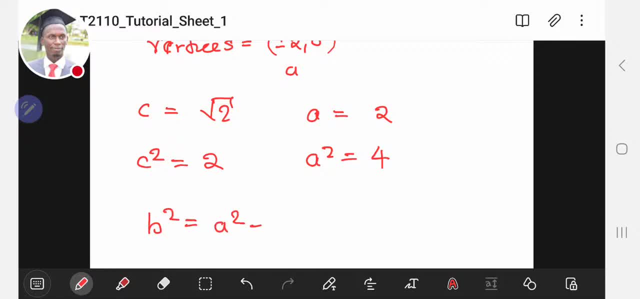 the matrix of the x-square matrix. so we have to find b squared and b squared, remember, is s squared minus c squared, so b squared will be equal to a. squared is 4c squared is 2, so we have minus 2. this becomes just a two here. so now we have a squared, that's 4. b squared: we have two, so we can now come. 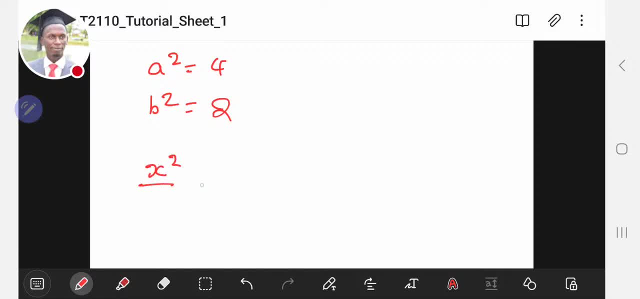 up with one with our equation. this is an ellipse. it's x squared over. so again, how does it open is it? does it open in the, in the y or in the x, or in the major? is it in the third third or in the fourth third? and so you know, that's what the 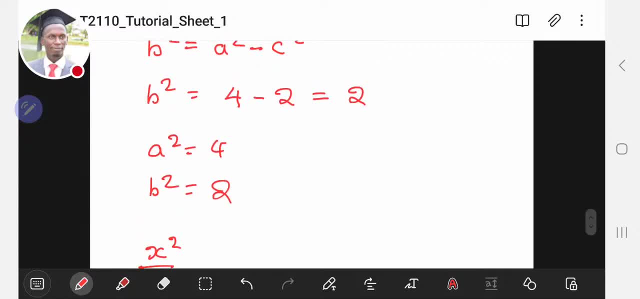 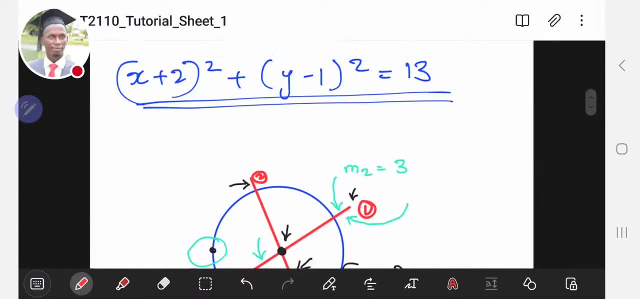 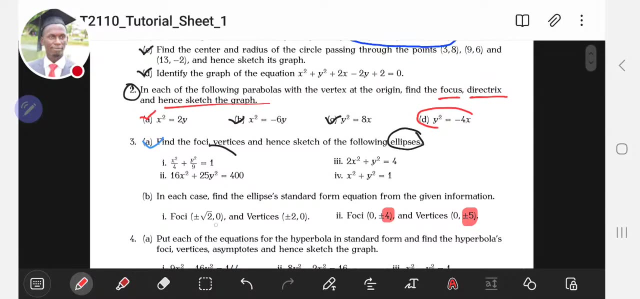 it major X or major Y in this case, remember, the prediction was major. the prediction was major was in the X, based on where the values for the foci was well, the zero was and where the other value was, so the major was in the X. yeah, for this one, the major was in the X. so because of that, we're going to come back. 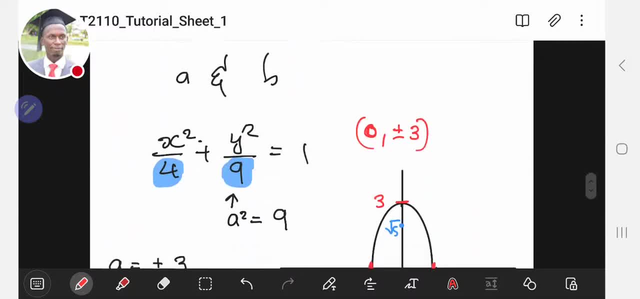 to this and say: since the major is in the X, then X has to be the one that has a, because if it's in the X, X must be bigger, as in the denominator for X has to be the bigger one. so this is where a squared is. then this is plus y squared. 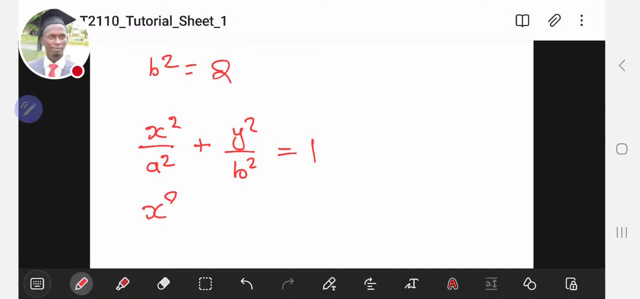 and this is where b squared is- is equals to 1. so this is x squared over x squared. what did we find? that was 4 plus y squared. y squared. this is over b squared, and we found 2. this is equals to 1. then we're done, we have found the equation. 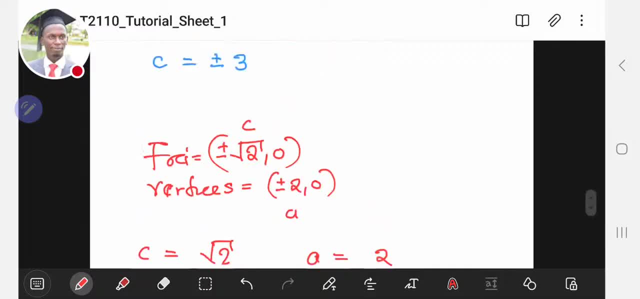 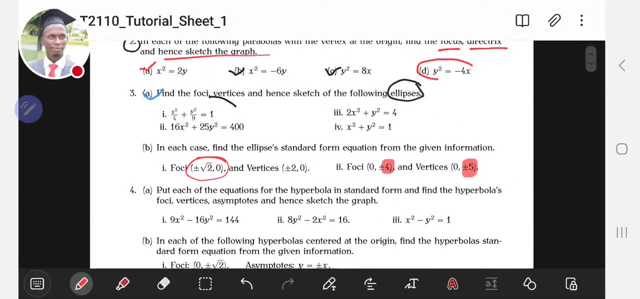 okay, of this ellipse. so we can use the same, the same technique to work out part 2 of the same question. so I can use the same technique to work out this question. the only difference now is that the major is now in the y-axis. so you still say C is. 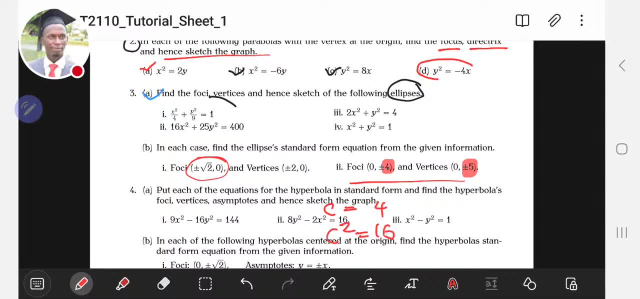 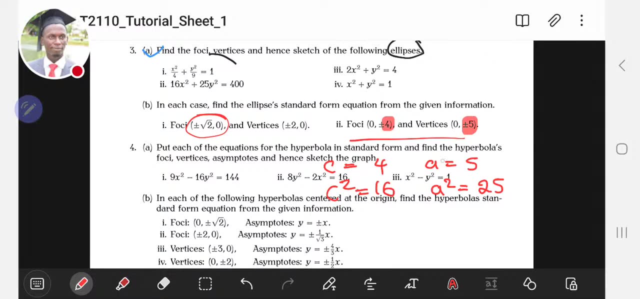 equal to 4, so that C squared is equals to 16, and you still say this is giving you a. you should say a is equals to 5, so that a squared is equals to 25. doing this will give you your, because you're going to have b squared equal to a squared 25 minus 16, so that this comes. 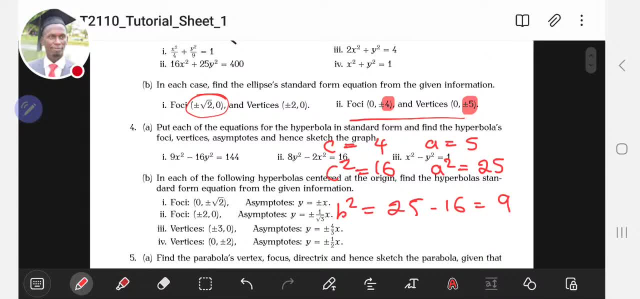 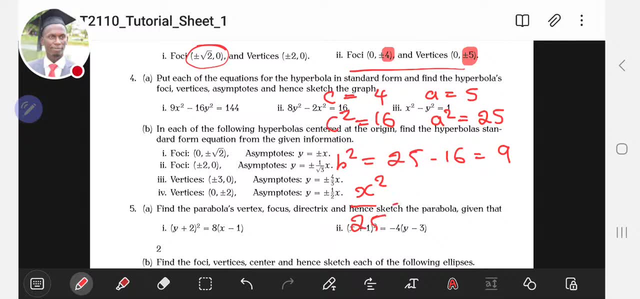 out as 9. now what you have to see is when writing your equation, you have x squared. don't get tempted and say here a is going to be here 25, and then say plus y squared over 25.. So this is going to be the denominator of y squared. so the denominator of y squared. 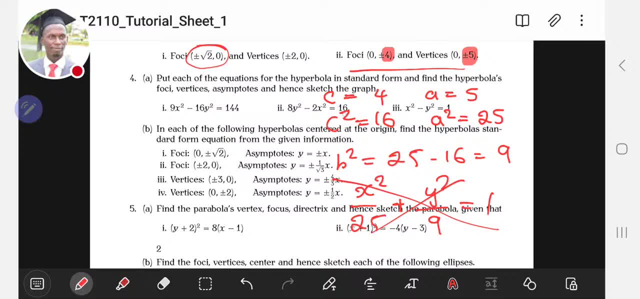 is this: one over 9 is equals to 1. this is wrong here. what I'm using is, I know to say the major is in the y-axis, based on the fact that these values are given to be y values: the value for the foci in the value for the vertices, with that in. 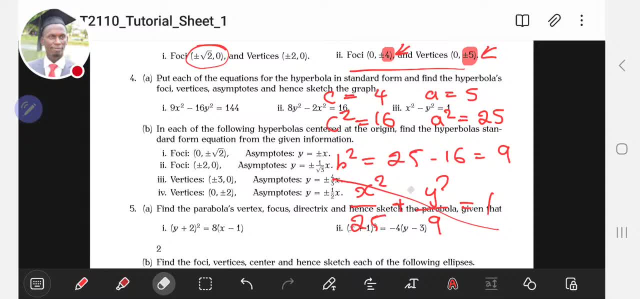 mind, I know to say the denominator of y has to be the bigger one, so the general why. why has to be the bigger one? in other words, why is the one that is moving with a? that is moving with a, so it has to be here 25.. 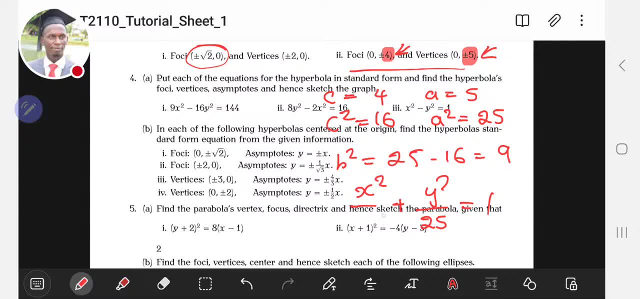 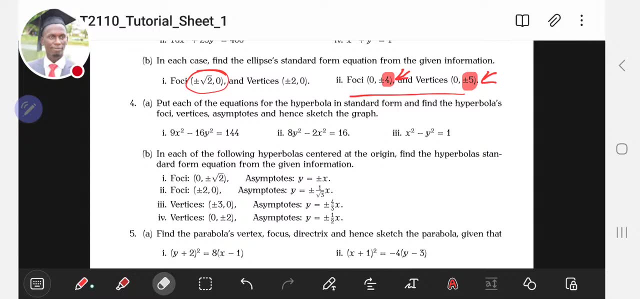 five and then x has to be the one moving with b. this is where the nine is. this is going to be the correct expression. okay, so that sorts out question uh, question three. we can now move on to question um. question four. question four: now they're talking about a hyperbola. 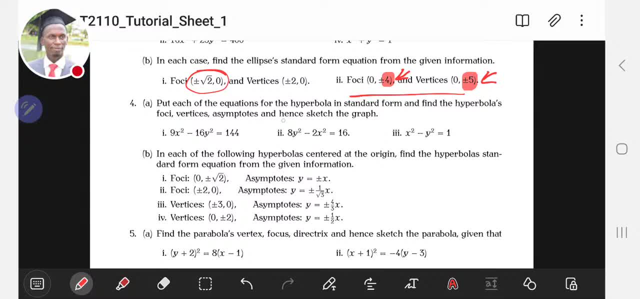 put each of the equations um for the hyperbola in standard form and find the hyperbola's foci, vertices, asymptotes, and hence sketch the graph. okay, now for this one, what they're saying. first, again, you have to understand what the standard formula for the hyperbola is. so for the hyperbola, 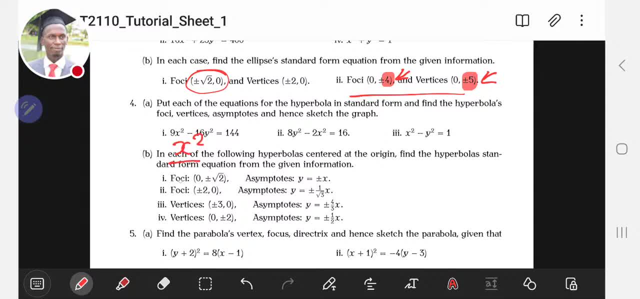 you know to say it has to be x squared over a squared minus y squared over b squared is equal to one. again, notice that it's similar to the ellipse. the difference is that now, on the middle you have a minus. another difference is that in this case you won't have b squared is. 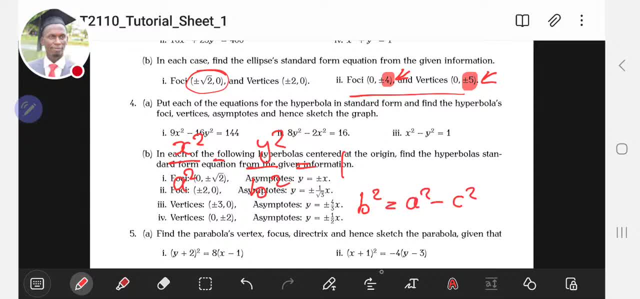 equal to a squared minus c squared. it's going to be a little bit different, the rather the sign here is going to change: instead of a squared minus c squared, this is now going to be c squared minus a squared or, if you want to remember it easily, for the hyperbola, the relationship. 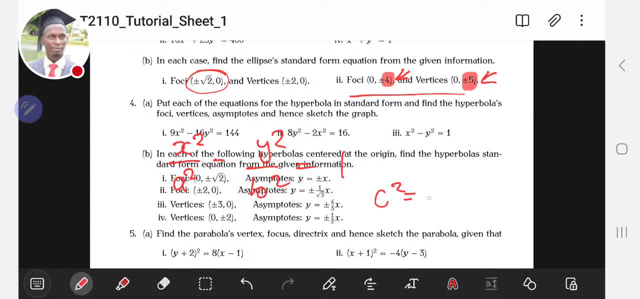 between the hyperbola, and the hyperbola is going to be c squared minus c squared. a, b and c is going to be such that c squared is equals to a squared plus b squared. You can see if this will be easier for you to remember, then you can stick to this one With this in mind. how? 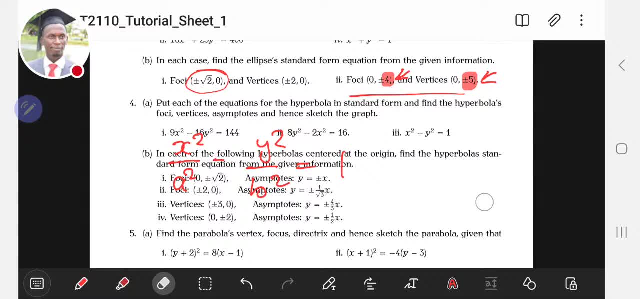 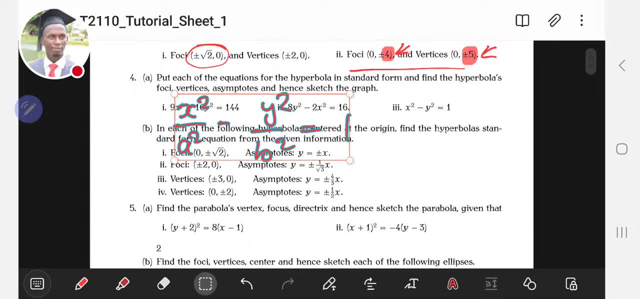 do you actually work out this expression? Well, generally, if you have a hyperbola that has this standard expression, then such a hyperbola actually opens in the x-axis. It opens like this and it opens like this one If, let's say, x was the one that was negative, if this term was the negative, 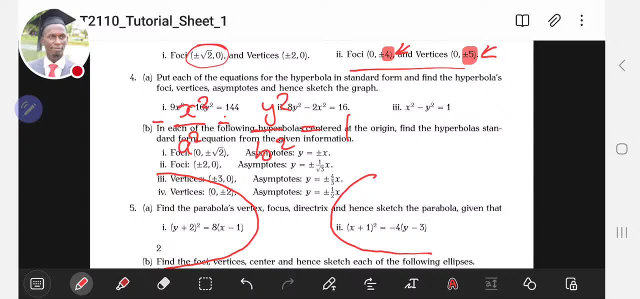 one, and this term was, of course, a few other things would change, but if, let's say, these were to change places such that now you had y squared being here and x squared being there, the minus being here, now what you're going to be able to do is you're going to be able to do this, You're. 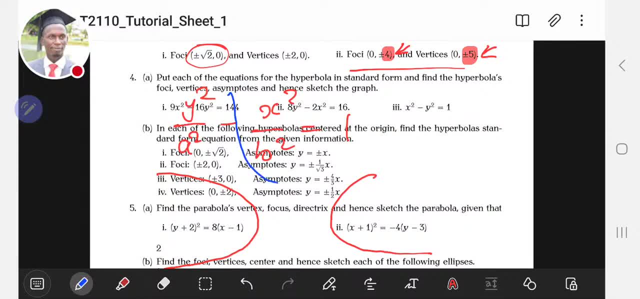 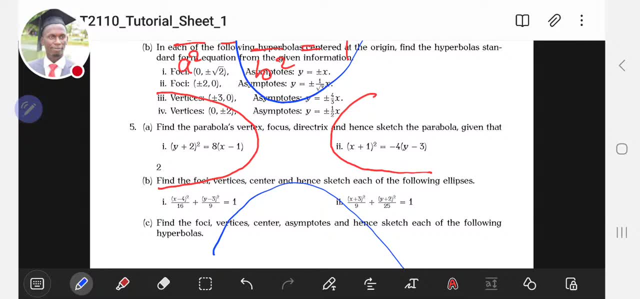 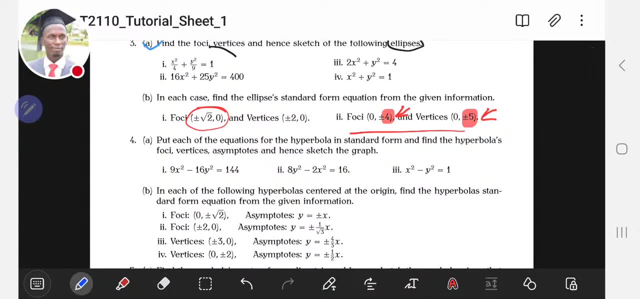 would see is that you still have this being a hyperbola, but now it would be opening something in this manner. so this is how it would be opening. so, of course, we're going to do examples to demonstrate each case. so let's start with the standard format. for the first one, what we have is: 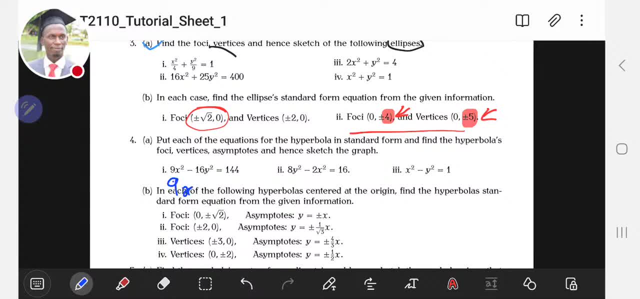 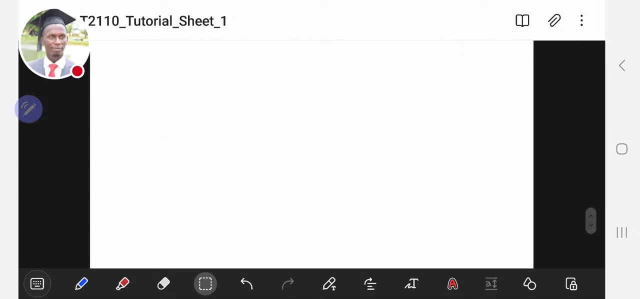 9x minus 16 y squared is equal to 144. so, just like before, you want to divide this by 144, so let's get this. let's go to the other side, okay? so you want to ensure that the right hand side is just a 1, so divide everything by 144. 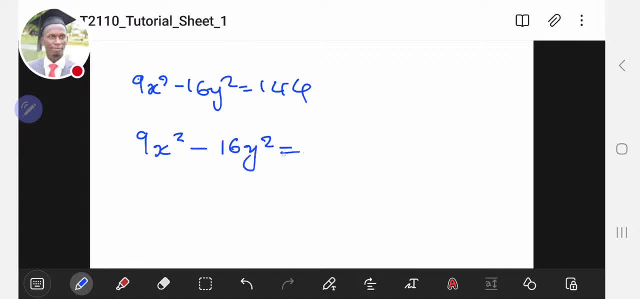 144. so you divide by 144, you're going to have 144 here, then you're going to have 144 here. the right side is just going to be 1. 9 goes 16, y squared is equal to 144. so, just like before, you want to demonstrate each case. so of course, 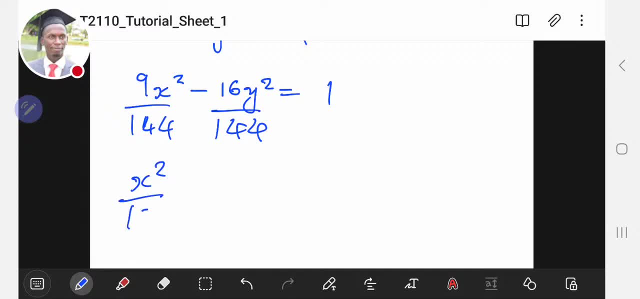 you want to ensure that the right side is just going to be 1: 9 goes 16 times into 144. this is going to be x squared over 16. minus 16 goes 9, 9 times into 144. this becomes y squared over uh over 9. 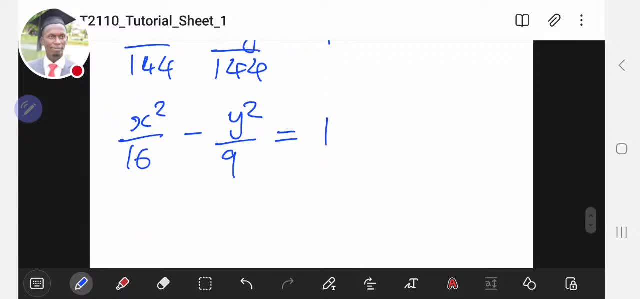 here, then this is equal to 1. once you've reached this part, you see that y is the one that is being negative here. um, once this is done, the position of a and b here will not change. the only thing here is that you're only identifying which one. if it's negative, of course you know to say it's. 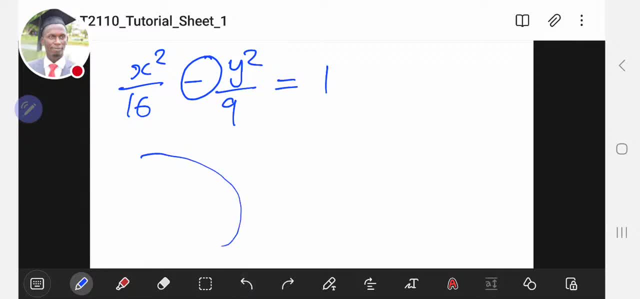 going to be opening. if y is the one that is negative, then you know to say: this behavior is going to be something like this and something like this, then you can easily get, uh, the, the position for the, the vertices, and so on. so let's, let's continue this, let's see how it goes. so, once, 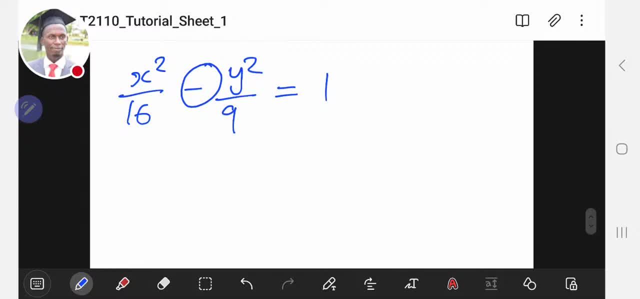 we've identified that. this is where the negative is. we know it's opening in the horizontal axis. so from here we can see that x a squared is equal to 16. once we have our a squared, we can easily get what our. our b, of course, is still equal to b. squared is equals to 9, and then you can easily get what our 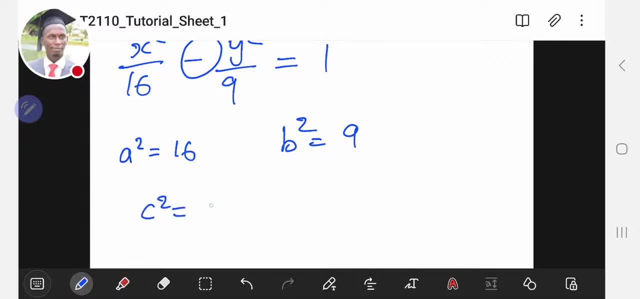 c is and our c- remember c squared- is equals to a squared plus b squared, so that this is just going to be 16 plus 9 and this is going to be 25. so our c squared is equals to 25. we can easily get what. 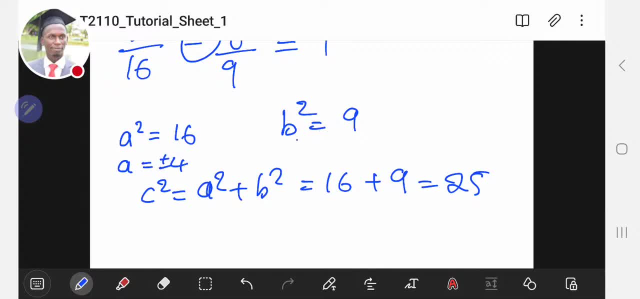 a is a is going to be 4, plus or minus 4. b is going to be plus or minus 3, so that c c is equal to plus or minus 5. once we've obtained what these terms are, we can now go back to our 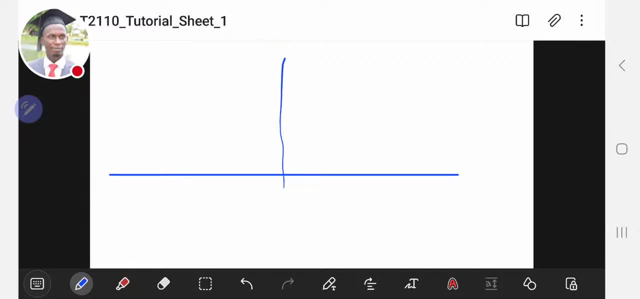 expression and try to plot it. so if we try to make a sketch there, we know to say it opens in the horizontal axis and to sketch it what you need now, you need a and b first. so get your. get your a, since you know it's opening in the horizontal axis. you know a is in the x-axis. 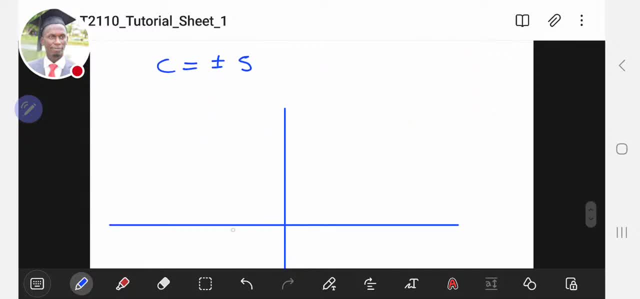 so a? you found that it is a 4, so you're going to go to negative 4. put your minus 4 here, put your positive 4 here. next your b. b here is plus or minus 3. so i'm going to go up here, put a 3, then go down, put a minus 3. after that you want to draw some form. 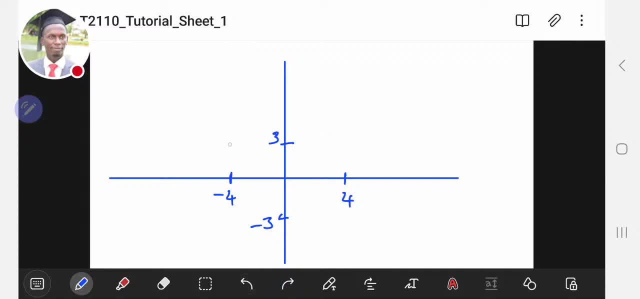 of a rectangle. here, of course, this has to pass through your point. okay, now that our rectangle is drawn, it has to pass through 4, of course here. uh, let me just play with it a little bit, i'll do this. it has to pass through 4, so let me just remove this one. so we're going to do. 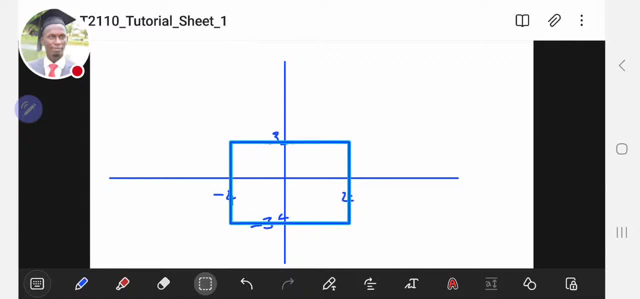 okay, it has to pass through 4, it has to pass through 3, and so on. okay, approximately that. no, not too good. okay, something like this: once you've done this, you're going to draw your, your asymptotes. your asymptotes will be running from diagonal to diagonal, so it's going to be a line passing through the origin, from diagonal to. 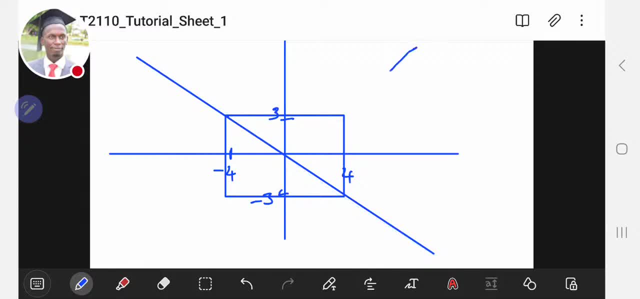 diagonal, so something like that. and then the other asymptote is going to be again from this diagonal to that diagonal, something like that. i can just shift this, can i? okay? not too good, so let's do this. so I'm going to do this, okay, better. so these are going to be our asymptotes, this one and this one. 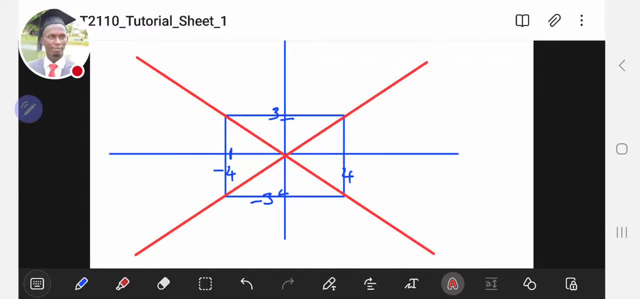 we need their equations. we're going to find the equations as well. so to sketch the graph, you want it to pass at the at the vertices. this was at four and our four has to be literally here, right here. our negative four and our positive four will be here, so this is going to be a parabola. 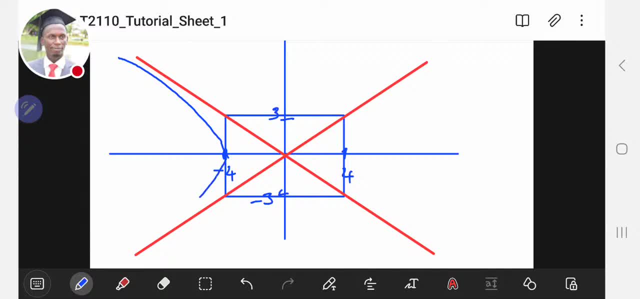 hyperbola. it will pass like this: uh, touch our, our vertex, vertex there, and then come down like this. and then the other one is going to come like this: touch here and then turn down, never touching those, um, those red lines. so once we've done that, 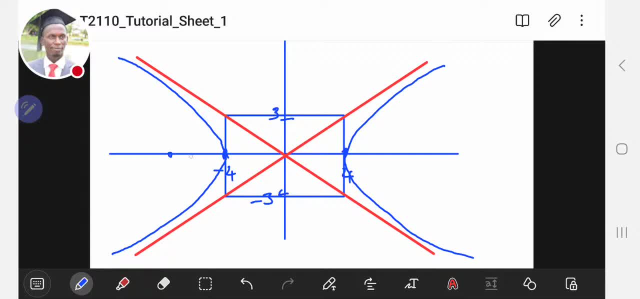 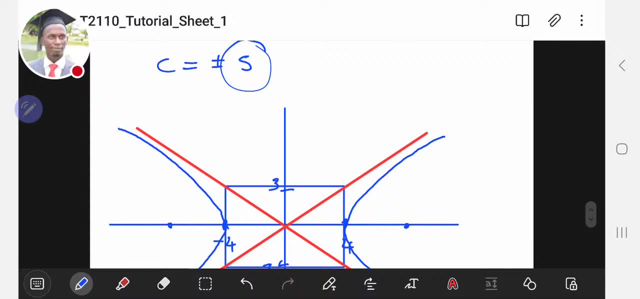 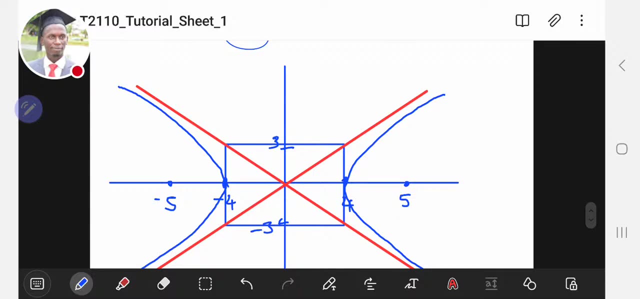 the focus is going to be somewhere. here we can approximate it, and the other one is going to be somewhere. here we already have the value. the focus is given by c. it's plus or minus, so this has to be minus five. this has to be plus five. then the only thing that is left is 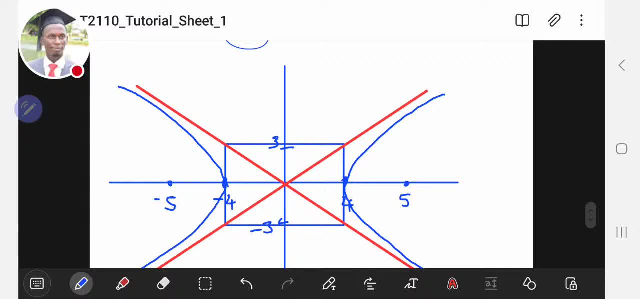 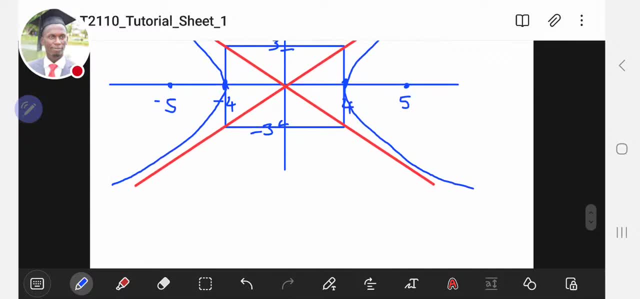 for us to state the equations of the um, of these asymptotes. now, how do we get, how do we get the, the asymptotes? well, there's a formula. if it's opening in the horizontal axis, then the asymptote is going to be given by: y is equal to b over a x. if it opens in the y axis, then the asymptote 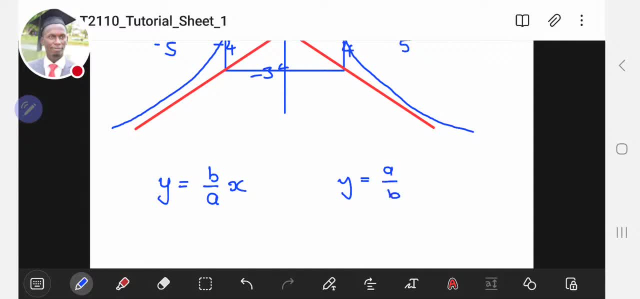 will be given by, y is equal to a over b, x. you can use this, but if you forget, maybe you swap them. you know whether it's a over b or b over a. just go back to the expression. in this case, the expression is this one here. uh, the simplified one, this one. you want to get the equations of their asymptotes. 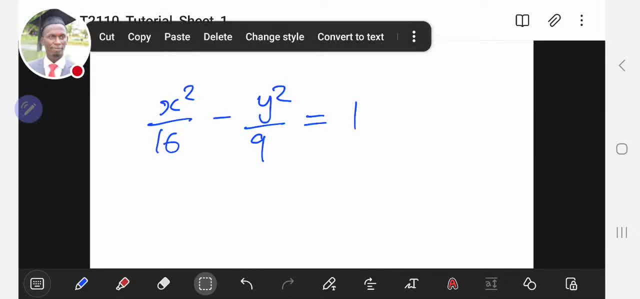 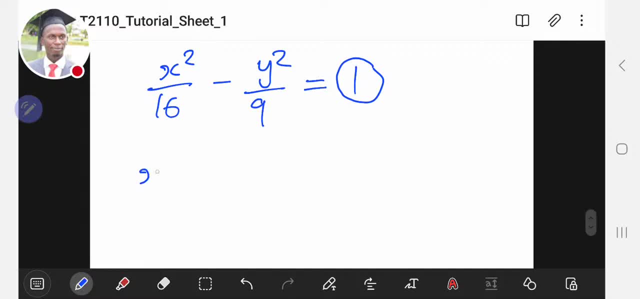 so what you do is, let's say, i don't know, i've forgotten whether it's a over b or b over a. the only thing that you have to do here is just make the right hand side a zero and then solve what remains: x squared over 16, minus y squared over 9 equals. 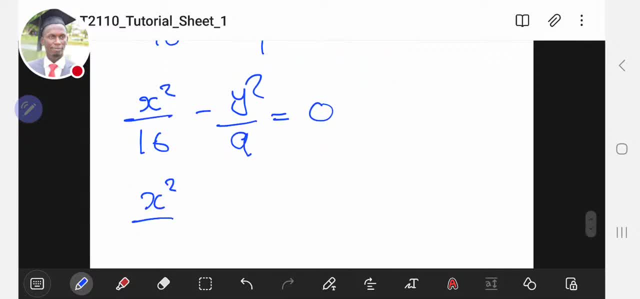 equal to negative sum x, and that will leave you with negative infinity until x to theист 0. express this: this becomes x squared over 16 equal to y squared over 9 becomes positive. and then make y subject. here it's going to be: y squared is equals to 9 over 16. 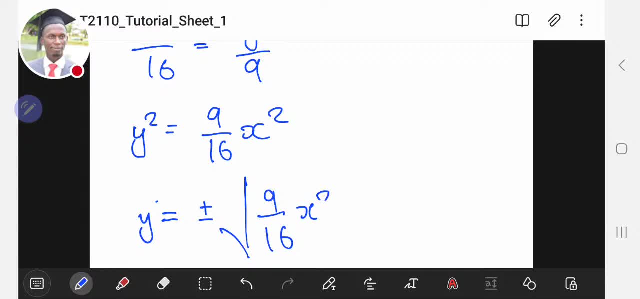 x squared square root both sides, this becomes y is equal to plus or minus the square root of Bible 9 over 16. x squared Minus, that's a 3,. over the square root of 16,, that's a 4.. The square root of x squared, that's just an x. 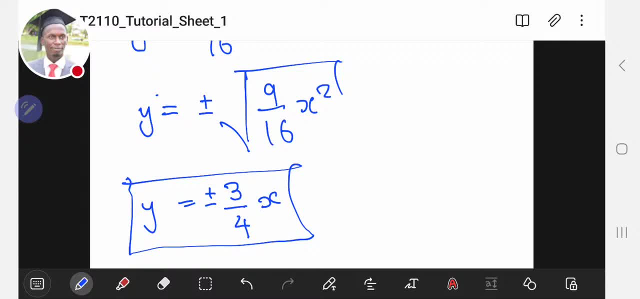 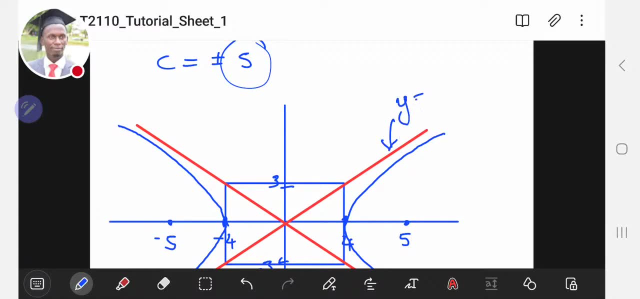 So this is the expression that actually gives us the asymptotes. So the positive one gives us the one that has a positive gradient, which is this one. So this is going to be: y is equal to 3 over 4x. The one slanting down will be the one with the negative gradient. 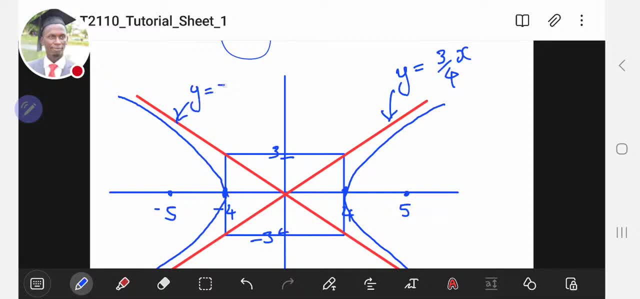 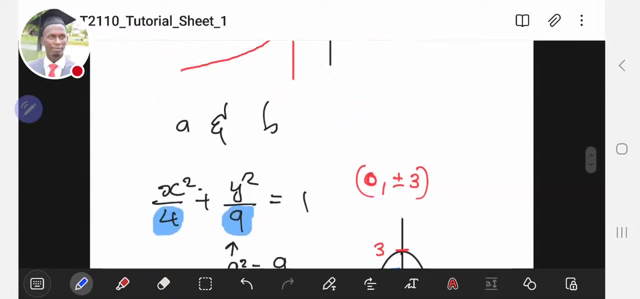 This is going to be. y is equal to negative 3 over 4x. So we've got the asymptotes now, So we're done with this one, Okay. so, yeah, we can do the next one, But the next one it's pretty much the same thing that you're trying to do there. 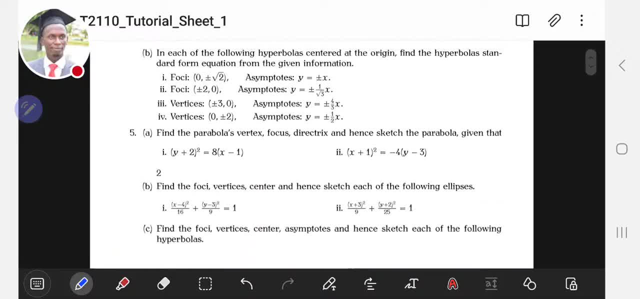 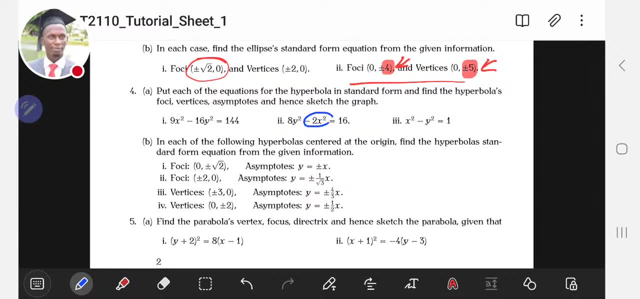 But the only difference now is because x squared is the one that is negative. you know to say, this one is going to be opening in the vertical axis. So, because I'm seeing x squared is the one that is negative, this is going to be opening in the vertical axis. 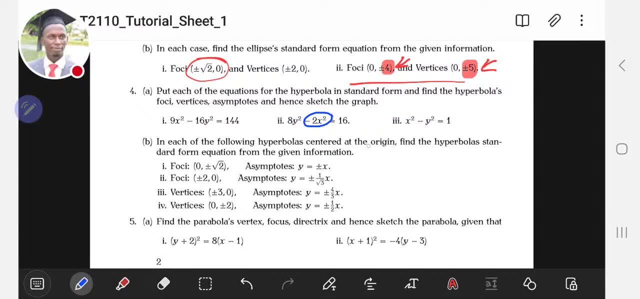 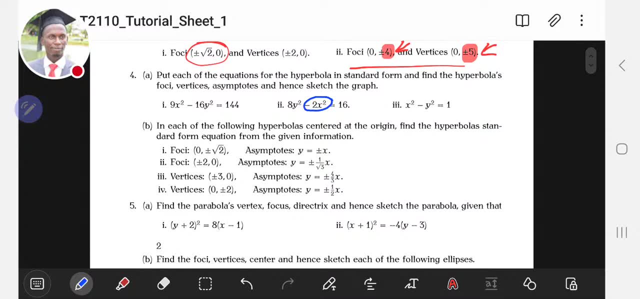 So that's going to be the only difference here. Yeah, so that is going to be the only difference with this expression. Okay, so yeah, I'm thinking we end here. I think I have to go for another program If you guys have more questions that you might want me to help you with. 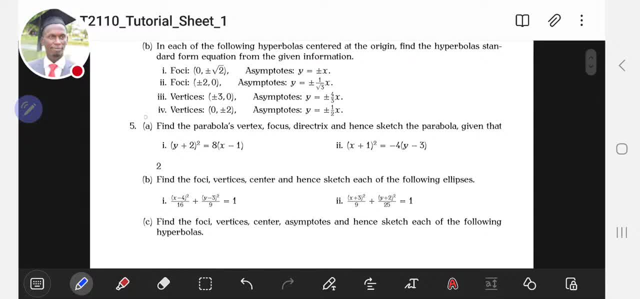 you can still get in touch. I really wanted to also do question five with you guys. It's something that is very, very interesting, But I guess we can do this some other time. Yeah, I think we'll have to end here. 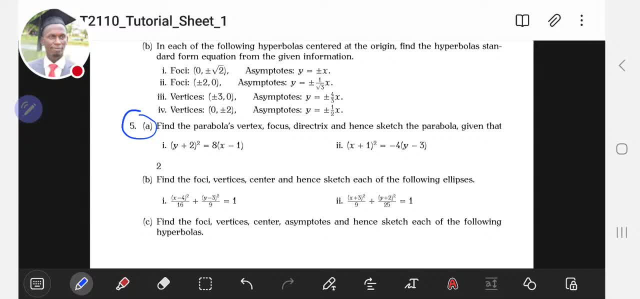 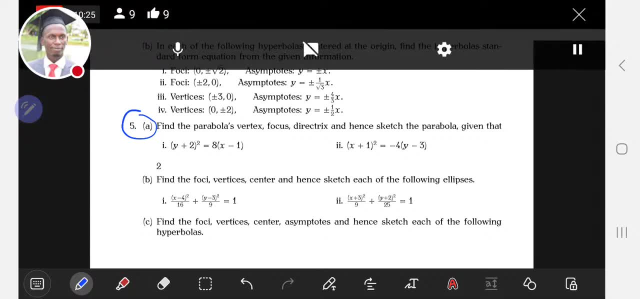 All right, so Yeah, all the best to you guys as you prepare for your assessment. All the best, Bye.